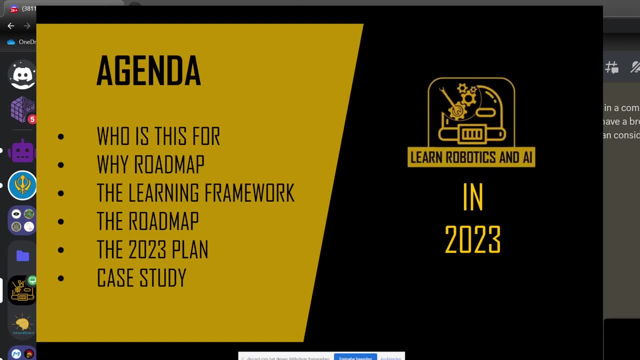 courses for that. and also you can plan. you can create a weekly, monthly plan for the next year, and then I'll be taking a case study that deals with using this roadmap and how a hypothetical person who wants to start learning robotics and become a software engineer in that domain would use this roadmap and actually start. 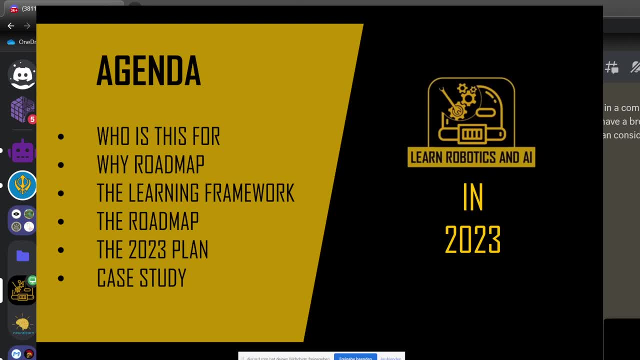 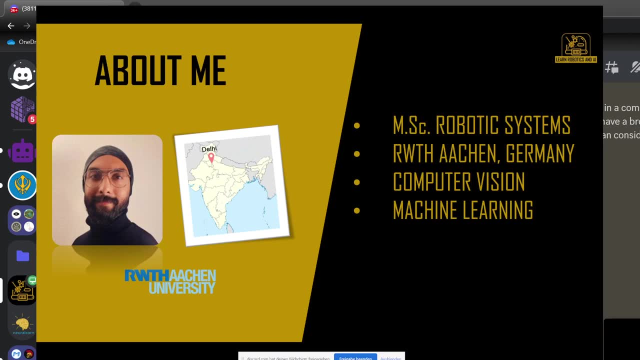 Start working Eventually using this system. So a little bit about me. So my name is Chandan deep Singh. I did my masters in robotic systems from RWTH Aachen in Germany and after that I've worked for a bit in computer vision and now I'm working as a robotics. 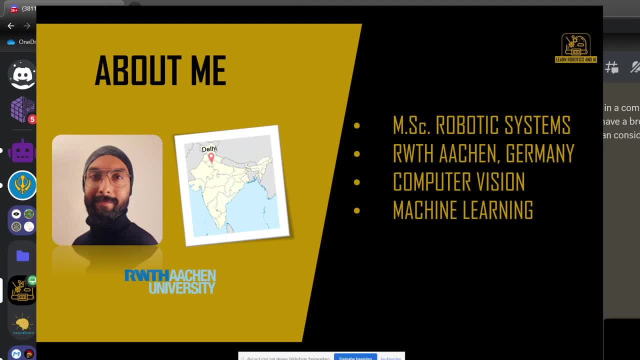 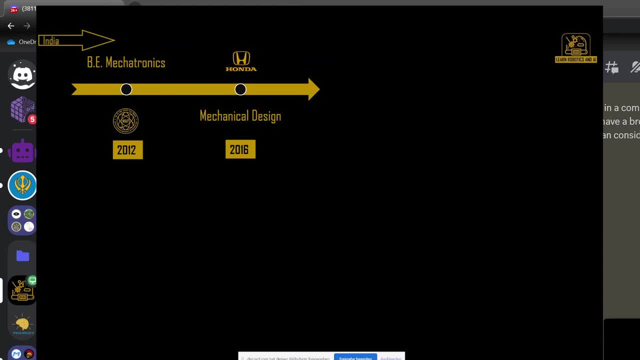 researcher. so my areas of interest are robotic manipulation, machine learning and computer vision, and And So the reason I'm sharing this is so that you can get a sense of Where I'm coming from. So the My background was that I did my bachelor's in manufacturing process and automation engineering from NSIT. 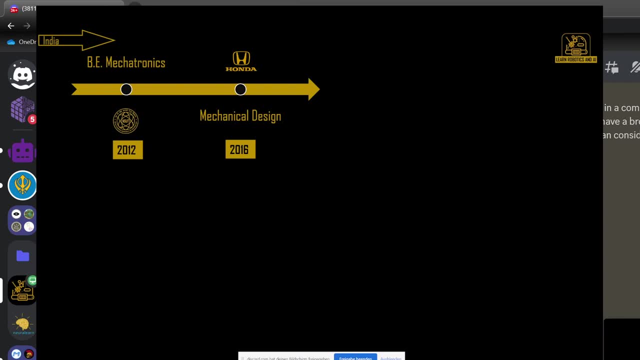 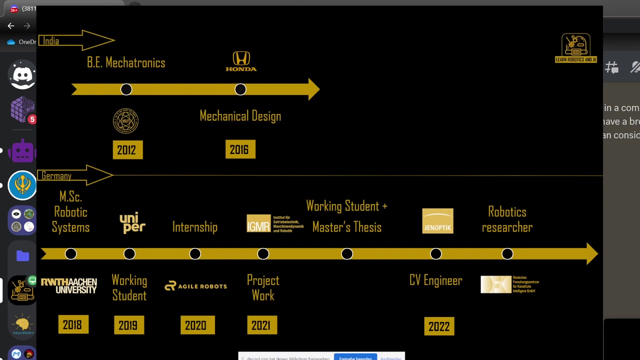 And then after that I worked as a mechanical design engineer. So in in India, when I was there, my profile was primarily mechanical engineering. I was working with Katia and mostly in the design domain, and Then after that I wanted to switch to robotics and then I did my master's in robotic systems from Aachen. 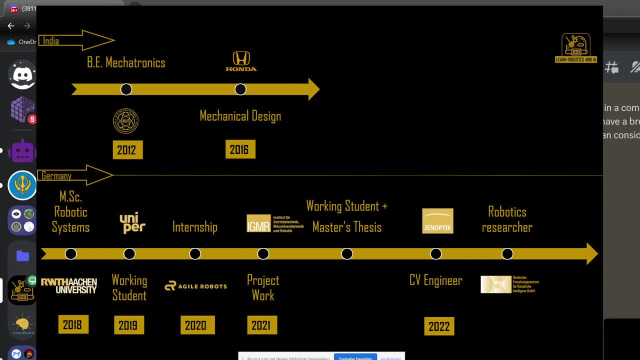 And while pursuing my master's I got the opportunity to work in some Industries, some positions as working student and internships, and also For my master's thesis. So there I got a lot of exposure to different kinds of projects that are going on. So first, 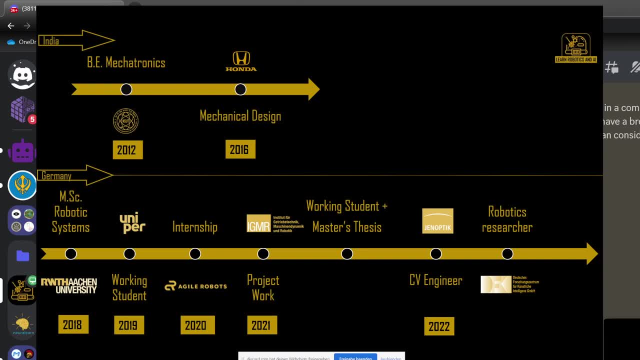 My first project was with drones At one of the companies where I worked as a working student and then I did my internship at one of the other robotics companies and then I did some additional project work where I got exposure to task planning. so a different Domain of AI. it has to do with scheduling and planning. 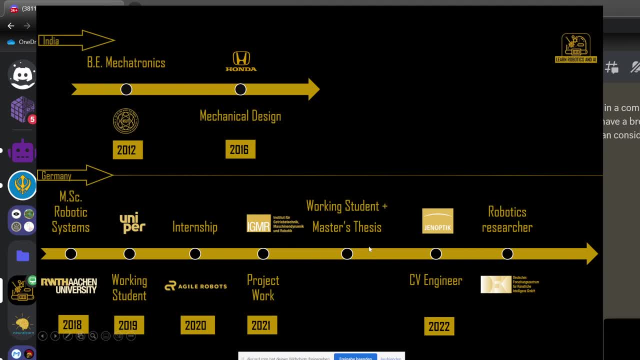 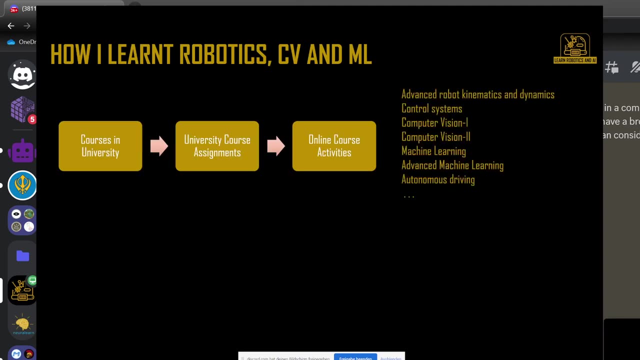 in an automated way. and then I did my master's thesis at Another company and then I worked for a computer vision engineer and now currently I am a robotic researcher. So how I learned a robotic CV and ML? of course, for me it was a bit systematic, since I was in a 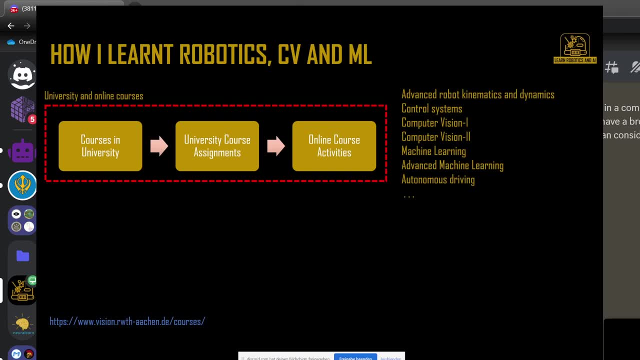 Systematic university program for my master's. I did took up courses in the university and I did assignments which gave me exposure to using the tools, And then I also took some additional courses to fill in some gaps. So primarily, this course was very interdisciplinary and I took up subjects ranging from control systems to robotic. 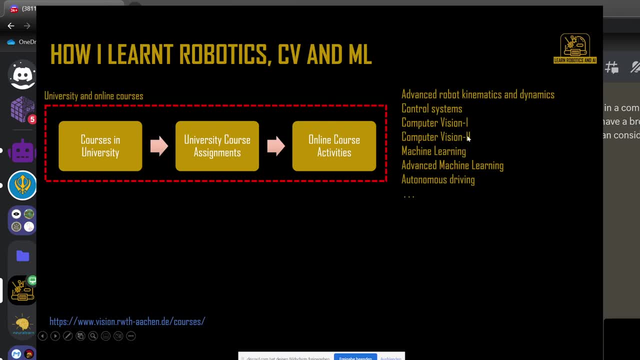 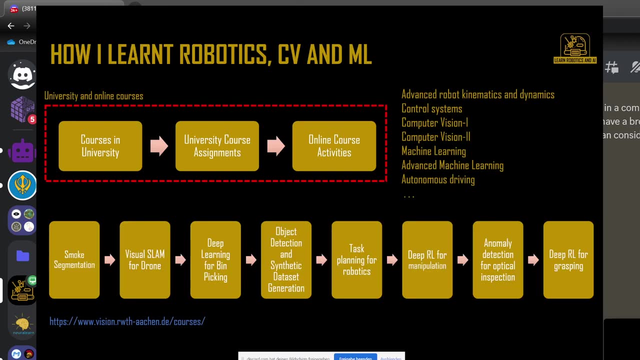 kinematics and dynamics, computer vision, machine learning and Eventually I focus more on machine learning and computer vision. But this was just one part of the picture. So the major learning for me was when I Got the exposure to work in industries and as working student, internships and also full-time positions. 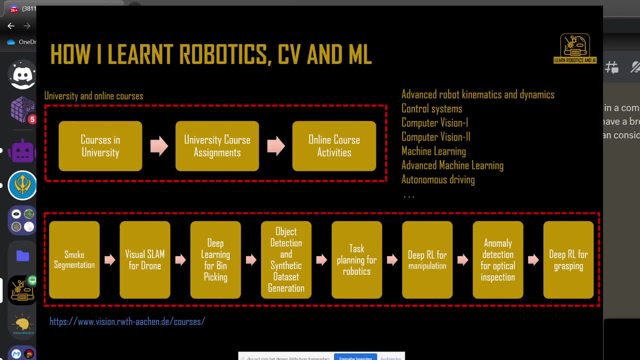 So I've worked on these projects, without going into too many details and just: I worked on one smoke segmentation project, and then I worked with drones and creating a mapping of the environment, And then I would use deep learning for bin picking for one of the other startups. 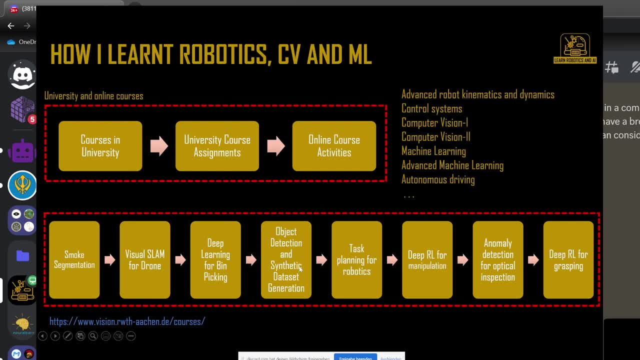 And then I used object detection and synthetic data set generation for deformable objects, And then for the project work that I mentioned, I used task planning for robotics, And then for my thesis I did deep reinforcement learning for manipulation and then computer vision. 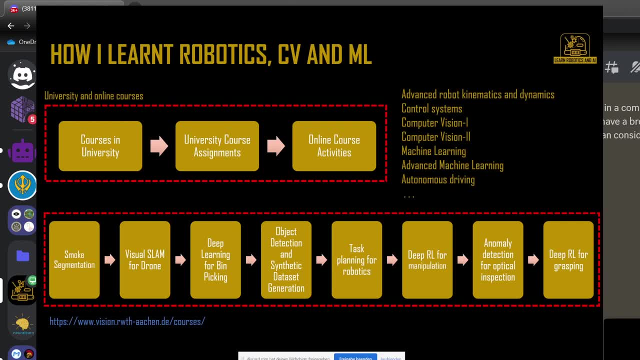 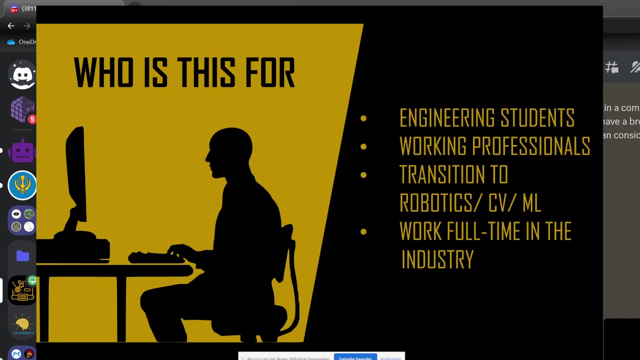 conventional computer vision and also machine learning for optical inspection, And currently I'm working in deep reinforcement learning for grasping and other applications, which is similar to my master's thesis. So this was my industrial experience. So the reason why I shared my industrial experience, 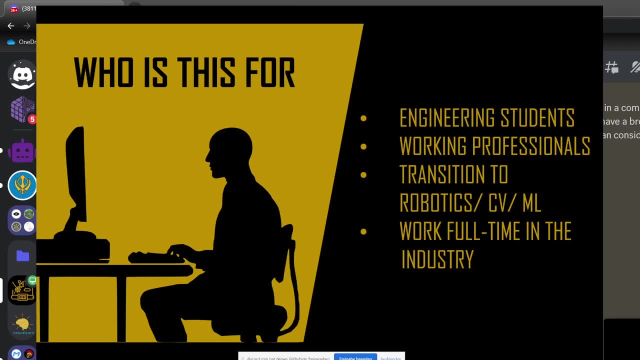 So that you know my background and I'm basically making this roadmap based on my own experience And, as you saw, that I have experience in diverse set of domains, in robotics or different areas of that, And that is why I understand the broader picture. 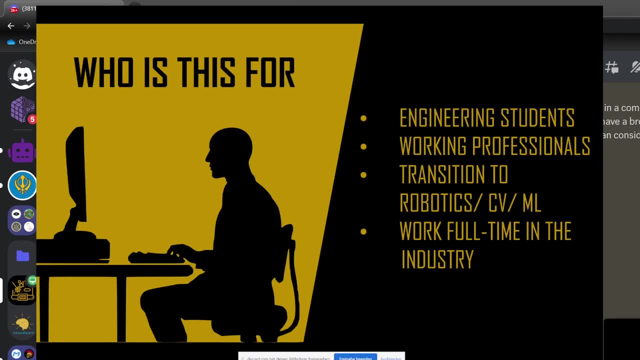 And I also know that one needs to have a specialization, And no way, nowhere, have I seen such a system that allows one to explore several domains in a single day, In a project based fashion, And also such that you identify things, identify your own specific interest, and then you gain mastery in that. 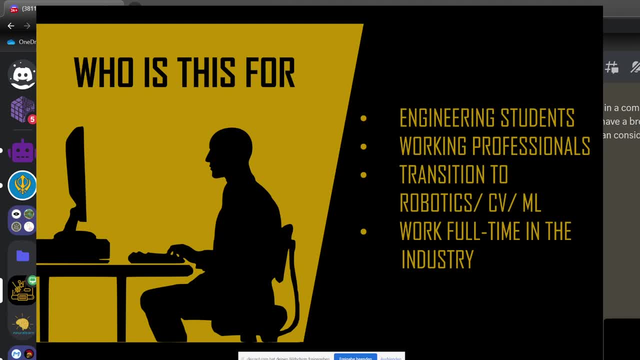 So this is what I'll be focusing on, And I'm focusing on engineering students, students who have some background in engineering- whether you are doing your bachelor's in engineering domain like mechanical electronics, computer science and so on- and working professionals who are also engineers but who want to do engineering. 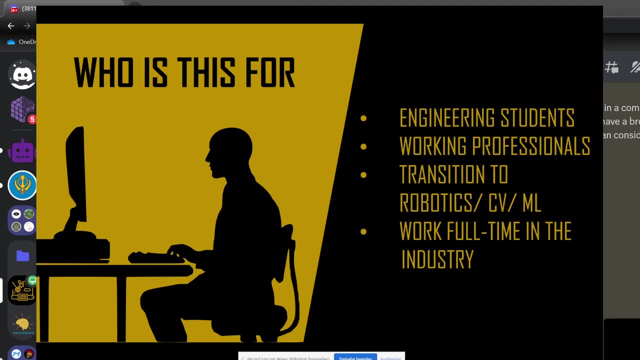 But who all want to become engineers, to transition to robotics, uh, cv or ml. so these are the three domains i'd be targeting and you could learn robotics and build projects as hobbies, like we do. we see the arduino projects and the robotics kits and so on, but this is not what i'll be focusing on today. i'll be focusing on 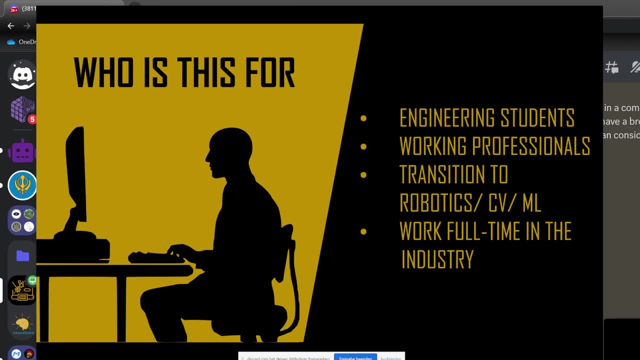 which are the specific skill sets that you would need if you actually want to work full time in the industry. so i'll be focusing on the very specific things that you should be focusing on and, of course, you could use this framework to also build some side projects, but primarily the idea. 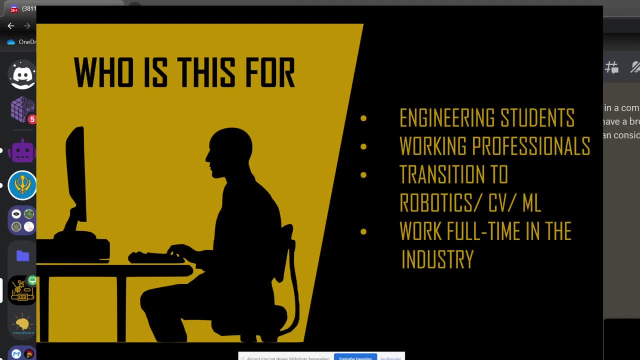 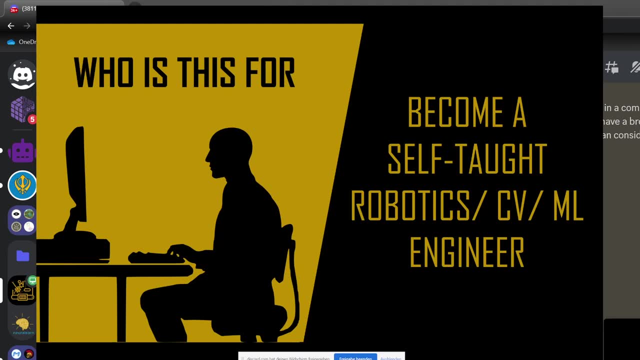 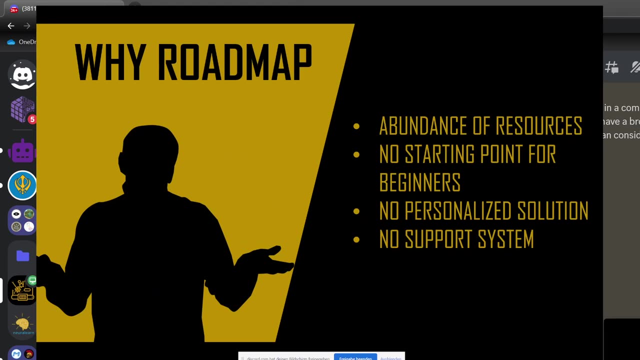 would be that you want to be employable based on these skills. so the idea would be: the target audience would be people who want to become self-taught robotics, cv or ml engineers. and why do we need a roadmap? i think we have an answer to this already. 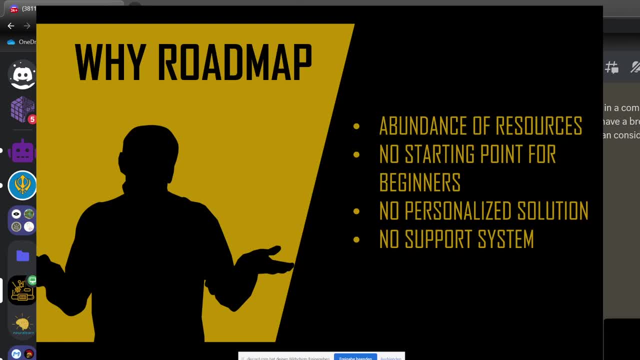 i talk about this in our previous meetups and also in our in the videos that i've been making recently. so there's a huge amount of resources that we have all online, which is a good thing, but it is probably confusing, and i was there when i was already working as an engineer in india and 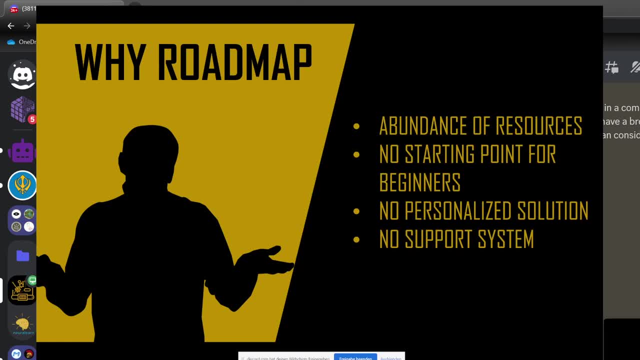 i wanted to start learning robotics on my own. i didn't know where to start and i was just trying out different things, but there was no clear direction, so this is something that i can help beginners with right now, which is what i'm trying to do. there's no personalized solution, and i think 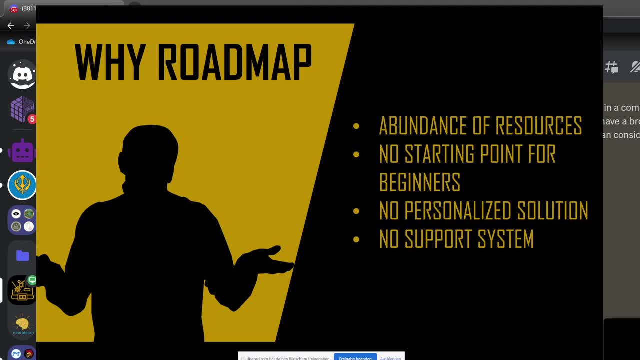 this is a universal problem. even the best universities won't take into account a personalized system, a personalized curriculum, and eventually everyone has to find their own direction, but the system that i will be sharing today. it will hopefully help you identify your own niche in a very systematic way, without causing a lot of. 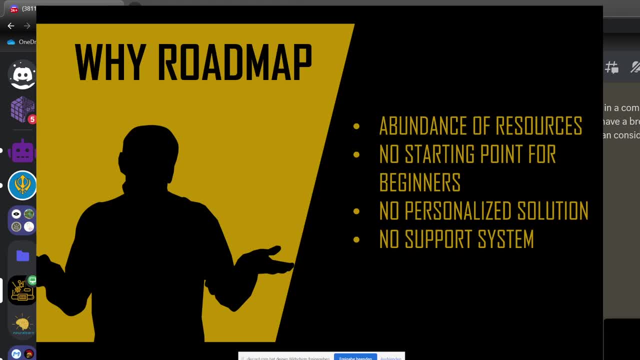 confusion and without trying out random projects and ideas. and another thing would be: there is no support system. if you are, if you want to be a self-taught engineer, you want to. you want the support of people when you get stuck while debugging for a project that you start on your. 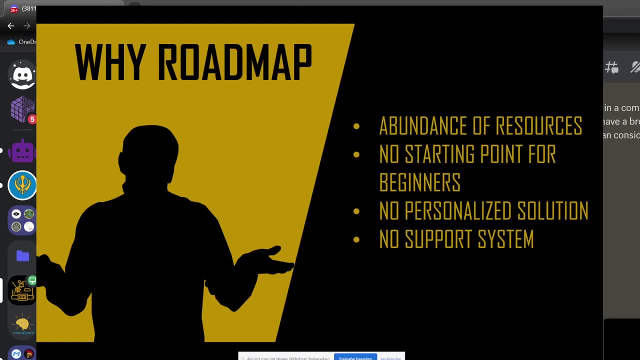 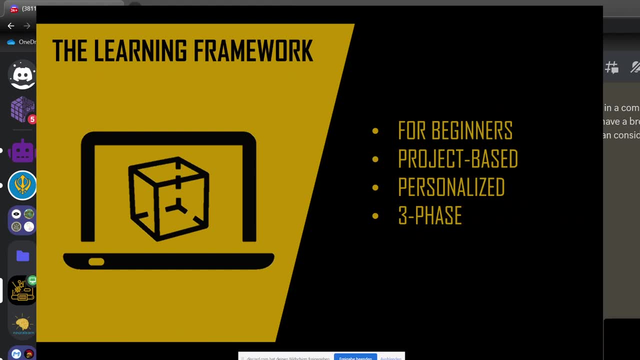 own. so all of these are the reasons why we actually need a system or a roadmap, and first i'll talk about the learning framework which i have expanded over time, as i mentioned, and i'm excited to share this today. i'm also looking for your feedback and i i think at the end of this session we can discuss, we can talk. 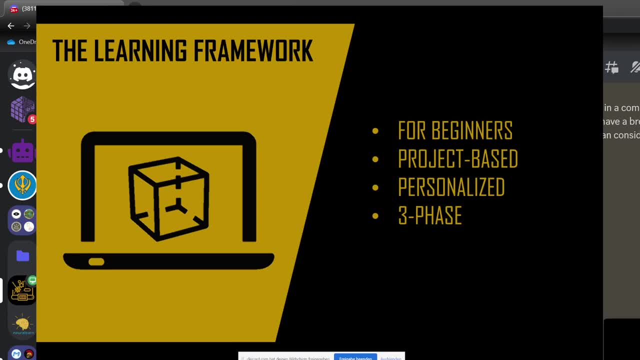 about your views and if you have any suggestions for improvements. so the the learning framework is absolutely for beginners. so anyone with any with no no knowledge about any of the fields of robotics or ai can just start using this framework. it would be personalized it and it would. 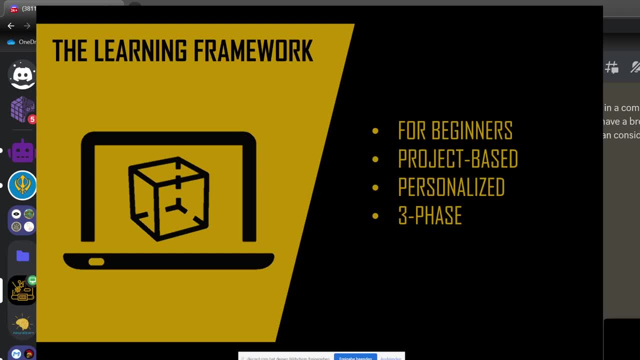 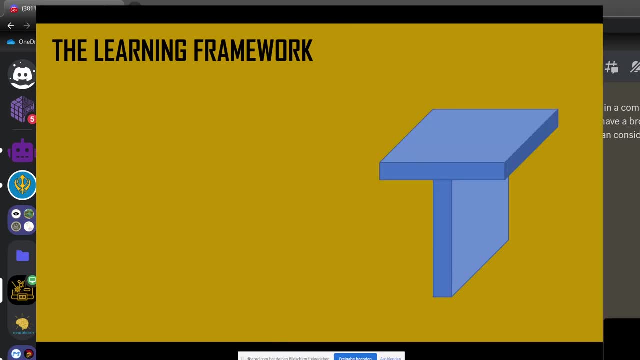 consist of different phases, because i think learning must be done in different phases based on the goals that you set for yourself. so this is, uh, this is a the t framework that we talk about so generally when we talk about robotics or actually any field, any engineering field or any field in general- that you want to learn and gain mastery in, you want to have a 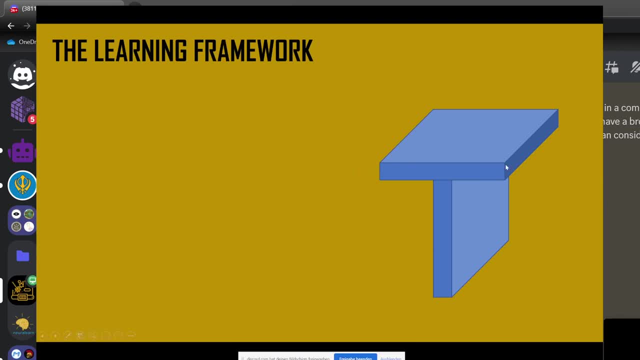 broad understanding of different domains in that field, but you also want to gain deep expertise in one area. so this is what is at the core of this framework. so the top portion that you see is exploring and having a broad understanding of different domains, and this bottom portion is 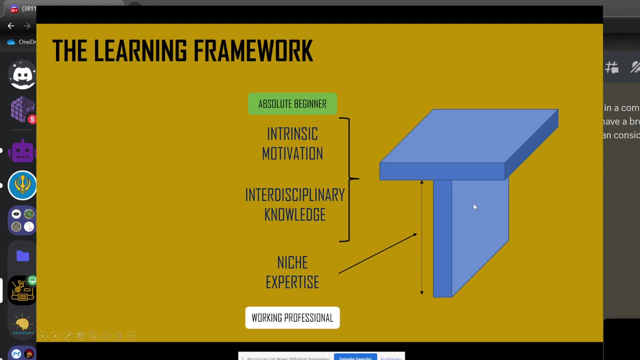 basically deep expertise that you would have in your niche, and the way that you get to understand different domains is, first of all, as an absolute beginner. you should be driven by your intrinsic motivation and intrinsic curiosity. what are the things that you find really interesting? what kind of projects interest you? 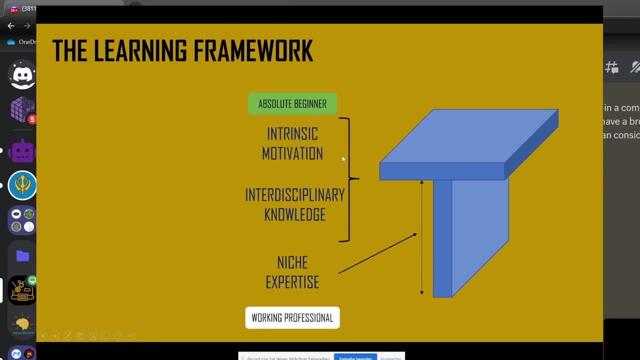 and focusing on those things and then also focusing on different kinds of subdomains which you might not be interested in, but you would still want to explore, to get a foundational understanding. so this is exploration stage and this is the mastery stage where you would be focusing specifically on your niche. once you have identified your niche, you would be focusing 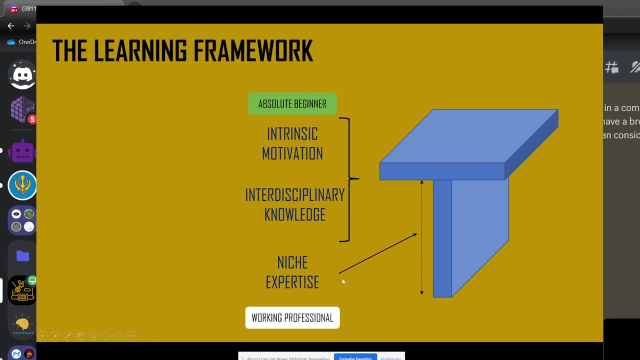 specifically on that and then, only then, would you be capable of working in as a professional in the industry. so, as i mentioned, there are three phases of learning. so the first one is curiosity driven exploration. so there will be activities that i would share throughout this presentation that 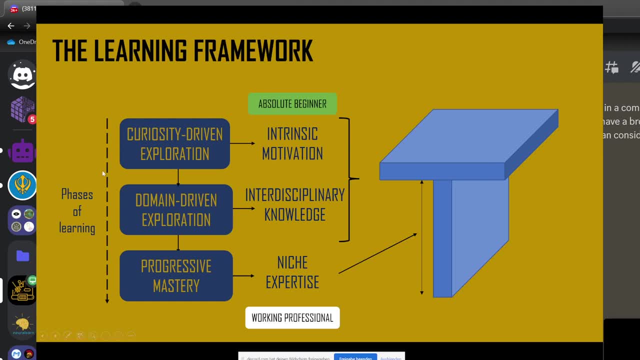 would allow you to explore your interests and focus on what you are interested in and what you find interesting. and then i'll be talking about domain driven exploration, which would be featuring different domains based on your interest. that would allow you to explore the different areas that are in robotics and also artificial intelligence, and after that you should. 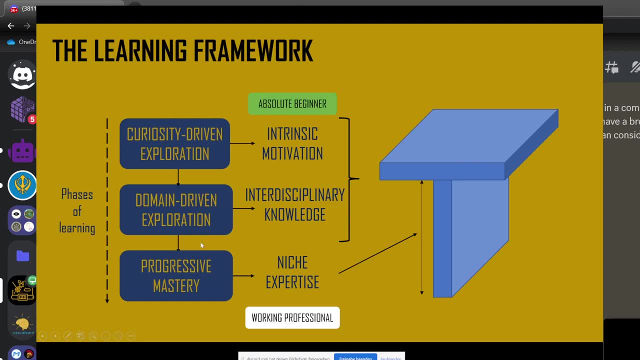 have a niche. basically, we'll have activities where you can define your niche and then you'd be able to get mastery in a progressively increasing manner, which means that you'd be taking up projects of progressively increasing difficulty. and all of these phases are project based, so the entire framework is project based at the core. 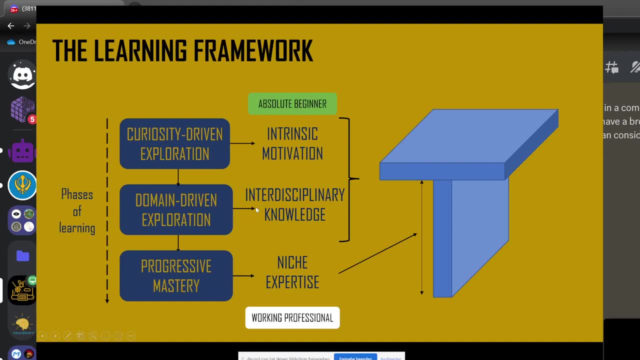 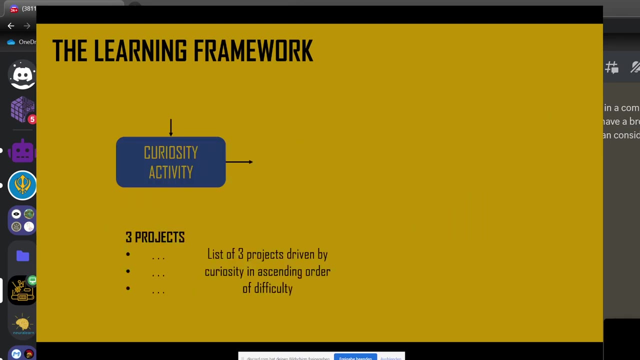 and it's totally different from the conventional way of learning, where we have lectures or theoretical discussions and then projects. so this is the main idea behind it. so let's talk about curiosity based learning. so before i do that, let's pause a bit and if you have any questions- because 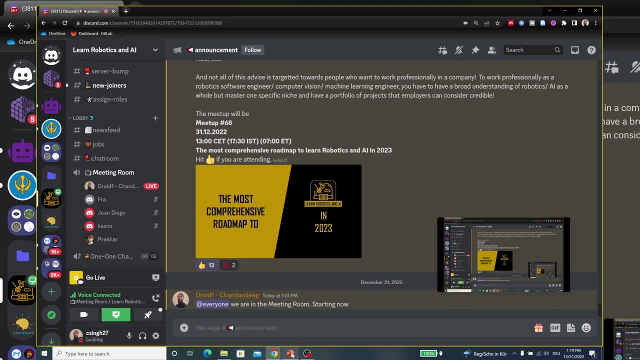 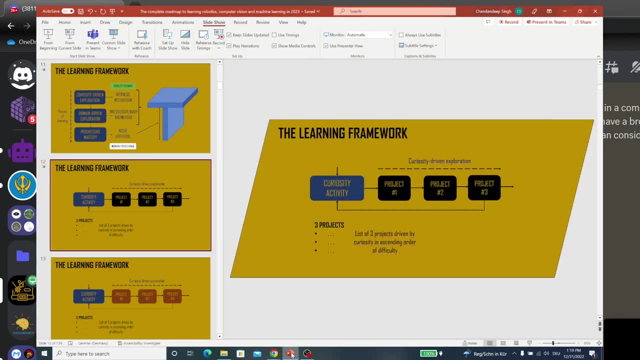 this is going to be a long session, so it would probably take one hour, one and a half hour or something. so if you have any questions, just feel free to stop me also in the beginning. so so far does it make sense. i haven't covered anything in much detail yet. 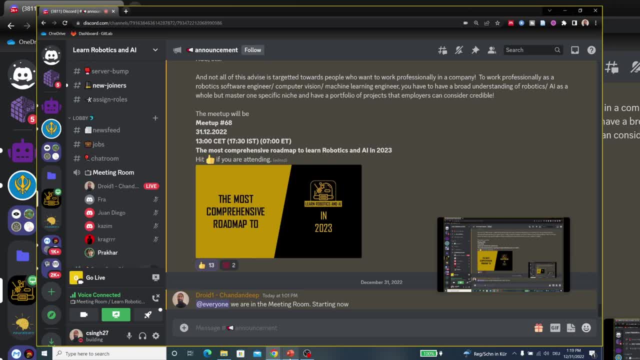 okay, hey, i'm audible. hi, yeah, you're audible. hey, so i'm a student in india. i'm currently in 11th standard. okay, i'm currently learning web development. okay, because i'm interested in that field and i want to start my tech career in that field only. 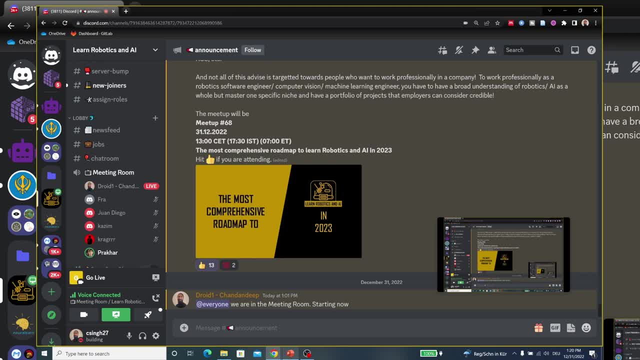 but i'm very much interested in robotics and artificial intelligence too, so i wanted to know that, like, um, i don't want to go seriously into the industry of robotics, but rather make my own, um, good, like side projects and with web development, okay, and yeah, yeah, so, uh, so, basically, your, your question. 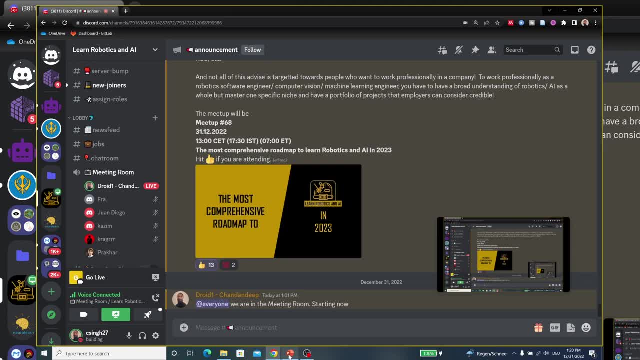 is specifically, uh, related to, um, whether you want. so you want to explore robotics and do some side projects and so on. so i think the the framework that i will be sharing would allow you to also take up different projects just for your interest and explore and see if this is for you or if you. 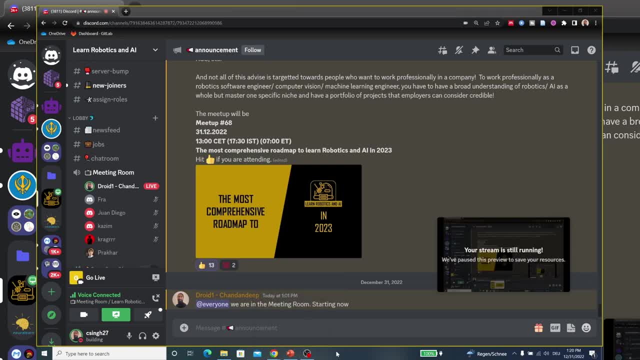 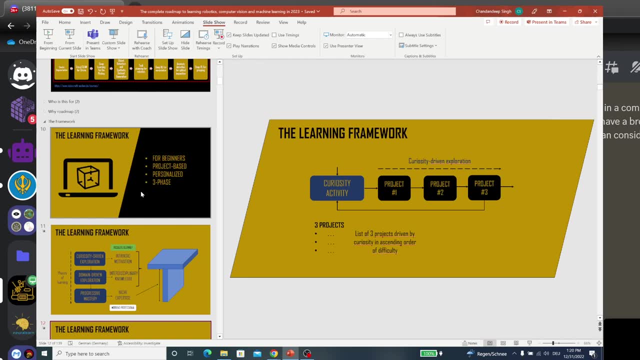 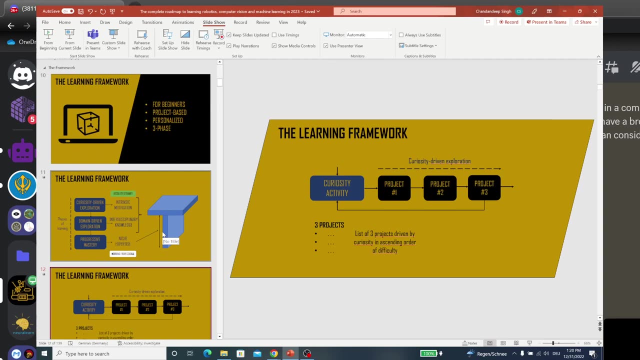 want to focus on web development, so that should not be a problem. we can take up your question in more detail uh, after the session. uh, but so far, if you have any questions related to the presentation, you can um ask: yeah, everything is fine till now, okay, yeah, so i'll uh continue with the presentation. 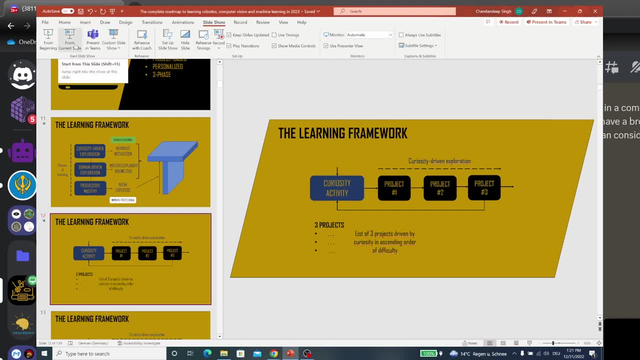 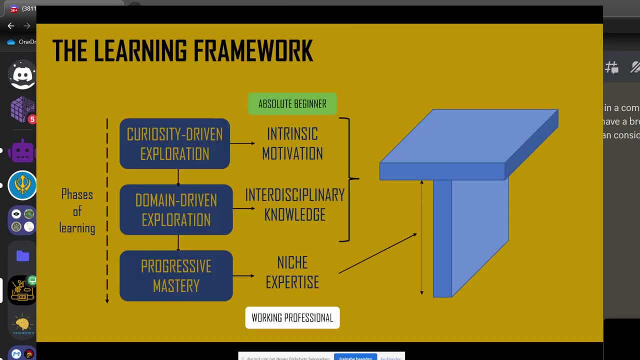 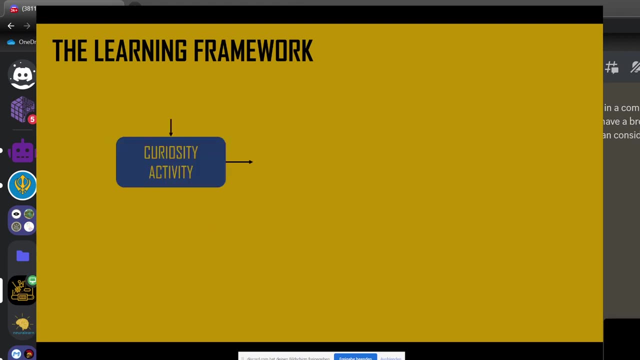 and then we can, of course, discuss at the end in more detail. okay, so we talked about the three, the. we talked about the three phases of learning that we, you, would require to focus on as a beginner. and then the first phase is curiosity driven learning where, uh, you do an activity. so i'd be sharing a little bit about the activity. 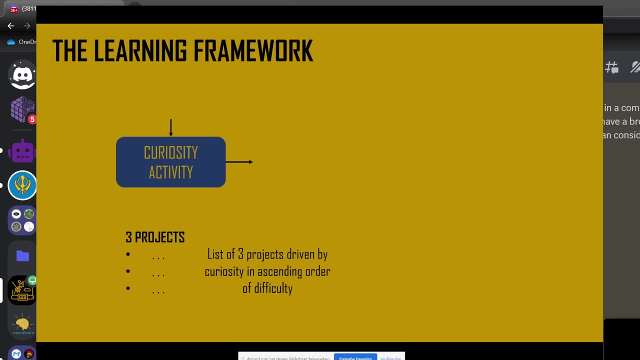 as well today and i've talked about in one of the videos. so you'd be doing an activity, a very simple activity, and at the end of the activity you'd be able to list three project projects driven by your own personal curiosity and arranged in an ascending order of difficulty. so the project number one is 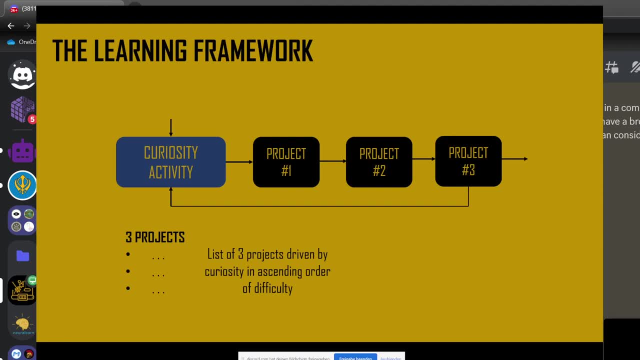 would be the easiest project, project two slightly difficult, and project number three would be the hardest out of the three, but all of these projects would be, uh, relatively easy compared to the projects that I'll be talking about later, and the main idea is that these projects would be. 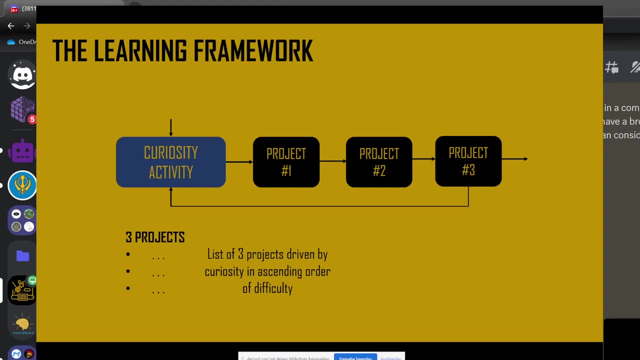 defined entirely by you, without having any reference online, just based on your own interests as per your limited knowledge at this point. so this is the initial phase. I think one should start with learning any field first of all by intrinsic, by their share, intrinsic curiosity, because otherwise you would lose interest at the end of it. and, of course, 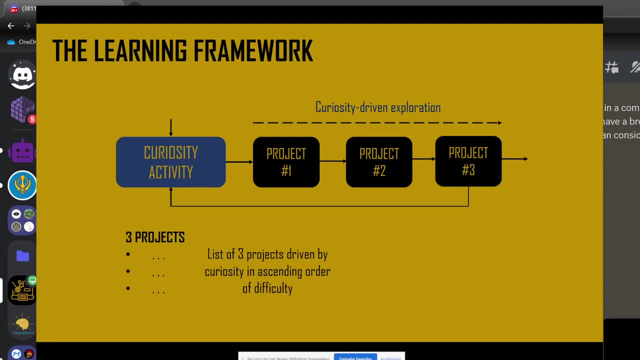 you, you would also require to explore domains that you might not be totally interested in, and those are important. but if you start with things that you are interested about, projects that you care about, you are more likely to stick with the process. so these are three projects that you would. 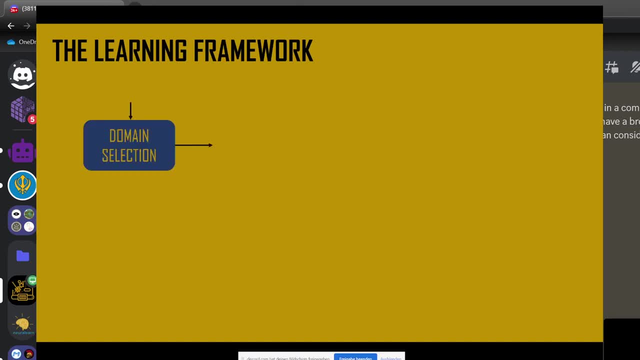 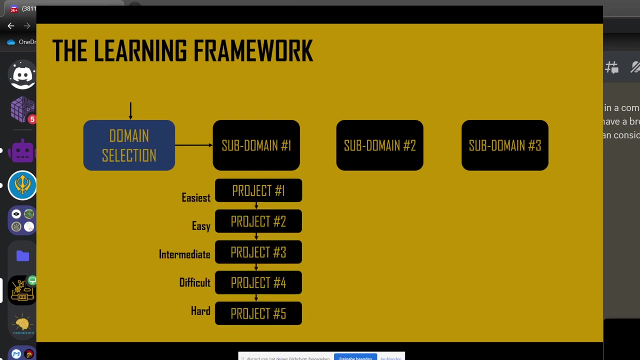 start with and then after, that is the domain driven exploration approach, and then this is you. this is again driven by an activity which would expose you to several different subdomains in both robotics and AI, and at the end of this activity, you would be able to select projects in the increasing order of difficulty in each of the different domains. 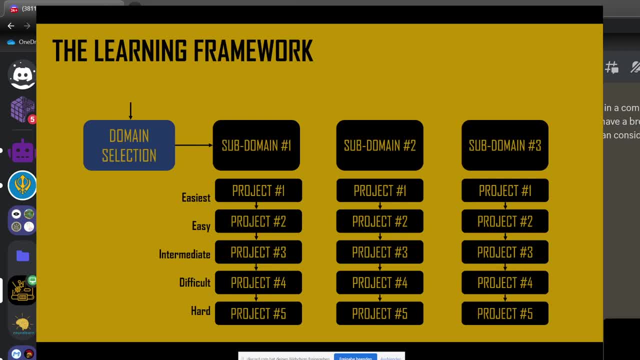 so you would have sort of lists in several domains and you would be able to select, first of all, three specific domains that are most interesting to you, and then you would have- you would be able be made available- a list of projects that you would be doing. so you would start with 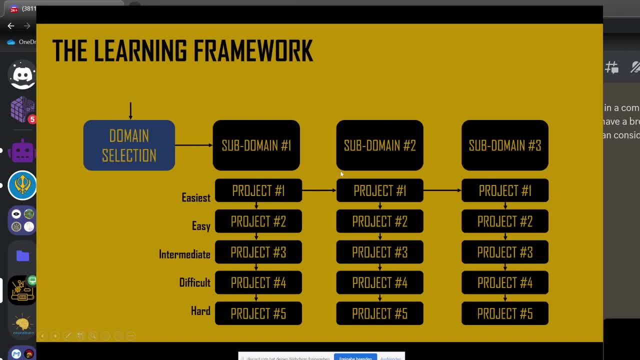 so in this phase, basically you would take up the easiest project in each of the domains. so because the idea is, you want to explore and get a sense of different domains which you don't know about yet, or which you know about, but you want to explore a bit more. so this is domain driven. 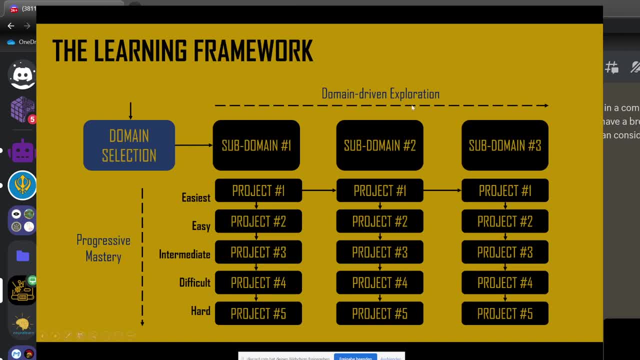 exploration and, after domain, given exploration. basically, once you try out the done that first step, try out the three easy projects in each of the domains. you would choose one specific domain that is most interesting to you and you would be able to do that because you already did some projects that would be similar to what you would. 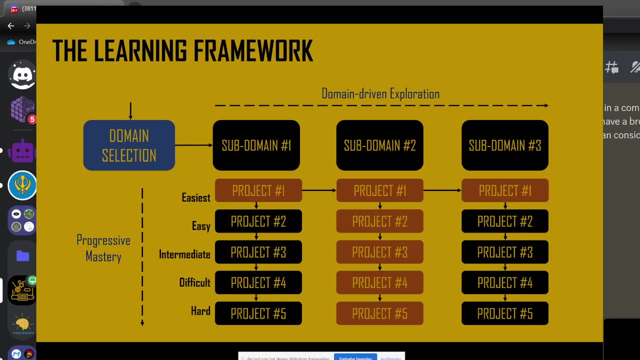 do in the industry, but on a smaller scale. so you would start with these projects and then you would take up more projects in one specific domain, and with. the reason why we are taking four projects is because you want to take up more projects in your area of expertise, and the reason for taking the previous. 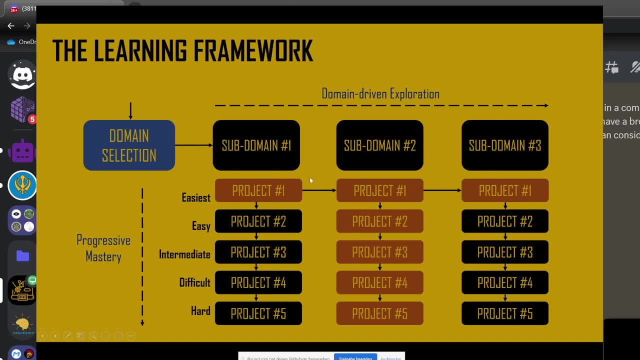 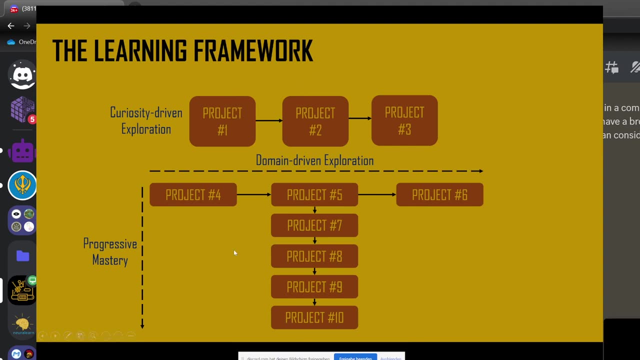 projects based basically here in domain driven exploration and curiosity driven exploration, so that you can get an overall sense of different fields and projects. so by the end of this framework you would have ten projects overall, so by the end of 2023. I'll also share a weekly and monthly plan on how you can systematize this and- but ideally it is very much. 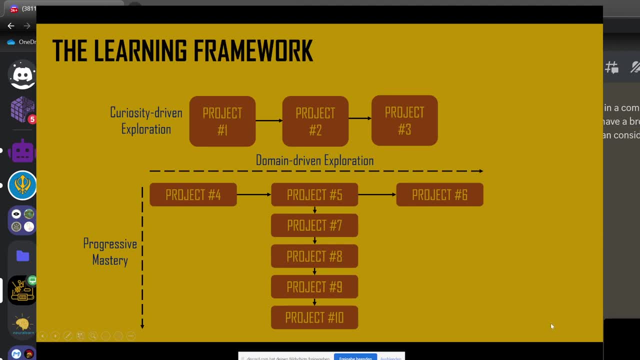 possible that, as a total beginner, you'd be able to have 10 projects in your portfolio: three projects that are curiosity driven, three projects that are domain driven and four projects of your own niche. that would allow you to gain expertise such that you can then apply for jobs. 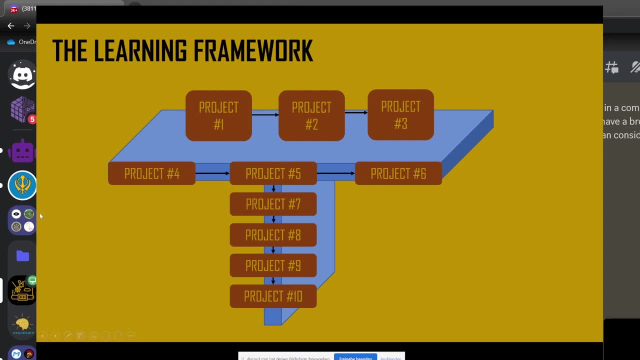 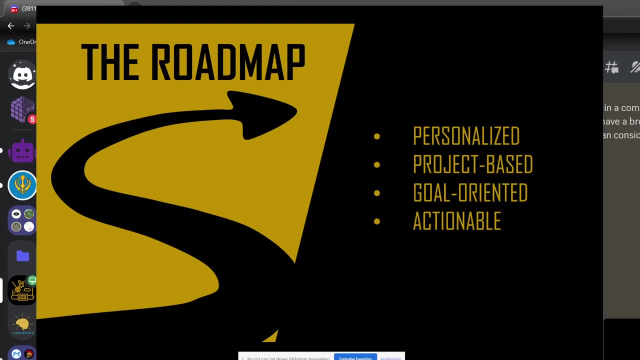 so this is in very much in alignment with the the t system that i talked about. and now let's talk about the roadmap. so the roadmap will be very much personalized. it would be project based, goal oriented and actionable. and i'll first talk about the different modules of the. 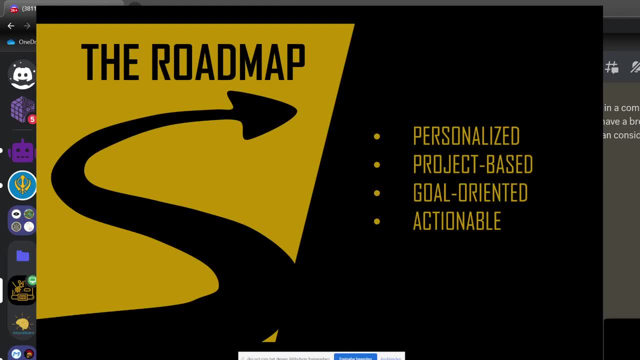 roadmap, so there are different phases of it. so the first is mindset cultivation because, as an absolute beginner, maybe you have some, uh, some limiting beliefs or some- uh, false ideas about robotics, or maybe you're not very much familiar, so you you have the right expectations on what to expect when you're learning. 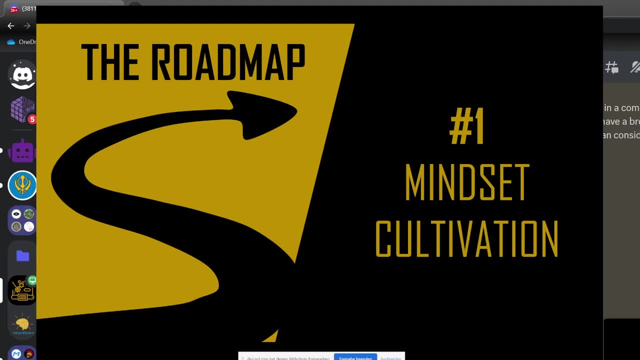 robotics and ai, and you start with the right, for the right reasons and with the right mindset, and you are also aware of the effort that it would be required and so that you can decide for yourself whether it's worth it for you or not. and after that we would be spending. 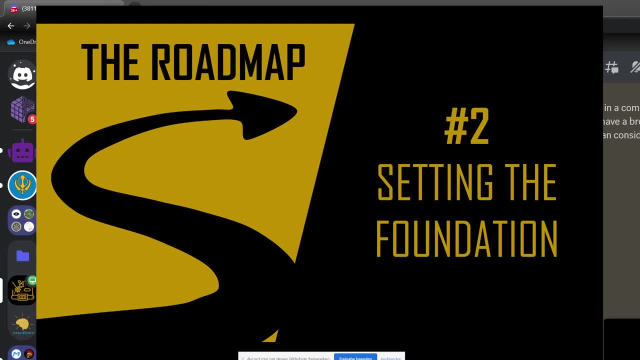 a few weeks or a month setting the foundation. so this would be: if you have zero programming experience, maybe you would spend some time building some basic programming foundation, just enough so that you can then start doing project or you can learn get or other software tools, software testing and so on- mathematics foundation. so any lack of hole. 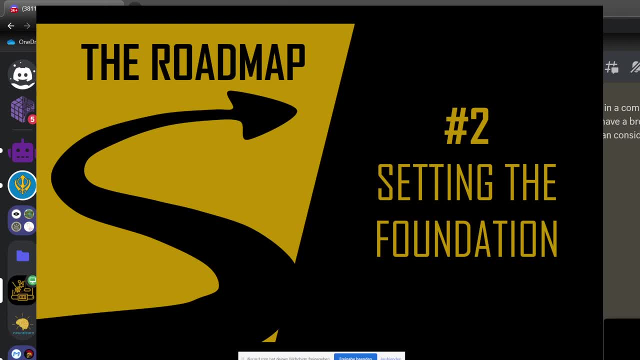 of mathematics knowledge that you have. you'd be spending some time doing that and after that, as I said, you just start with the projects and that those would be driven by your own curiosity and then after that you would be exploring several domains and doing projects in that. so three projects here, three. 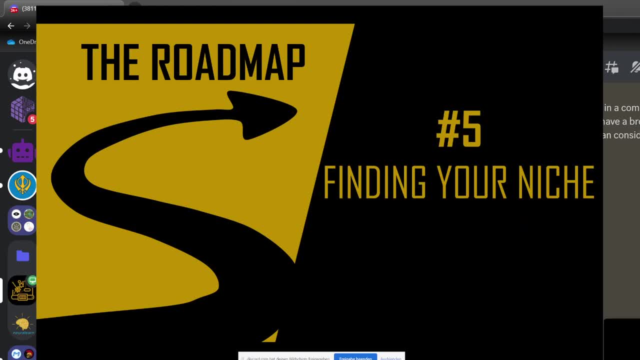 projects here, and then you'd spend some time actually identifying your niche. there would be activities for that, and then you would build the project. you would take up four more projects in the domain that you identified as your niche, and the projects would be of progressively increasing difficulty. 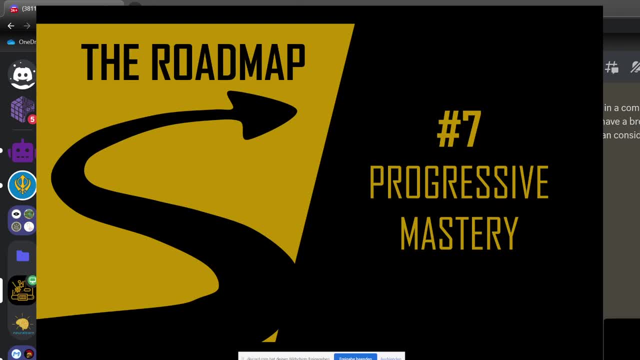 the idea would be that this is your domain, that you want to gain mastery in and want to work in the industry and also continuously improve yourself on that. then you'd build your portfolio, apply for jobs and then continue your learning even after applying for jobs, because robotics and ai are both fields that are progressing at a very fast. 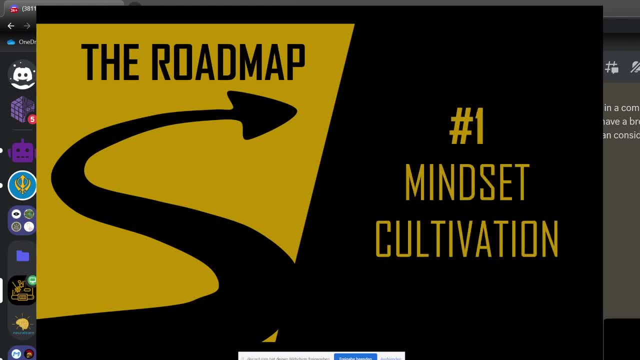 pace, so you have to be continuously learning. so this is also something to keep in mind. so let's talk about mindset cultivation. so here i'll not be talking too much in detail about the activities, because that would take up several hours, but i'll be talking about in specific what are the areas. 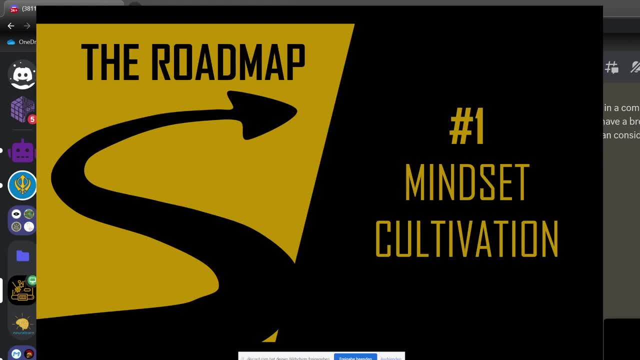 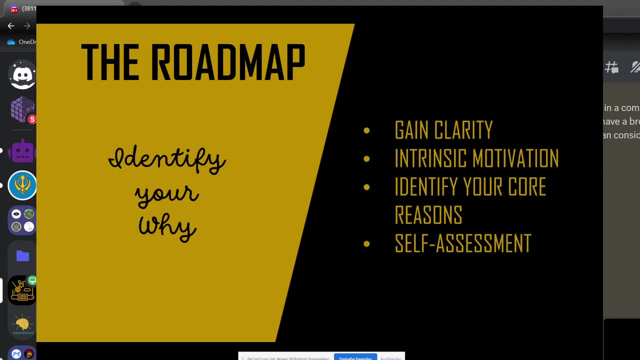 that you can focus on for 2023 and the mindset cultivation activity would be probably just for the initial few weeks and then after that we'll just get started with the technical stuff. so first is to identify your why, and i've made some recent videos where i talked about the importance of 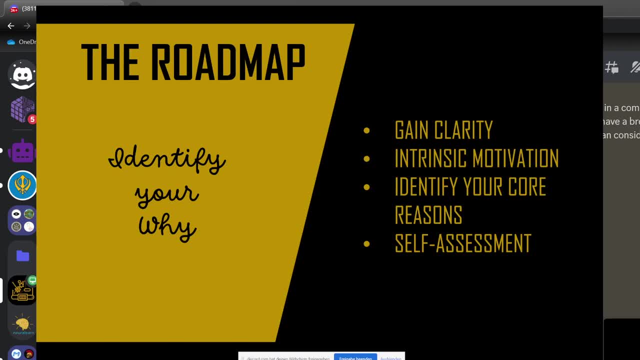 identifying your why and gaining real clarity as to why you really want to learn these fields, your core reasons, and making sure that you write. you start learning for the right reasons, and these would be based on self-assessment activities, so you would be doing the activity by yourself. it's not like somebody will tell you some mooc. 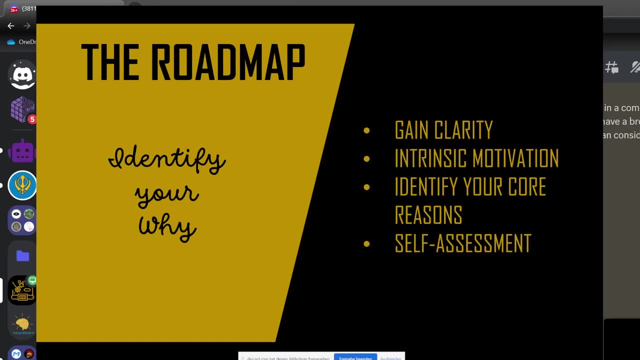 would tell you the reason why you should learn this is because it would. there are this and this job opportunities and you would be earning this much, and so on. you would be doing the activity by yourself and you would be asking yourself questions to identify these things and i think 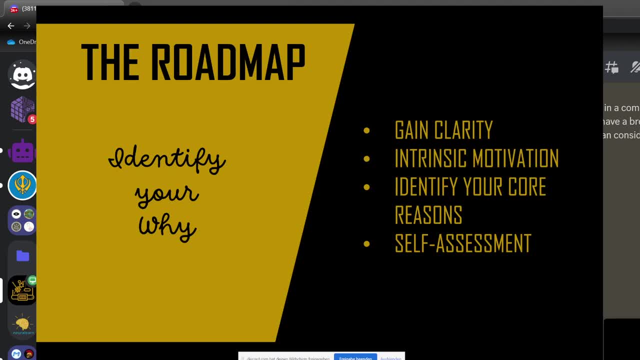 this is extremely important as a starting activity, because maybe you realize this is not for you and then you could focus on other things, like maybe web development or other domains, which is absolutely fine. but it is important to make sure that you understand what you will be focusing on, because you'd probably be 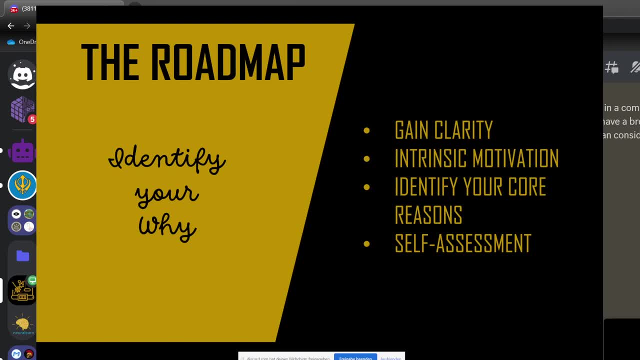 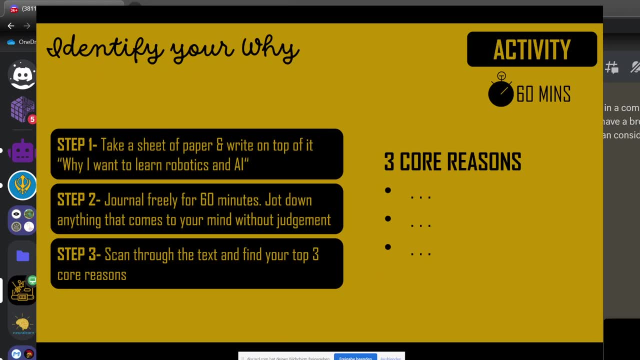 wanting. you'd probably be learning and learning different things throughout your career, so that is extremely important to focus on, and one sample of this activity is to understand the activities that you would take a sheet of paper and write on top of it why i want to learn robotics. 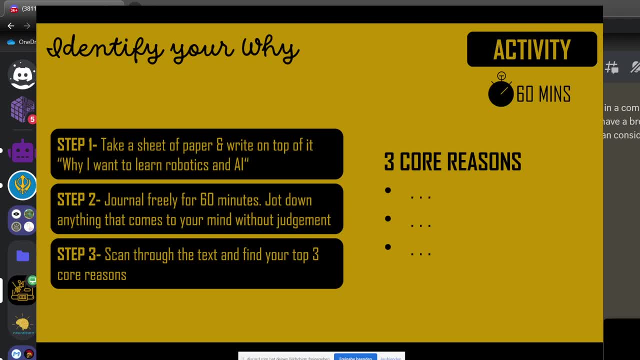 and ai, and of course i've written robotics and ai as a vague term here, because the idea is initially, you don't know which specific field in robotics or ai you want to learn in, you want to learn basically. so then you would free journal for 60 minutes or even two hours, take as much time as you. 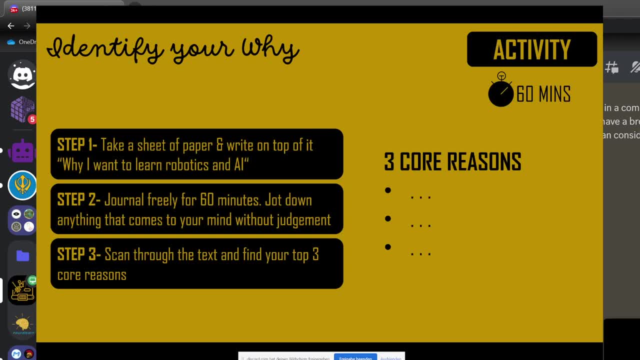 need. this is just something that you would do for once, and then you would jot down anything that you have in your mind related to the topic that you wrote on the top- why i want to learn robotics and ai- and you would collect all the points without any judgment, anything silly that comes into your 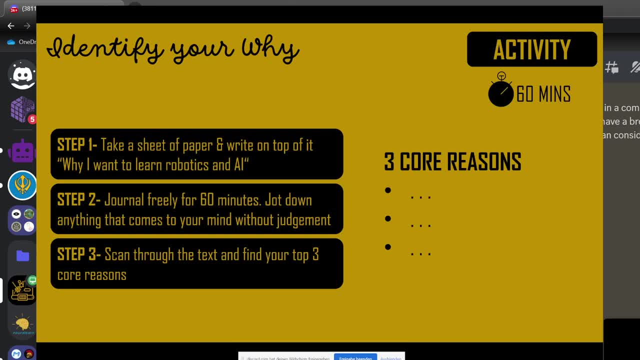 mind- you just collect those thoughts and then after that is when you would be evaluating that- you would be scanning through the text and find your top three core reasons. now all of this might sound a bit vague, but at the end of this session i also have a little case study where i've taken a 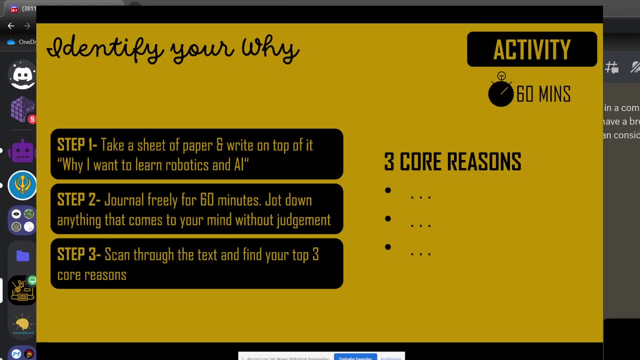 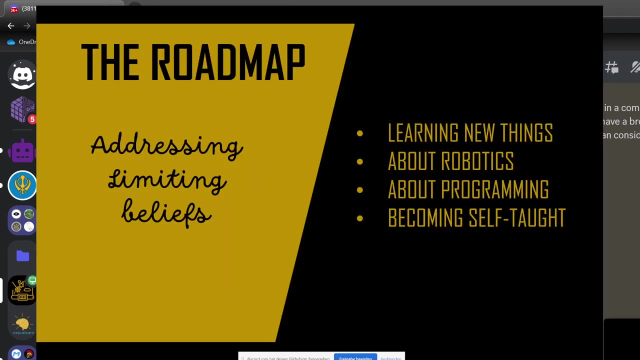 person who's an absolute beginner- and i have. i have tried to cover all the different aspects of this roadmap that the person might use to solve the different modules of the roadmap, basically. and then the module is about addressing limiting beliefs, so as, with learning anything new- whether you're learning a new sport or new programming or something like that- you're going to 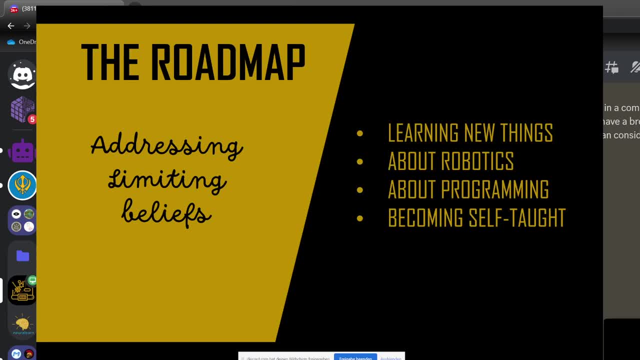 learn a new language- or a new language, in fact, anything. there are some limiting beliefs. you know that. you might think, hey, this is not for me, but it's too complicated, i'm not built for this. so it's. it makes sense that you spent a few days at least just addressing it and getting rid of the limiting. 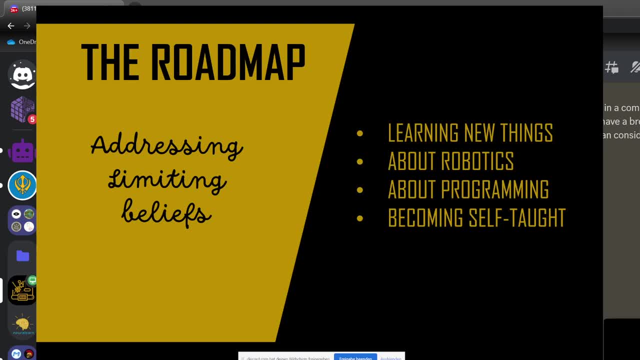 beliefs and just start with the right mindset. so we are still in the mindset stage here. so you might have limiting beliefs about robotics in general, because when people think about robotics it's it looks so cool and interesting, but at the same time you might think, hey, this is. 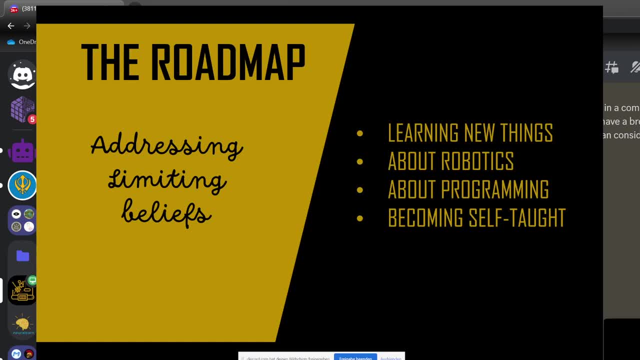 too complicated. i can never do that, and so you make sure you address all of these things. and about programming, another thing is, yeah, i cannot do programming, programming is hard, and about being self-taught: that it's not really possible to become self-taught, and 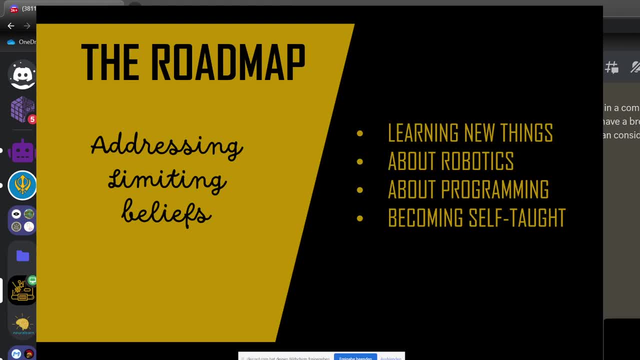 that i need a master's or a specific set of courses. you you can become self-taught, and the reason why i'm i can confidently say that is because, even though i had a systematic master's, a majority of my journey was based on the experiences that i got by taking part in. 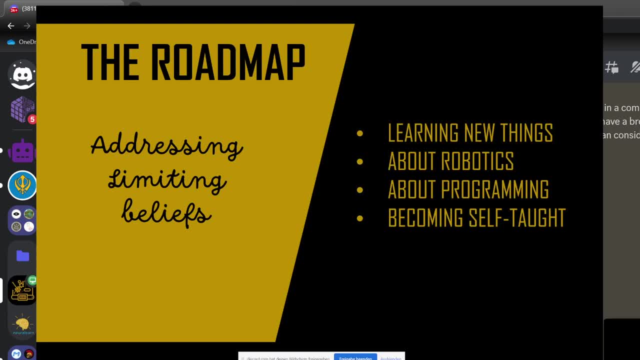 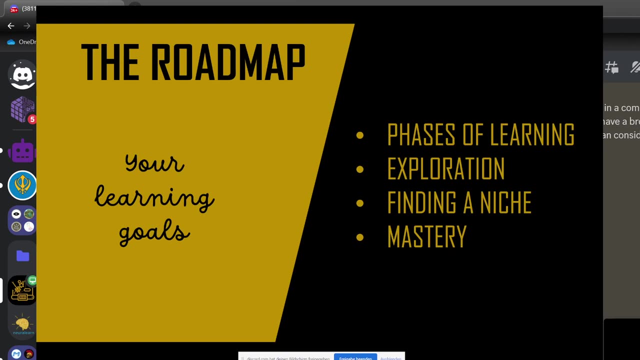 projects in the industry. so that is extremely important to take care of in the very initial stages itself, because you probably not be dealing with it later in any case, and then you should define your learning goals. which phase are you? are you exploring just several areas of software in? 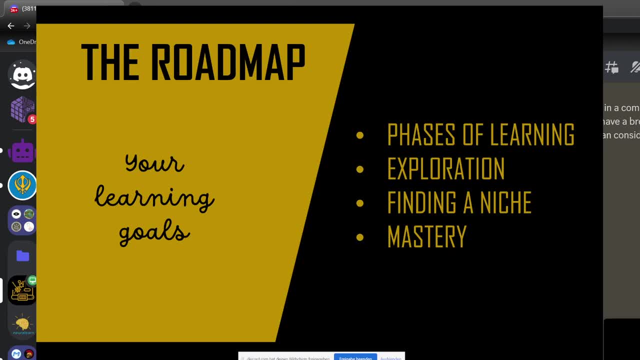 general? are you exploring blockchain? are you exploring blockchain? are you exploring blockchain, web 3, web development robotics or are you exploring specifically in robotics? do you have some level of clarity that i want to work in machine learning, but i want to explore and understand what specifically i want to do in that, or or is it everything totally clear to you? 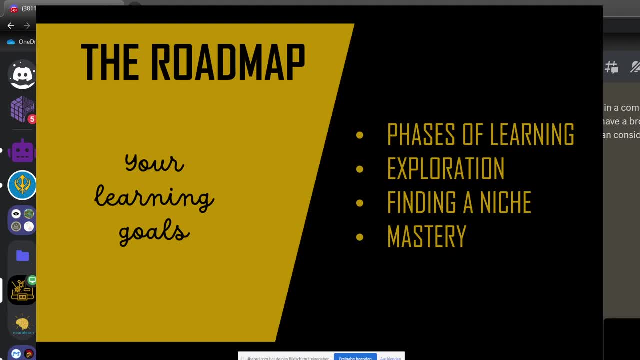 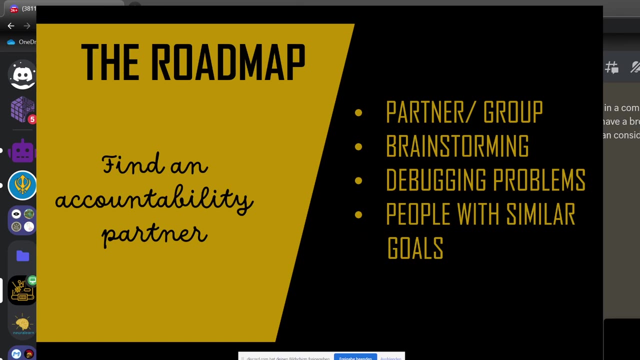 and you want to focus on gaining mastery and based on your goals. the roadmap, the 2023 plan, might look different, and that is the whole idea behind it: that you can make a personalized curriculum, personalized plan for yourself, without the assistance of anybody and, of course, the whole. 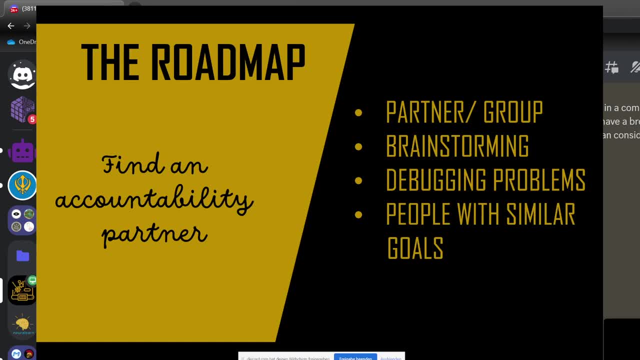 process is such that, since you are, you want to learn these things on your own. you might get stuck. you would definitely get stuck in at different stages of it. while choosing projects, by which projects to focus on, while doing certain activities, while brainstorming ideas for the projects, while 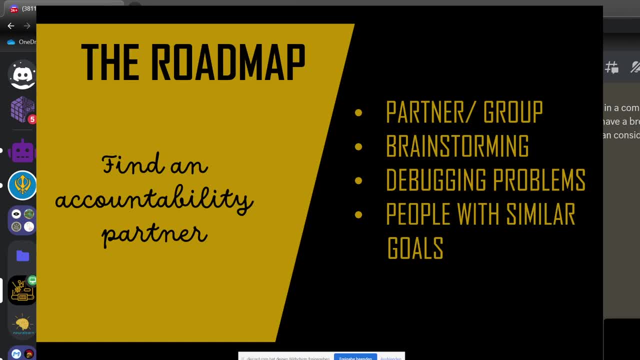 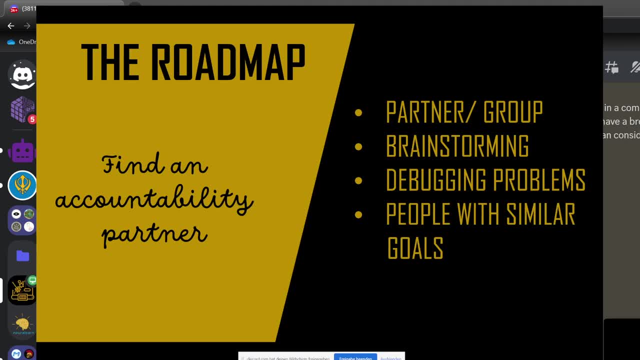 long way. and this is the exact reason why universities do so well: because all the students have more or less similar goals as you, so they keep you accountable. you have exams, you have lectures scheduled that you would want to attend, that you would have to attend, and so on. 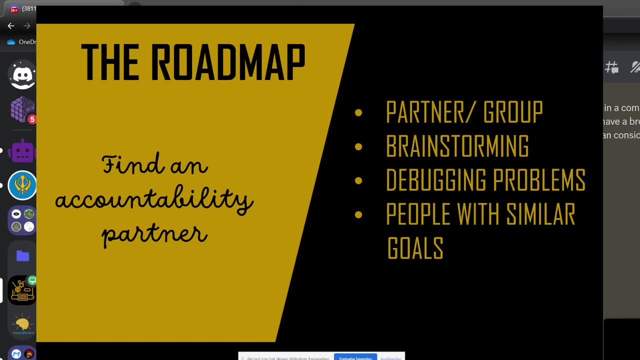 but if you want to be a self-taught uh engineer, robotic software engineer, CV ML engineer, then you have to make sure that you take this into consideration, And it is very easy to find accountability partners because we have this. 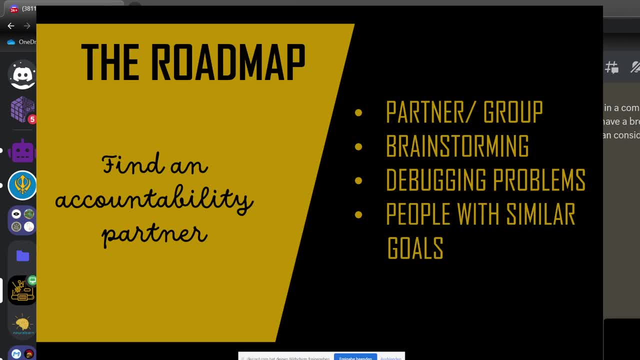 discord server. You can find people on LinkedIn. you can find people on Reddit forums, You can find people on Facebook groups. So there's just a lot of possibilities. And in today's day and age, if, uh, if- you're not able to learn things on your own, 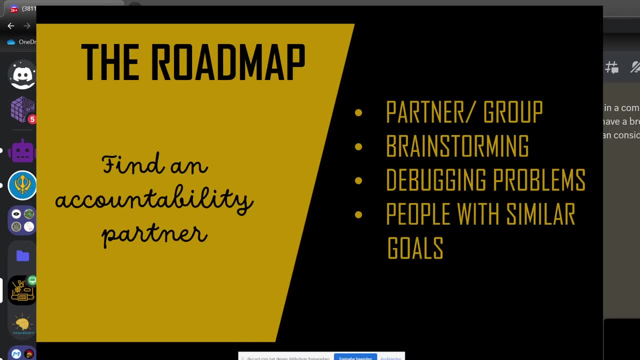 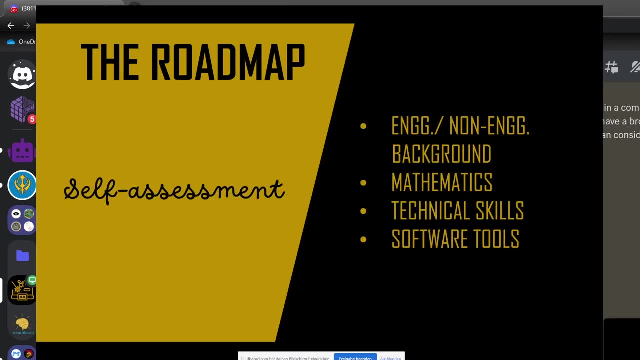 then you need to be more disciplined and just stick with the plans because, uh, it is very much possible if you have the right system. So setting the foundation is the next stage, as I mentioned. So you'll be doing some self assessment, taking up some surveys. 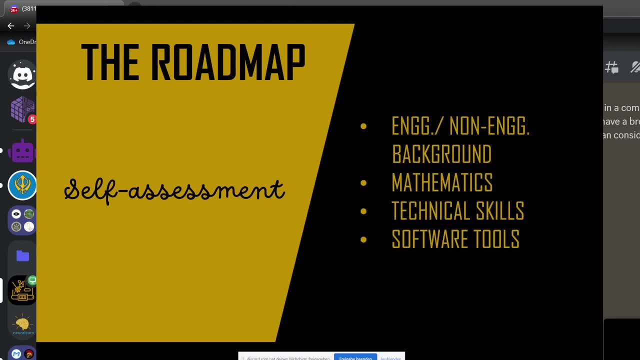 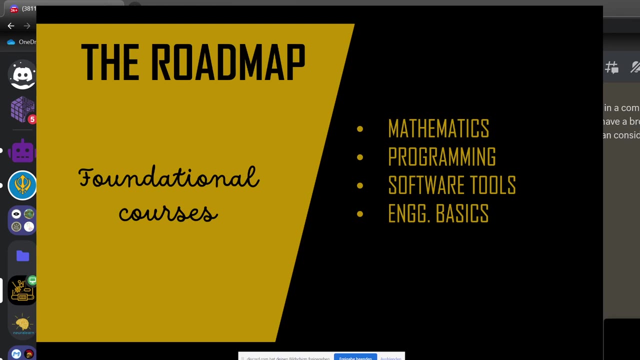 some small tests to identify, uh, how good your engineering skills are- mathematics, technical skills with regards to robotics or machine learning, software tools- And then you would take up some basic foundational courses, and this would be just maybe three weeks or something, And then you'd just fill in the gaps And uh. 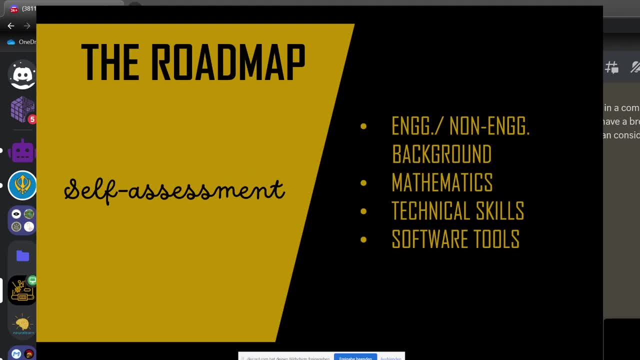 I want to mention that, uh, even if you don't have any engineering background, you could still fill in the gaps with basic mathematics, calculus, linear algebra and so on and some programming. It's not. it's not too hard, Uh. 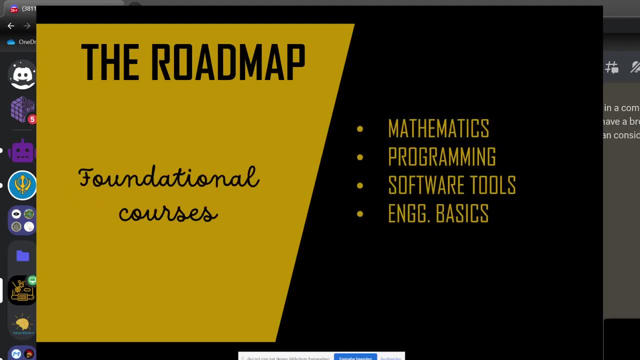 fill in the gaps, because then the main learning would be when you take up projects, and for that you would be spending several weeks. so and you're you have to remember that you're dedicating the whole year, whole of 2023, for your learning. so it is very much possible to do it as a non-engineer. 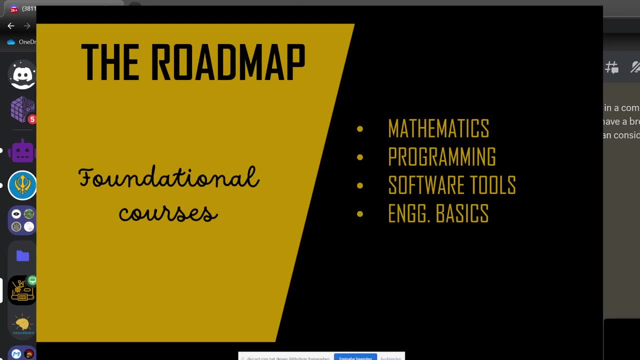 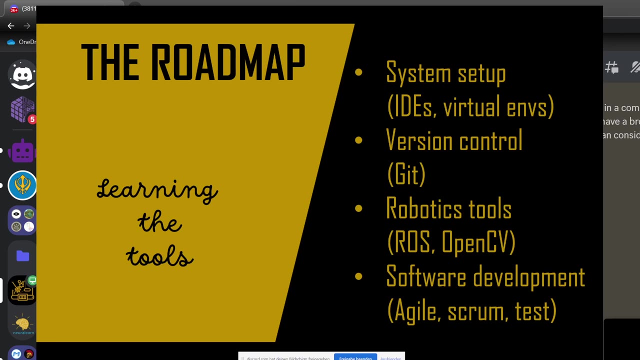 as well. but you have to fill in the gaps in foundation by taking up some courses, some projects or some way of learning in general. then you would spend time learning the tools. you would set up your system. you would learn git. you would learn some basic tools like ross- open cv, just to. 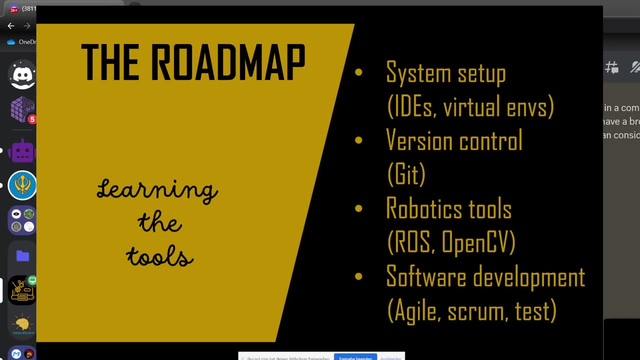 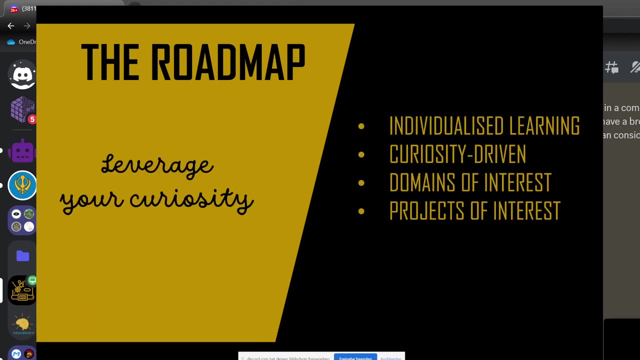 familiarize yourself with, not in too much detail. you'd maybe learn some software testing, agile development, scrum framework, if needed, and after that you can just start with focusing on the projects, and then you would spend time learning the tools. you would set up your on your curiosity, curious, exploration and and basically, the activities. 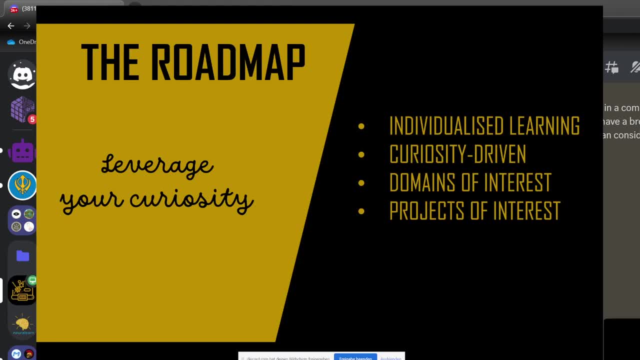 are more complicated to design, and then i have not shared the activities in too much detail, similar to the one activity that i talked about leveraging your curiosity here, but the idea is that there will be activities that you can do to ask questions, such that you would be able to find fields and projects that are of your interest. 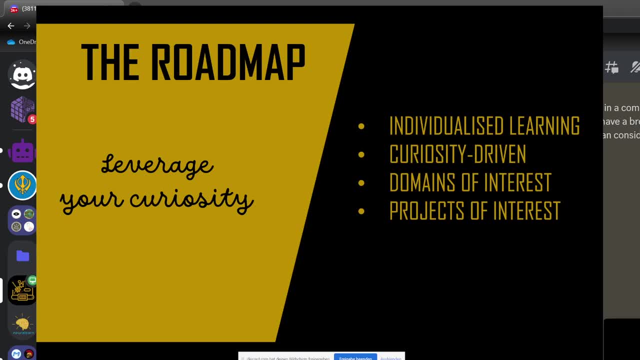 and these could be as simple as what are the areas that i'm interested in, what are the problems that i'm currently facing, what are the things, what are the projects that i'm doing currently that i could automate, and these could be general programming related, or maybe it could be more. 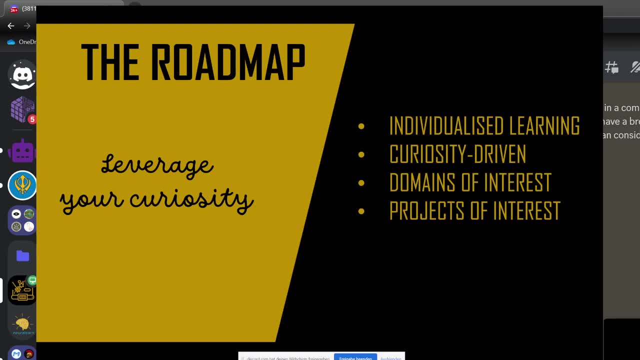 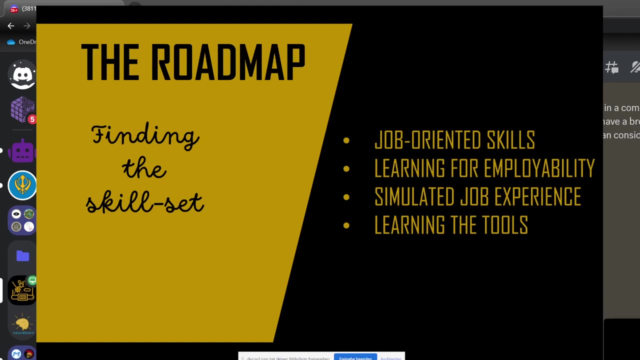 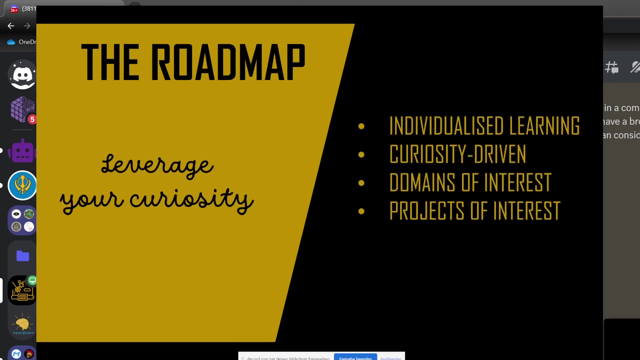 robotics related or machine learning related. there are several ideas that you could have, and the idea would be to leverage your curiosity, first and foremost, and then after that- and this is very critical- that you identify the skill set that would be needed for you to work in the industry, because you could come up with some projects out of your own curiosity that you of. 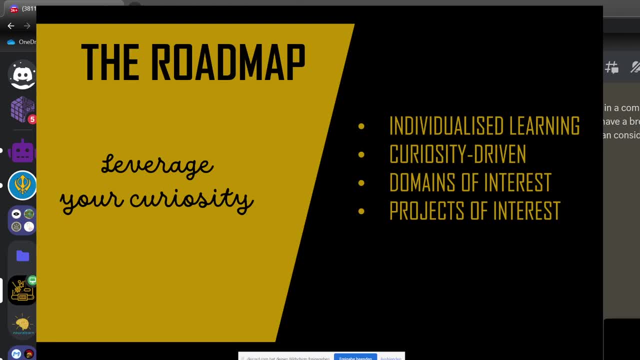 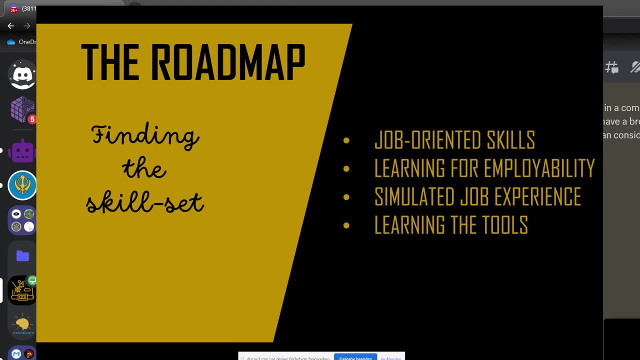 course find interesting and you would maybe stick with it and finish it, but it's of no use if you, if your goal is to work in the industry, if you want to work in the industry, then you also have to fine-tune the projects that you come up based on your own curiosity and then make sure you focus. 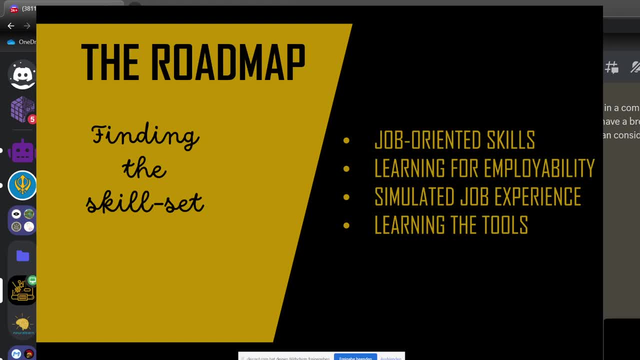 on the right skills. so an example would be that you came up with a machine learning project for segmenting like your family photograph, like people in your family photograph, just out of your own sheer curiosity. but then you spend some time evaluating the different companies that are using image segmentation and so on, and what are the tools that are? they that they are using are? 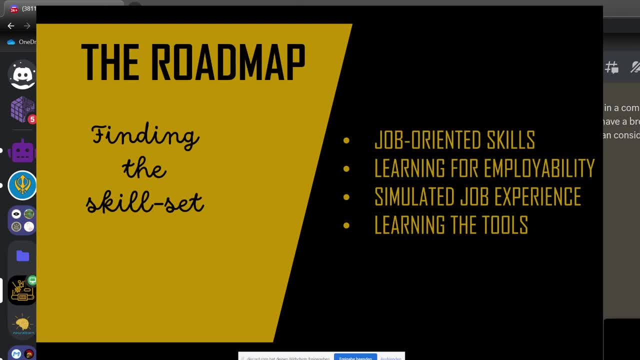 they using py torch? are they using more of tensile flow? are they using Python, C++? what are the different tools, frameworks, programming languages that they are using? and then you would update the project that now the project would be more like here to do a segmentation of people in in my family photo. but I'll use tensorflow and Python, Python. 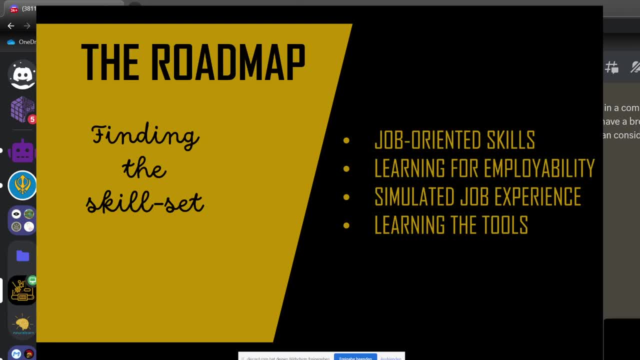 for that, because that would also make me employable based on this project. so this would be it, and the idea is that you would be getting simulated job experience, which means that you would be doing projects similar to the ones that are used in the industry. of course, they cannot be totally exactly. 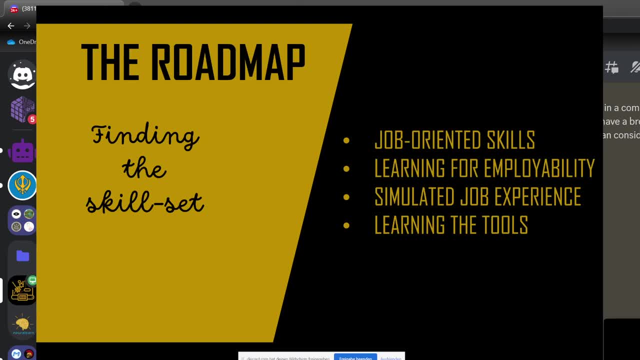 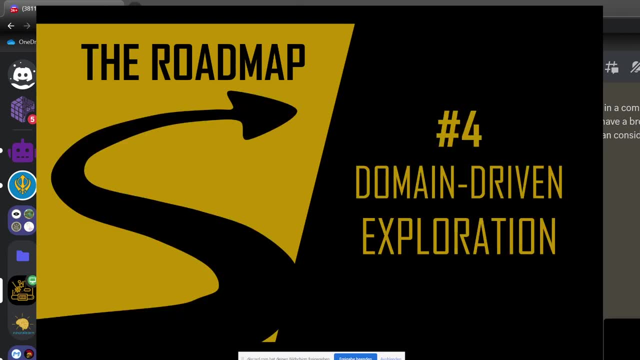 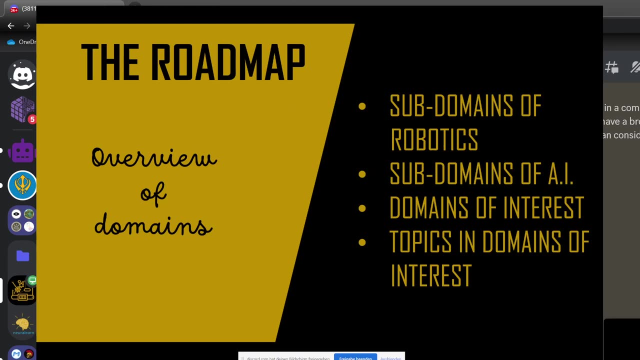 they could be very similar and you can learn the tools and that would make you employable. so the right job oriented skills and then after that we would be focusing on domain driven exploration. so you'd be getting an overview of several subdomains of robotics and I've been wanting to make a video. 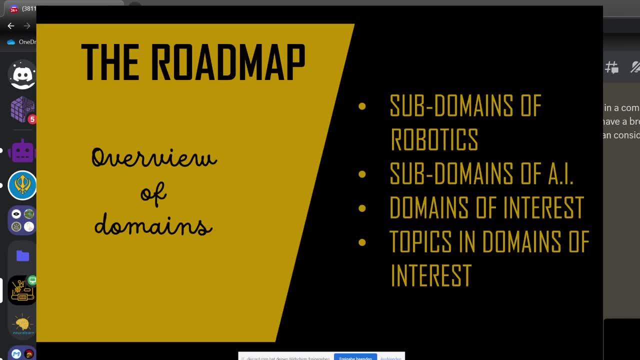 for this like a comprehensive overview of several subdomains- but I'll do it in the future as well- and then we would be selecting three specific domains that you find most interesting, based on just the applications that are in that domain and just what interests you, based on what's going on in the 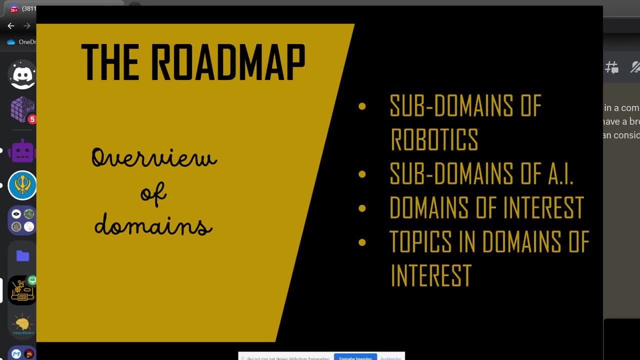 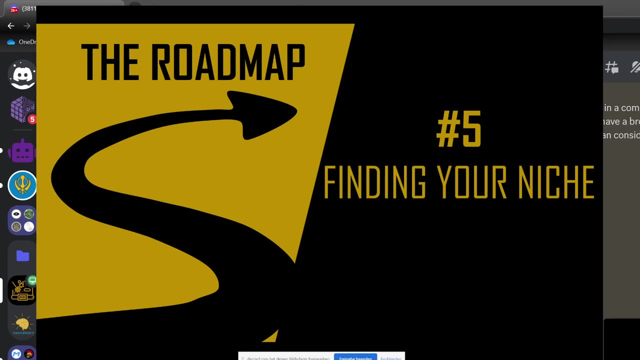 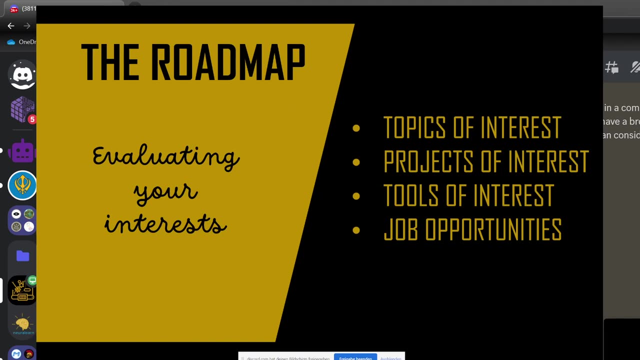 industry, and then you just choose these three domains and then you would take up simple projects in these domains and then, after doing these projects, you would spend some time finding your know in these domains. and then, after doing these projects, you would spend some time finding your niche, evaluating your own interest, evaluating the topics and projects that you did, exploring the job. 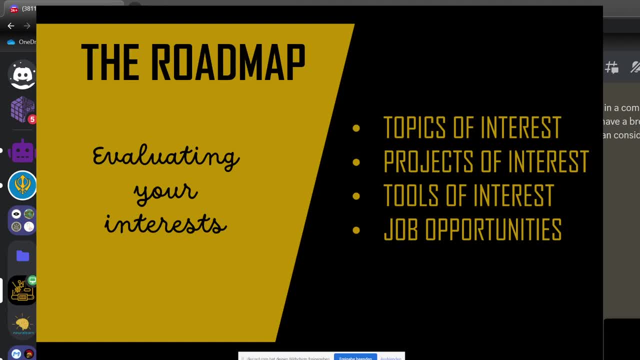 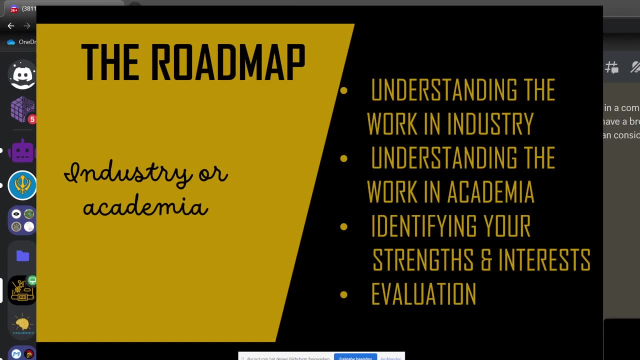 opportunities and then fixing your niche and then spending some time also identifying whether you want to work in industry or academia very early on in your learning journey, so that you focus on the right things, because for academia, you would probably want to focus also on research and reading research papers. publications are the most important thing, as you know, and if you want to work, 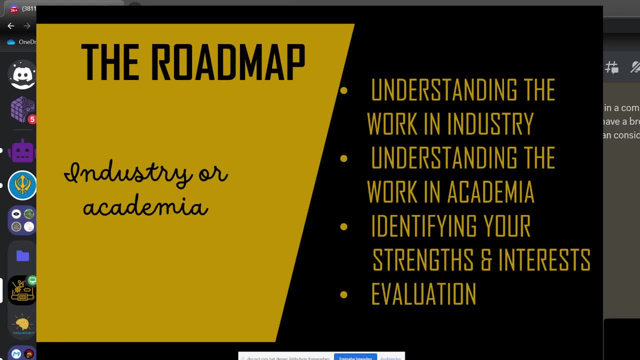 on as an engineer you would want to work, focus on learning the right tools, the skill set and, essentially, programming- you should be really good at programming and software development- and and, of course, also identifying your own strengths and weaknesses, you and which area you would be most suited to. and, of course, all of this might sound a bit vague, but we'll. 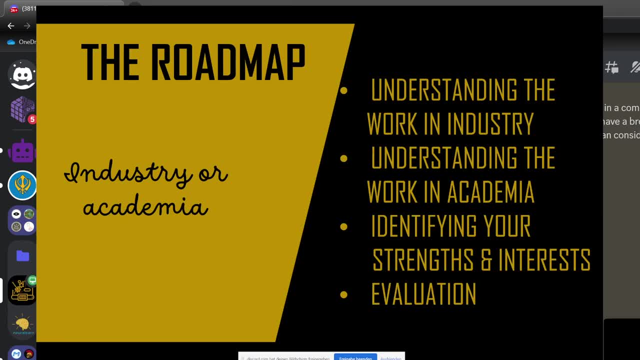 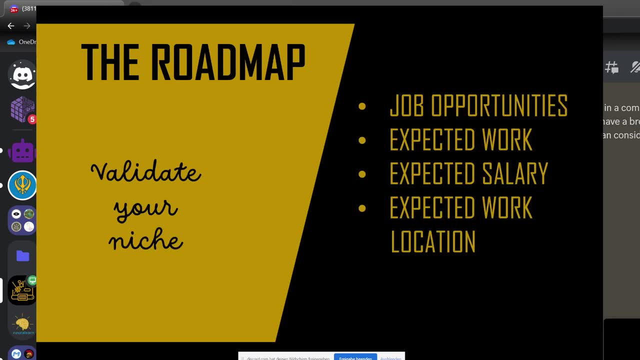 cover a case study at the end of it and which will connect everything together, and there will be activities as well, which I have not covered in this session. and then you would validate your niche based on the expected salary, expected work location, where you want to work the job. 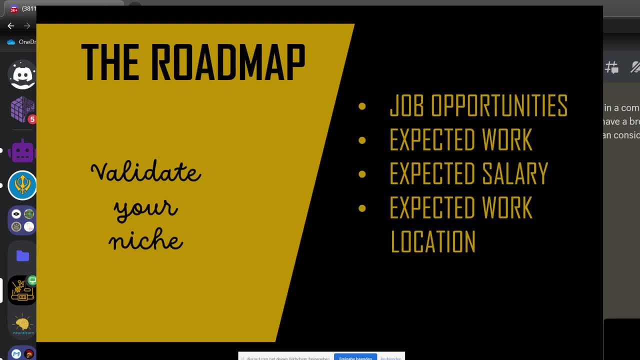 opportunities and your own interest, interests. so you'd validate whether you, the niche that you chose, is it something that is worth it? is it worth spending so much time and effort actually mastering this very specific subdomain because you could take up something as niche, as deep reinforcement learning? but then you should. 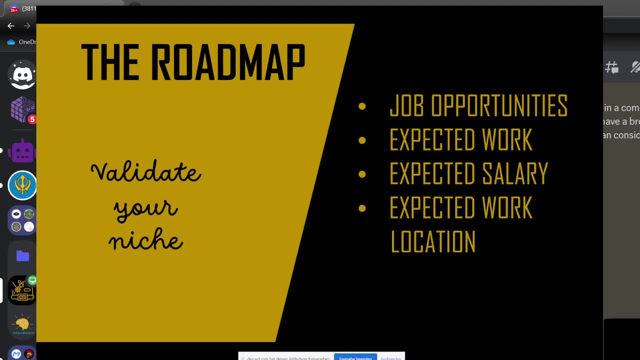 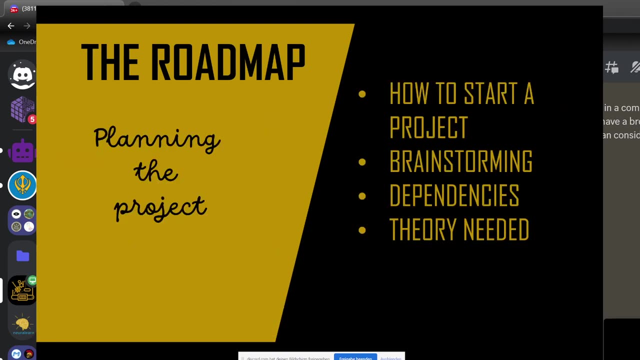 realize that there are not many jobs in the industry for that you, if you want to work in research, then that is probably something that you could do deep research in, but for industry it is not used that often. so that would be one example, and then you would build the project. 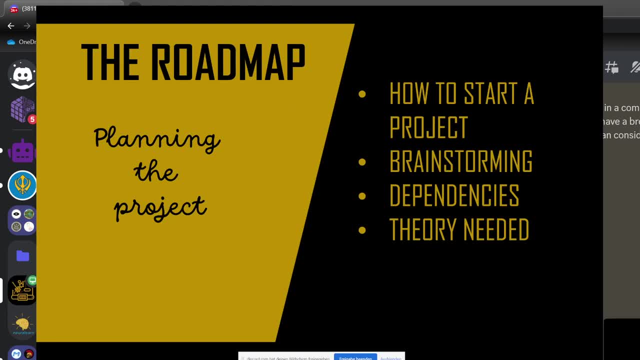 starting with planning the project, and then that would consist of brainstorming, finding the dependencies that you require for this programming project, identifying what is the necessary theory that you would need, and that is also one of the core ideas that I talked about: that you don't need to learn all. 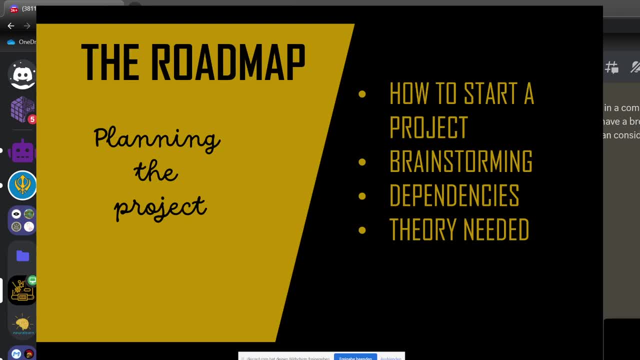 the theory. so you would be deciding what are the theoretical concepts you need to learn and only focus on that. only focus on the theoretical concepts that are needed to solve this particular project that you came up on your own or from domain driven exploration, or from the progressive. 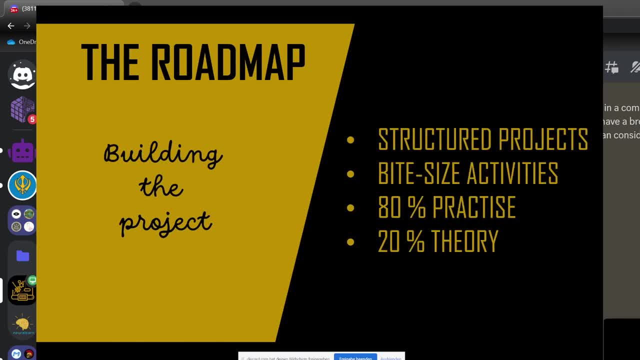 mastery stage. so it would be 80% practice, 20% theory, and the projects would be structured in such a way that each project is broken down into activities, like the one project that i conducted in one of our previous meetups about face blur. and you could, bro, if you break it down into activities, that would be essentially very 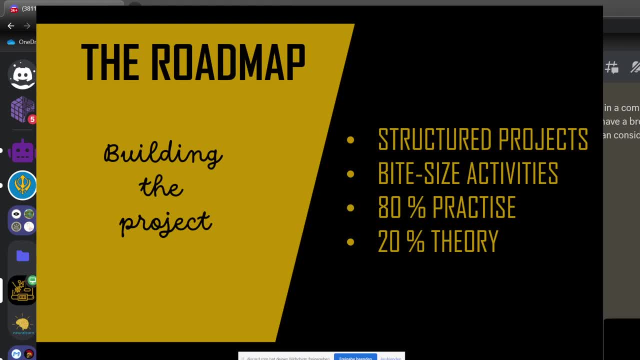 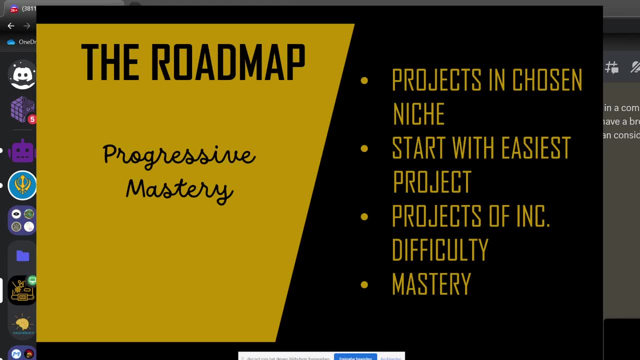 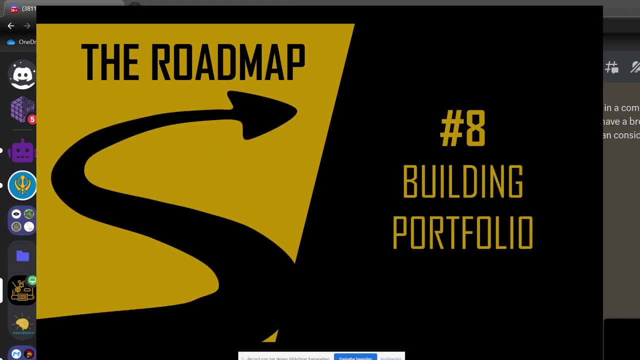 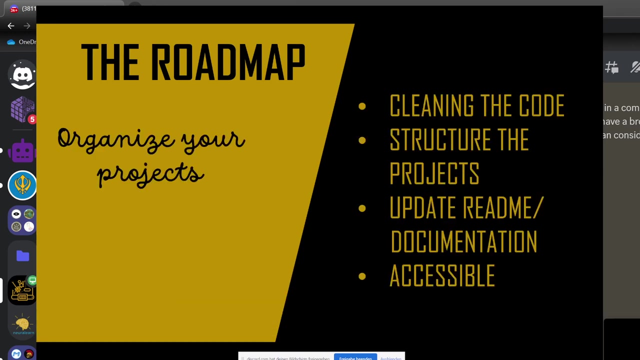 easy for you to navigate the project and then, after that, progressive mastery and you decide the projects in the chosen, chosen field. start with the easiest project, increase the difficulty and then spend more and more time, as much as you can, on mastering this specific niche. you build a portfolio, you clean the code, organize the projects that you built so far. 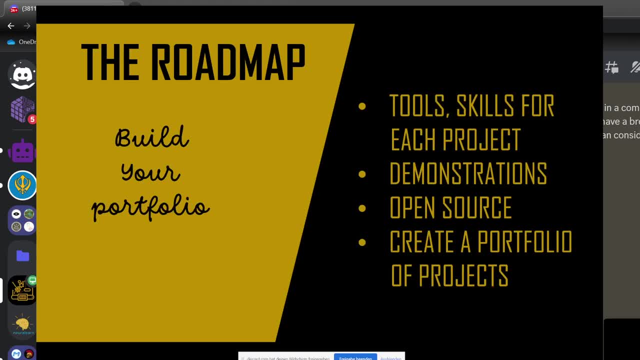 update the documentation, make it really neat and structured. you update the tools and the skills that you learn. for each of these you maybe open source it, you upload it on github you have. you add video demonstrations or or pictures of it. you create a really nice portfolio of projects and then you link it with your own web page where you would have your 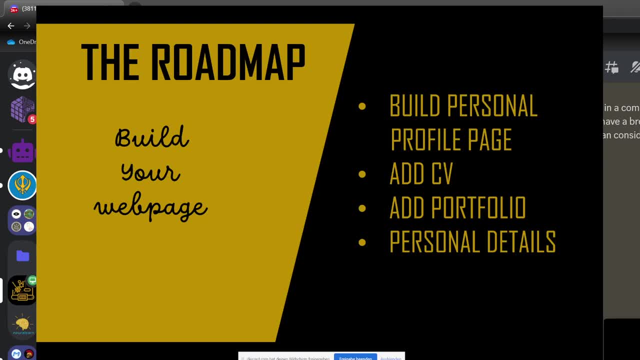 cv portfolio and your personal profile page with all the details, and that would make a really comprehensive, strong profile. i don't see any reason why, if you have a strong portfolio of 10 projects and organized in a systematic way, that you cannot get a job by learning on your own. i think this is extremely. this is very much possible. 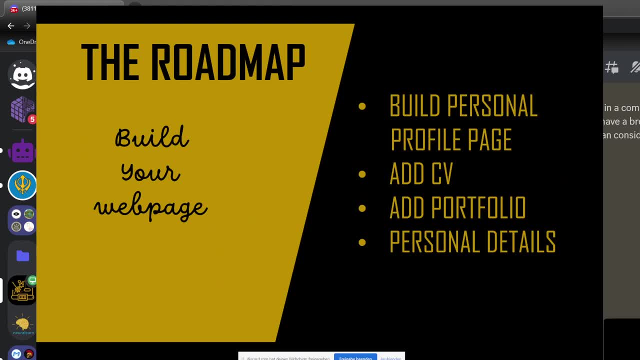 and even if you are enrolled in a university program, you have to do these things on your own anyway. so if you do the projects on your own, it's very much possible to be a successful entrepreneur. and then you have a strong portfolio of 10 projects and organized in a 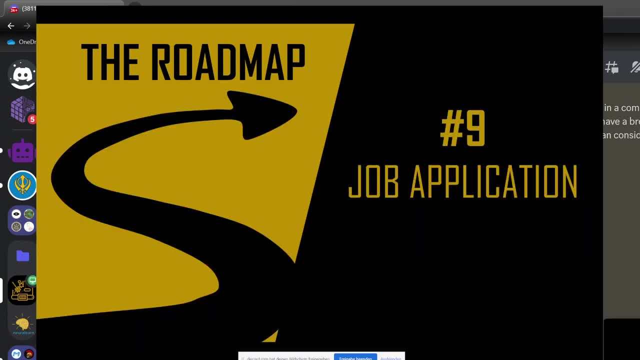 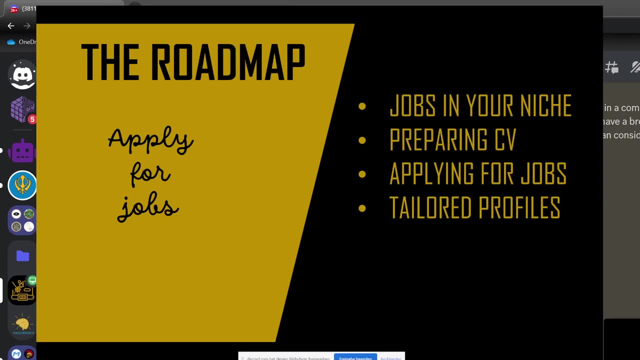 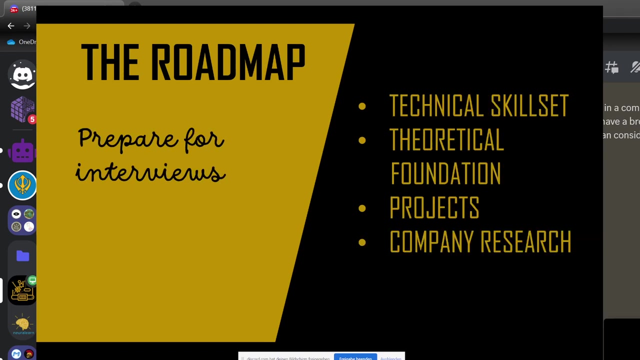 self-taught robotics software or cv or ml engineer. then of course, you would apply for jobs, prepare for, prepare your cv. you would be making tailored profiles for different jobs. maybe you want to still consider two or three different applications of robotics or different types of companies that you would consider you'd prepare for interviews, and interviews would be consisting. 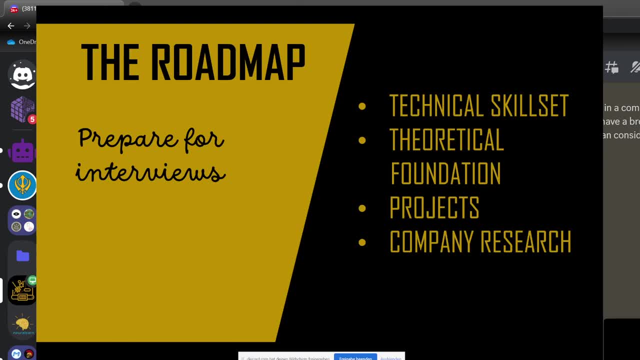 of your technical skill set, the theoretical topics in robotics and ai. you'd be learning to explain your projects. you'd be doing some research about the company and how those can be linked to the projects that you do and how to present well, and this would require maybe a few weeks and so. 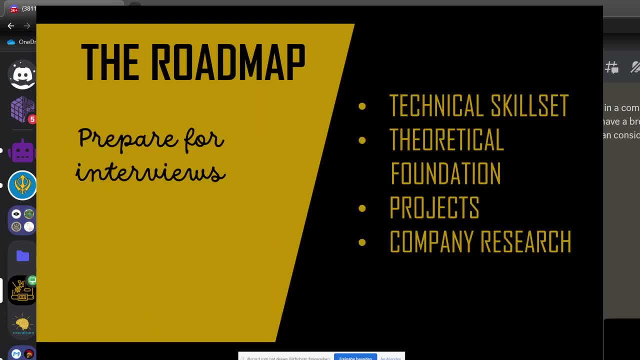 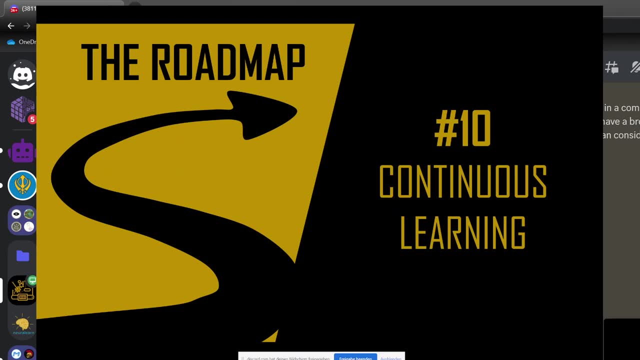 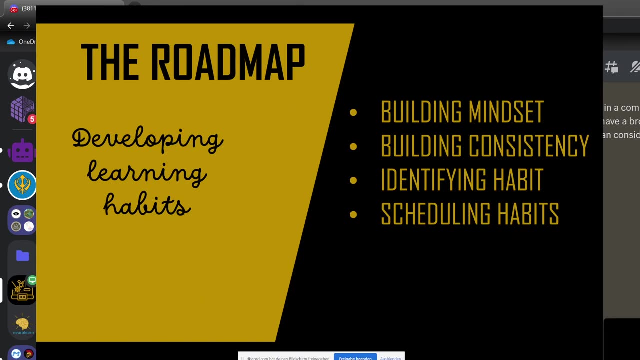 on for this and if you, if you have already built great projects, i think this phase should not even take that much time. you, and then after that, once you get a job, you'd be continuously learning, you'd be developing learning habits, scheduling those scheduling programming blocks in your calendar so that you 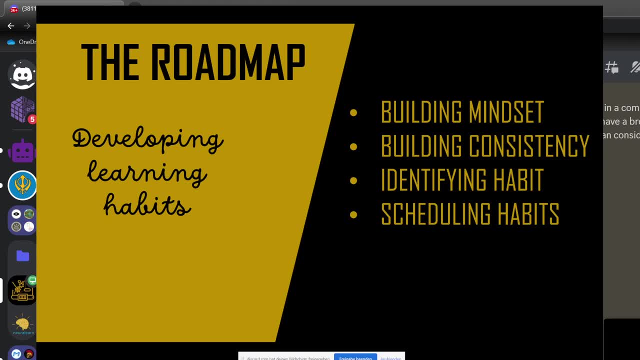 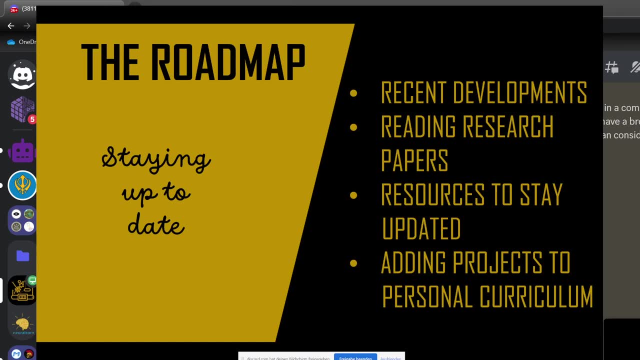 you at least spend some time learning something new every single week. you'd be wanting to stay up to date with the recent research papers, recent developments, adding projects to your personal curriculum and just trying out new projects again and again, trying out different domains and so on, and scheduling. 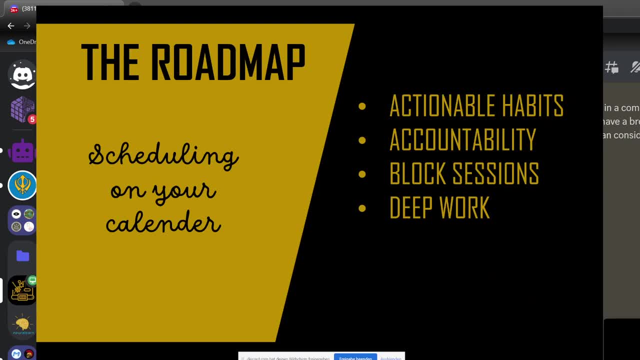 things on your calendar, doing deep work sessions, because for programming you would sometimes need maybe two to three hours to focus on a problem, and that would be more efficient rather than taking up 20 minute sessions with pomodoro. of course, you can consider this yourself, based on: 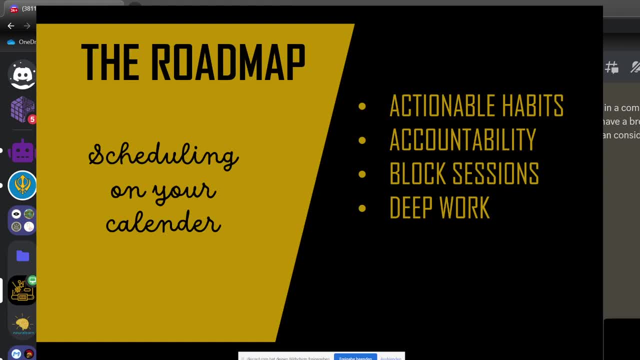 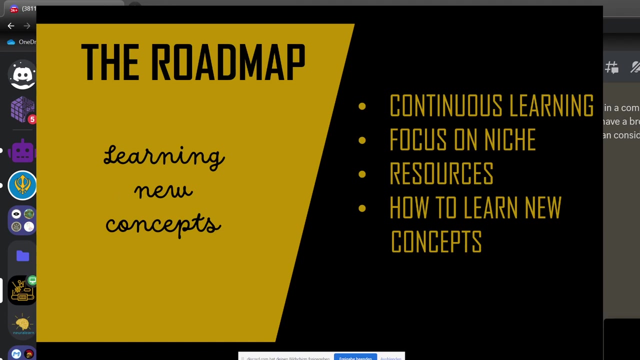 your way of learning, but for programming it requires deep, deep, focused sessions as well, and scheduling things on your calendar would also make you accountable. if you stick with it and cultivating habits, that would make you learn, that would keep you learn, that would allow you to keep learning throughout. so again, learning new concepts. 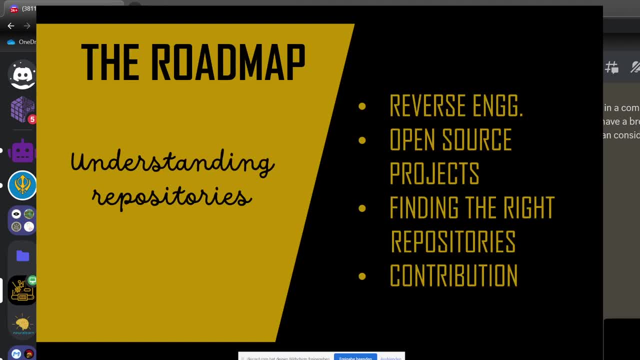 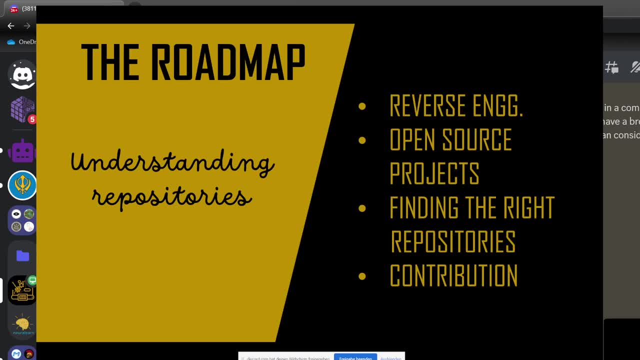 be making separate content on this throughout the next year and how I'd be making separate content on this throughout. you can use existing project to learn on your own and an understand basically how the other people started, because you could take up some simpler repositories that exist on verpe. you could start with seeing 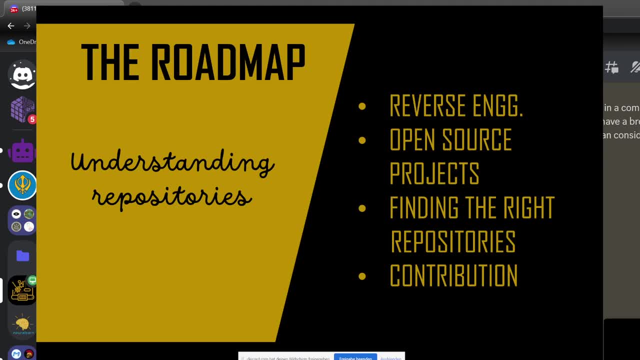 what was there first, commit? how did they start doing it? what are the things that they started updating and then based on just doing that and replicating them? so, basically, I would say that, starting from this guide, in which the other projects 1-2 leads- 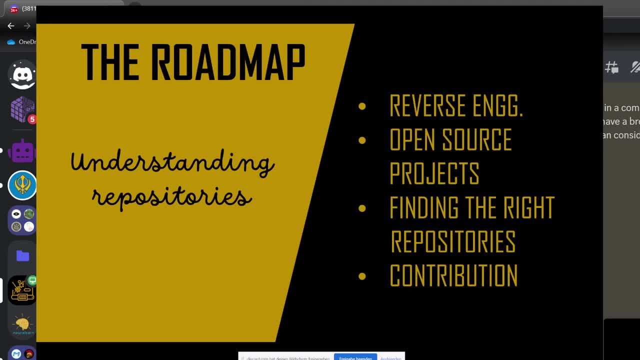 on your own, you'd be able to learn things, and this is kind of similar to the tutorials that you see, and the best way to follow tutorials is if you start doing the projects on your own and then refer to the tutorial only as a solution and then compare it. that would give you most learning. 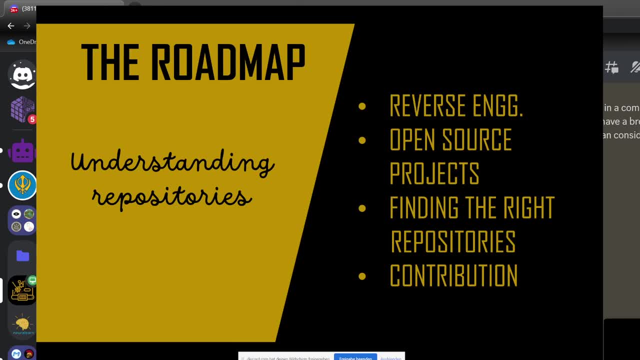 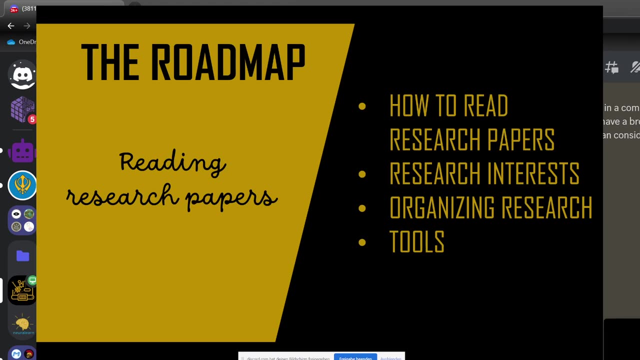 overall and then contributing to open source projects and so on. so this is something you can then focus on end of 2023, once you have already gotten a job and you're now continuing to learn, reading research papers, and then you can explore whether you want to still go into continue in. 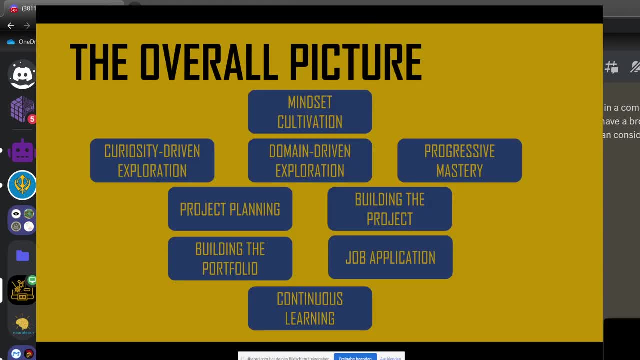 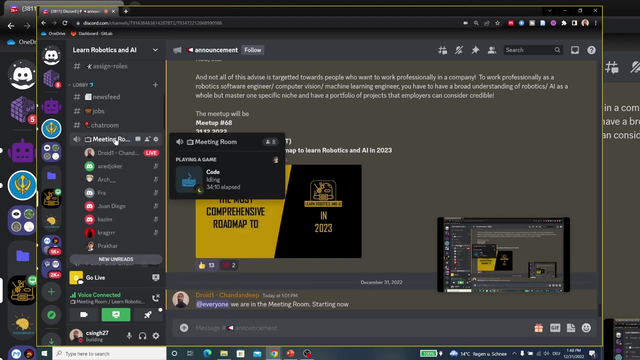 industry, or you want to go in research? yeah, this, this is going to go on forever, okay. so that's a lot already. let's pause a bit and then i'll take the. i'll talk about the plan, systematic weekly plan where i'll connect all of these things together, and then the case study. so any 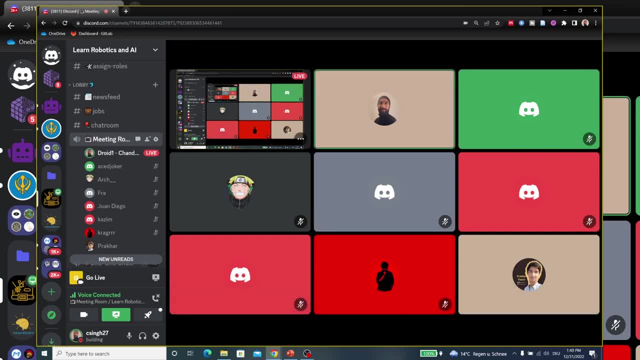 questions. anything is unclear so far, or is everything clear? yes, i guess, um, pretty much everything is clear. it was like, uh, just an overview, i think. yeah, yeah, uh, okay, that's great. thank you so much for joining us today and i'll see you in the next video. bye, bye. 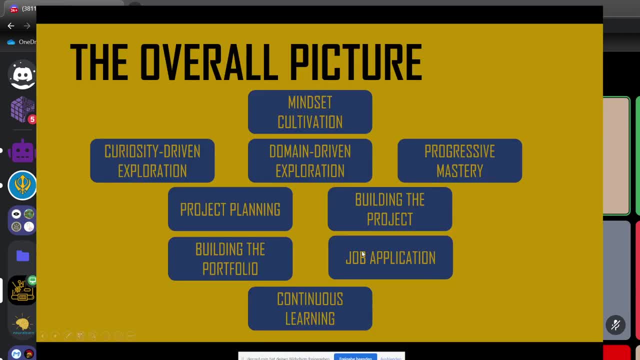 good, so i can just continue. uh, so the overall picture? overall picture looks like this: uh, so first you'd spend just some time cultivating your mindset and then, curiosity driven exploration, domain driven exploration, progressive mastery, planning the projects, building the project, building the portfolio, applying for jobs, and then continuing your learning, learning. 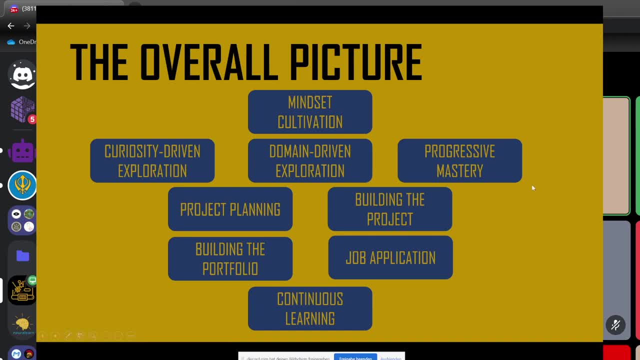 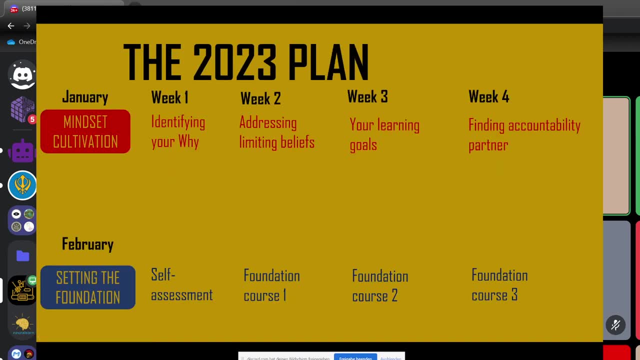 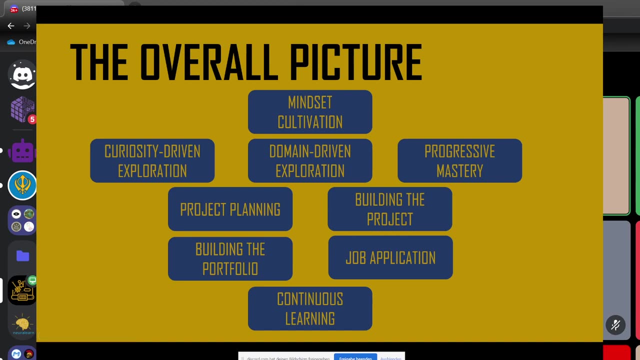 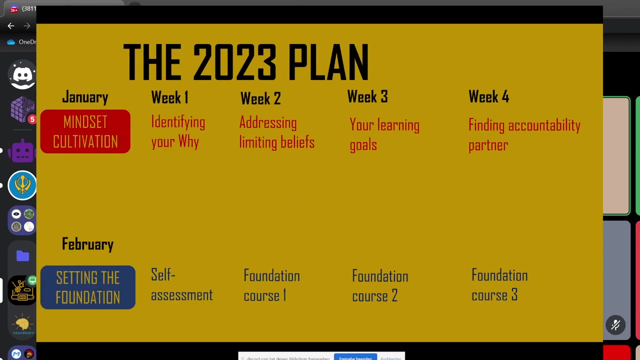 journey, basically. so these would be the overall modules of the- uh, all the modules of the roadmap. so how would you structure this? now, because these this is maybe complicating it further and I want to simplify it and not complicate it further. so the way that I can simplify it is by making a 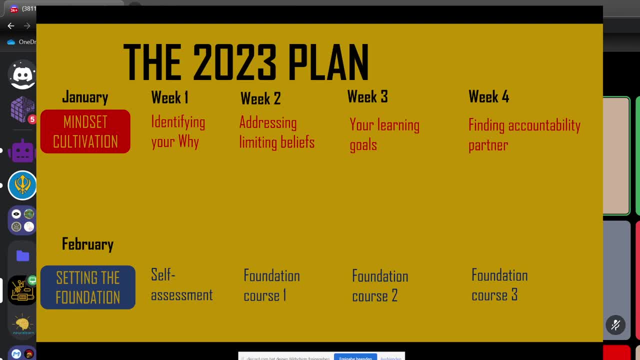 systematic weekly plan for each of these modules. so the first month would be mindset cultivation. one week would be identifying your why, and of course this is just one possibility. you can use this template and then update it, maybe identifying your why. you just need maybe a couple of hours one day and then you. 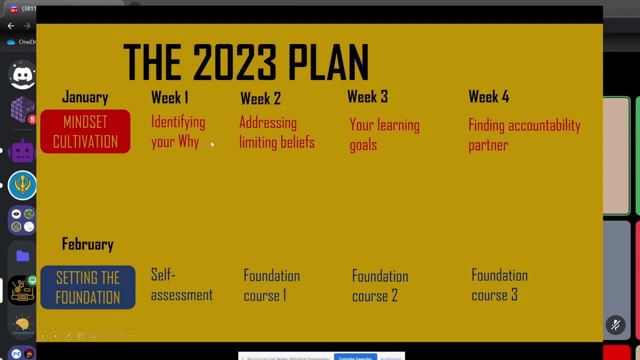 could do this also in the same week and so on. but to keep it realistic and possible, maybe you have other things going on and so you could spend only a few hours a week, and so you would identify or why you would do your activity for this week. you would. 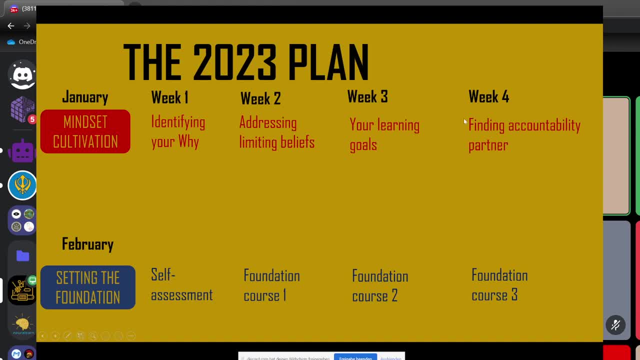 address your limiting beliefs, you would identify your learning goals, you would find an accountability, partners, and these are very small activities that you could just get done, and the first month would be to just cultivate your mindset and then in February, you would be doing a self-assessment. first of all, 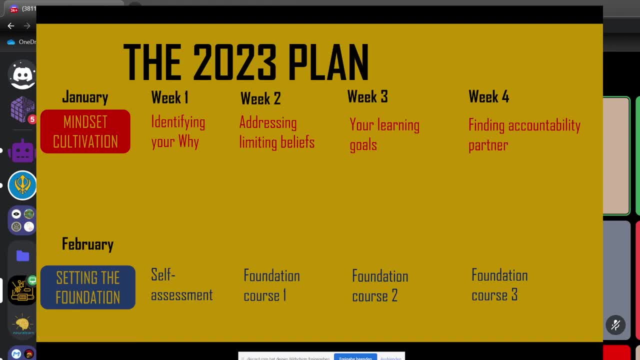 identifying what are the things that you lack. how good are your mathematics skills programming? what are the things that you lack? how good are your mathematics skills programming, what are the tools that you need to learn, and so on. and then you would take certain foundation courses, or these could be projects, these could be udemy. 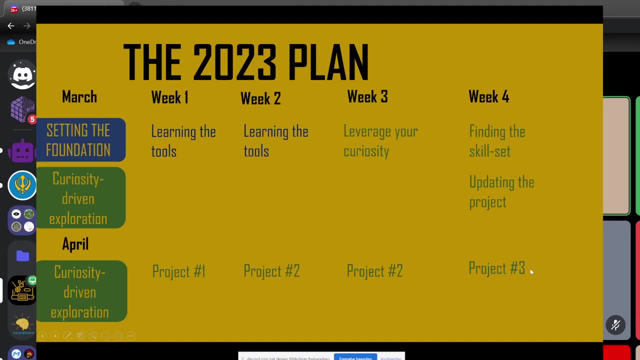 courses- these could be a lot of different things, like tutorials and so on- and just to basically fill in the gaps. and then two more weeks then to build an even stronger foundation by learning necessary tools like git, and I talk about why everyone should learn git before you start doing a project. so 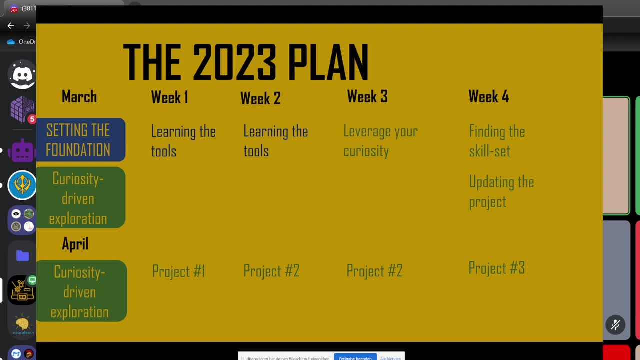 that you, from the very beginning, you are able to learn how it is what it is like to work in the industry, because every company uses git or some other version control system. so, learning this tool, learning a bit of software testing and, if you have an accountability group, maybe also some scrum and managing the 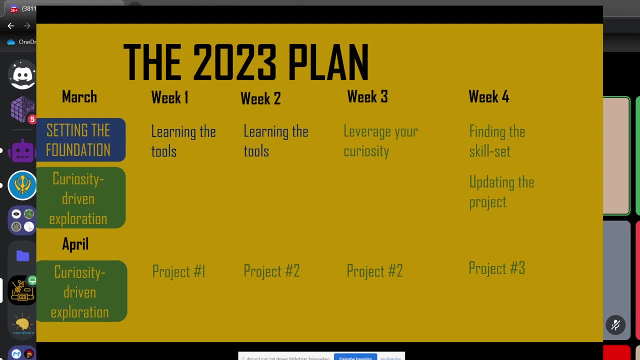 project, so that you meet up on a regular basis and then have tickets or tokens that you update, have issues for their projects and are approaching it in a systematic way. so the whole idea, as i mentioned, is to give you a whole simulated work experience that you could use on your own. 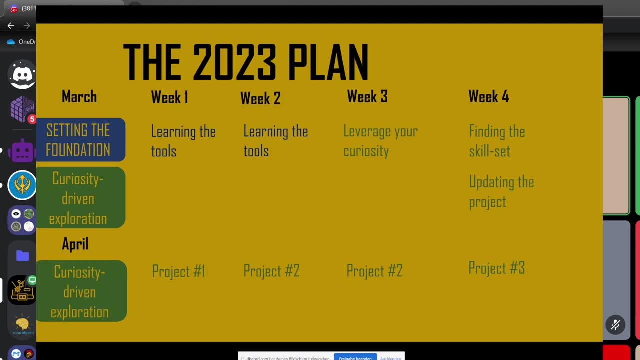 to gain expertise that would make you employable. and then again, just i'll quickly go through the whole plan because most of the things i've already covered now. so you would leverage your curiosity, you do the curiosity driven exercise, you would find the skill set that are that is used in the 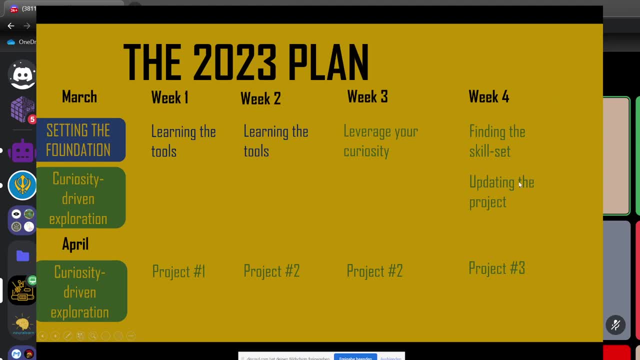 industry. you would update the project list such that you cover the skill set and link it, the projects that you came up with based on your own curiosity. so you would do one small project and then then another project. so this is maybe it's slightly harder- and then you give two weeks and 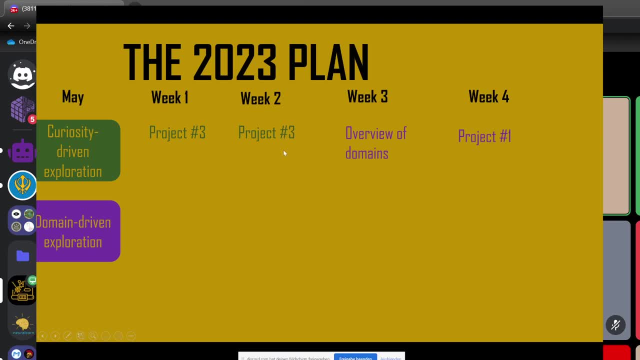 then the other project is slightly, even even more harder than you. would. give it three weeks and then in week three of may you would get an overview of different domains. i think one week is more than enough to get an overview of different applications and so on. this is nothing too. 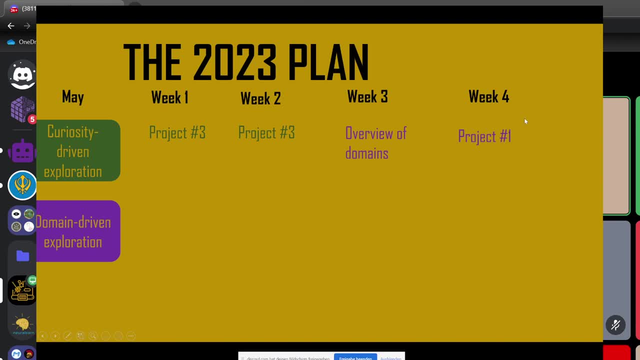 technical here and then after that you would just do one very simple project. so project one and then another small project in a different sub domain ّ, Something that you should consider to get the job done. This is very easy. this comes in all types of demand: software fights. 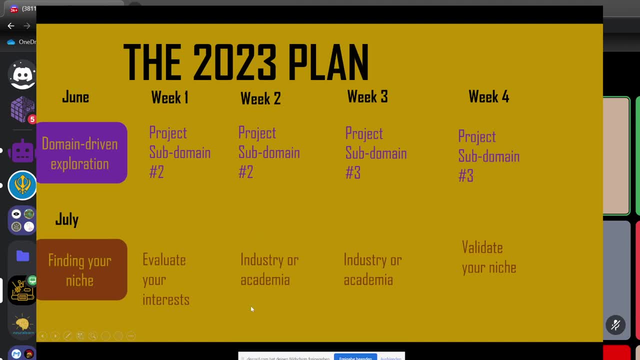 Post a document If you want to make an online cost. and second week of June and then in another two weeks, forfulness. You would be finding your niche, you would be evaluating your interests, you would be spending some time whether you want to go for industrial academia and validating your niche. 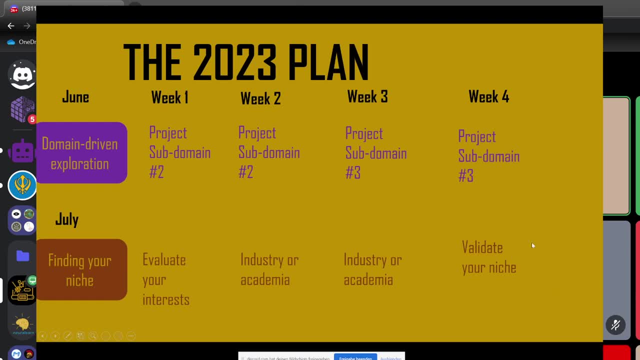 So I've maybe given too much time for this, but I think it is extremely important to be very clear on your niche, because you would be then spending a lot of time working on that, doing lots and lots of different projects. So maybe you don't need 4 weeks, maybe you could take 2 weeks or 3 weeks, but this is one possible way of structuring it. 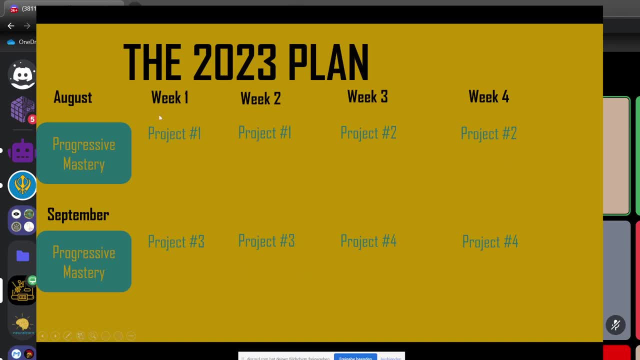 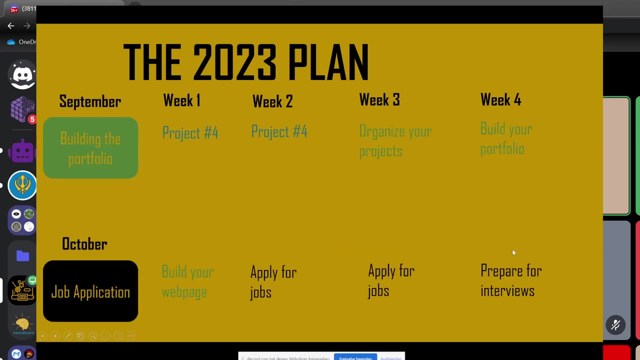 And then after that you would be taking up more and more projects. so one simple project for 2 weeks, and then another simple project and then projects of slightly increasing difficulty. So the last one. I've given 4 weeks for this, so maybe this would be the hardest project to do. 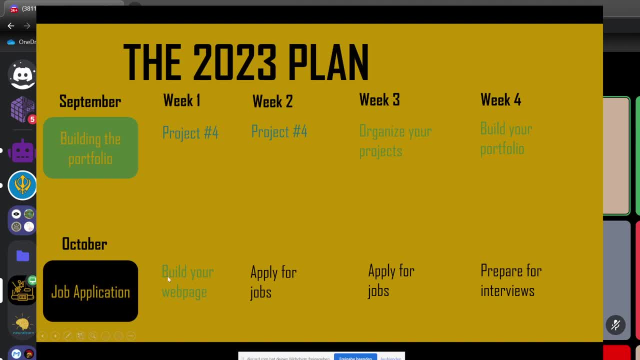 And then after that, you'd organize your projects, build your portfolio webpage, apply for jobs, prepare for internships. So this is so. you see that already mid of September you are able to finish all the projects and then after that, you'd just be applying for jobs, organizing the projects and things like that. 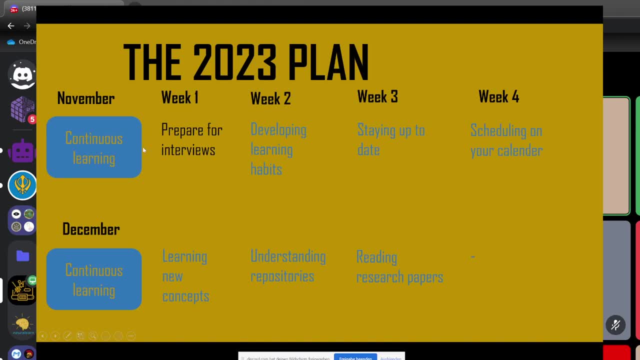 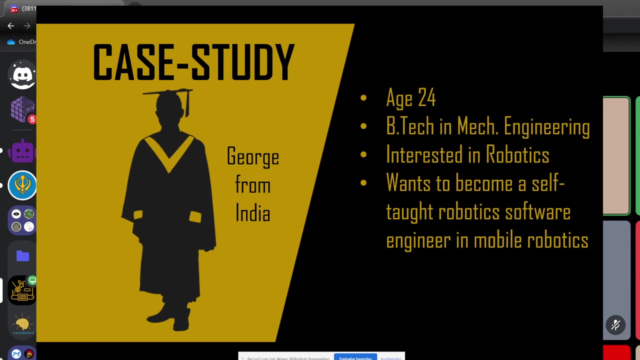 And after that, after preparing for interviews, after you have your job, or even if you don't have your job, you could continue applying and then developing your skills in all of the different ways that I mentioned. Okay, So this is a case study of George from India, who is 24 years old, and this is, of course, a hypothetical person that I have taken. 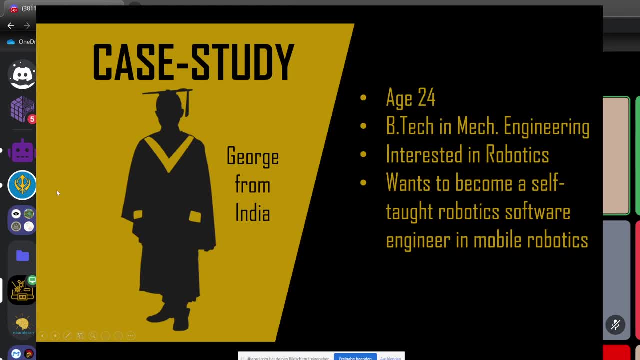 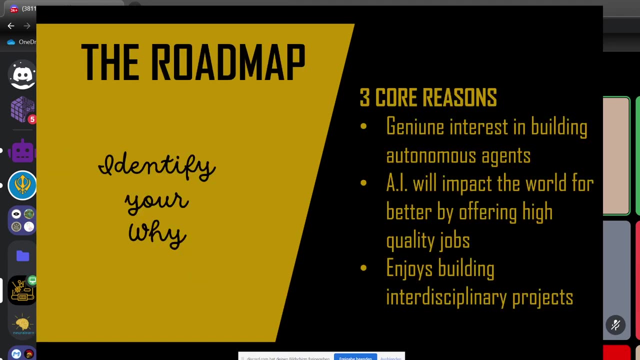 His BTech is, let's say, in mechanical engineering. he's interested in robotics and wants to become a self-taught robotics software engineer in mobile robotics domain. So very hypothetical problem, but maybe you could relate with it. So he would start with mindset cultivation, identifying his why. 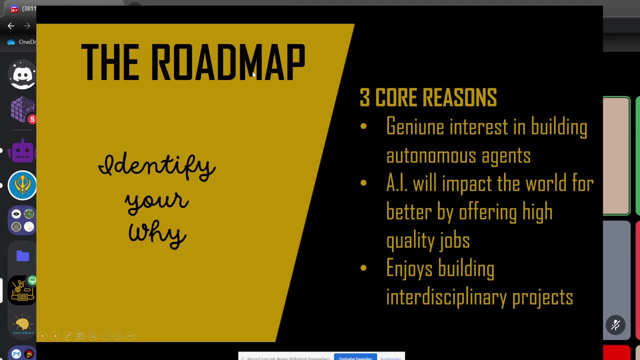 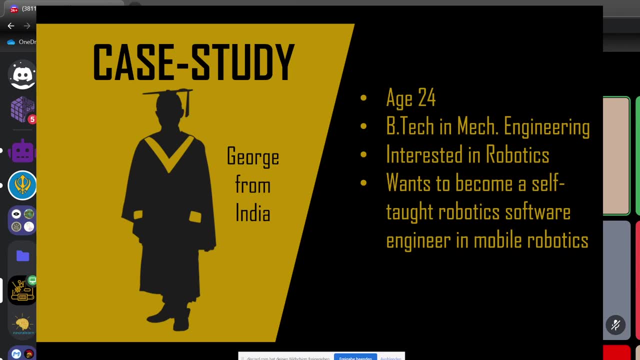 So he would. He'd spend some time and then- I'm sorry to interrupt, but like what's the? basically the mobile robotics. So mobile robots is basically ground wheeled robots and related to the realm of autonomous driving and things like that. 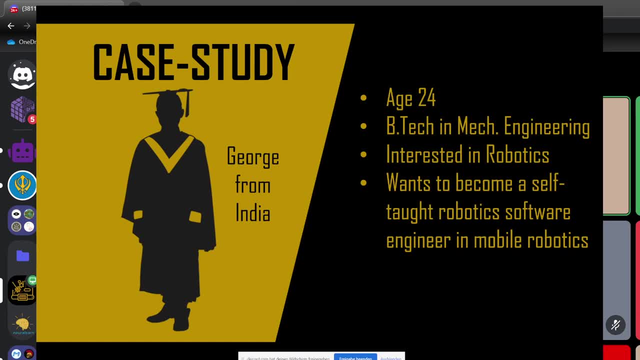 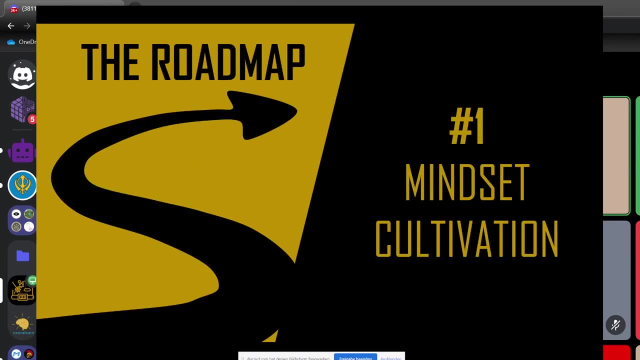 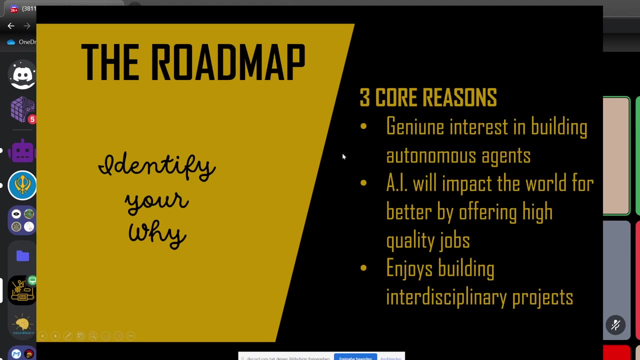 And also, for example, Roomba could be one mobile robot. So in that domain, Yeah, Okay, Thank you, Yeah, No problem. And then he would start with first identifying his why So? and of course, he would be updating this, also based on the activity. 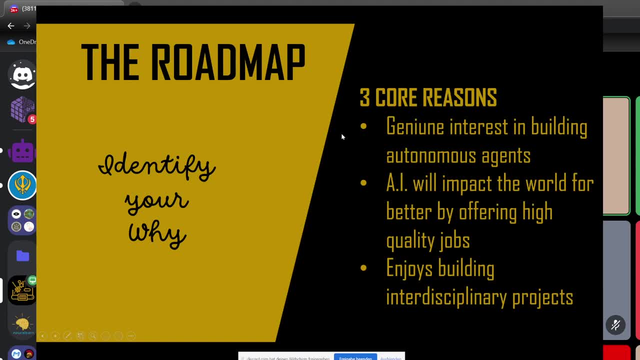 So the final core reasons that this person came up with is that he is genuinely interested in building autonomous agents and he believes that AI will impact the world for better by offering high quality jobs rather than offering more mundane jobs that we have And then would, and also, he enjoys building interdisciplinary projects because he 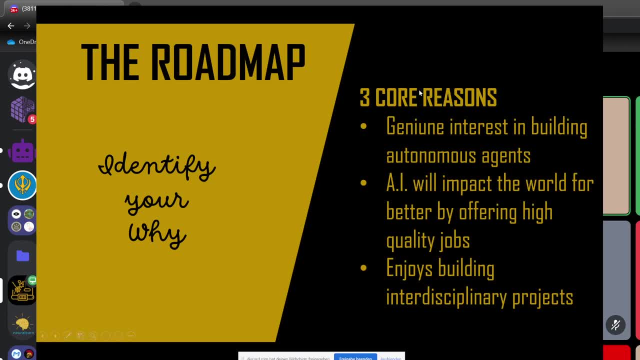 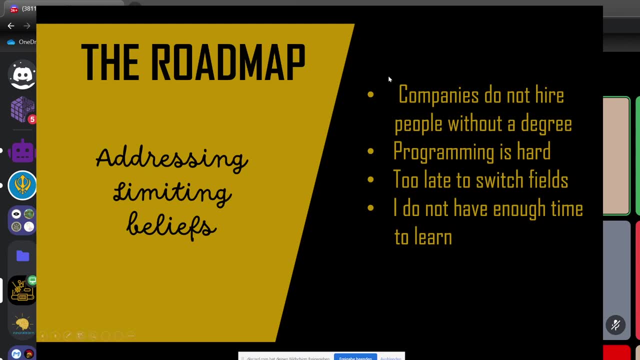 has done that in the past. so these are the core reasons that George has identified for himself, and then he spent some time also identifying his limiting beliefs. he George because he wants to learn robotics on his own. he believes that companies do not hire people without a degree. he would spend some. 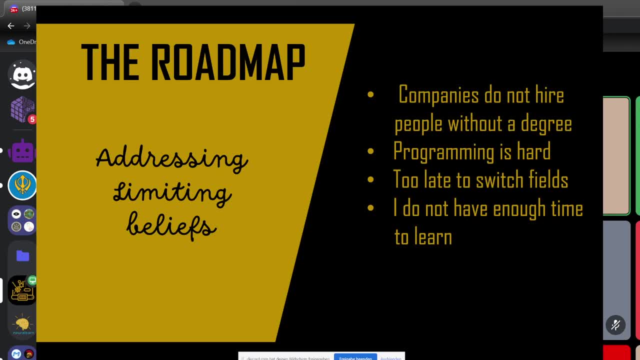 time really questioning it. is it really true? true, because you could find several examples on LinkedIn, on YouTube, everywhere. basically that people are able to get jobs by taking up online courses or learning things on your own and just getting the right opportunity at the right time. so it is not really a. good excuse that you could say that companies do not hire without a degree. it's very much. it's a good possibility that you would be able to get a job without a degree if you have the right skills and the projects and and that programming is hard. this is another. 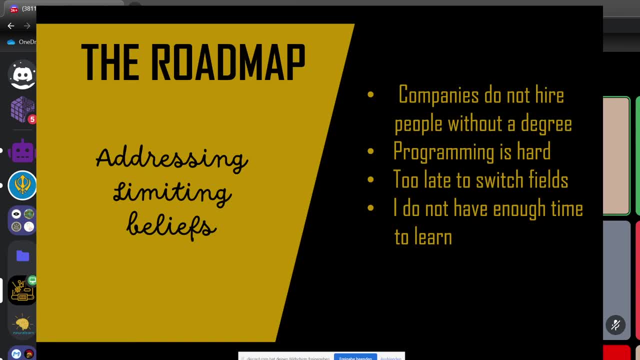 limiting belief. one one common thing that people say is that is it possible to to learn, to become machine learning engineer without learning programming? so this is, of course, not really possible, because if you want to be in machine learning or computer vision that you have to learn programming. so, addressing 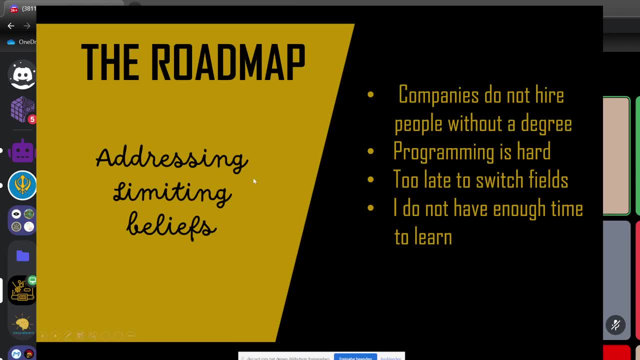 these kinds of ideas and just failures in mindset that you should address early on. so it one problem could be that. so George is 24 years old and he thinks maybe it's too late to switch fields- now he's in mechanical engineering, and this is also one of the common limiting belief- and that he does not have enough. 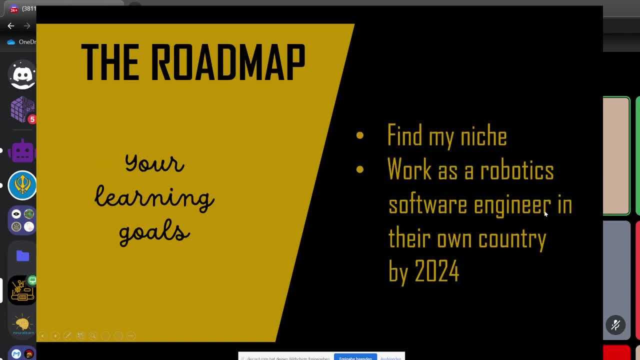 time to learn, because he's currently also studying full-time. so then, George identifies his goals. these are just a few things that you can do for yourself when you're working in your career. So he has two specific goals. He wants to identify his niche. 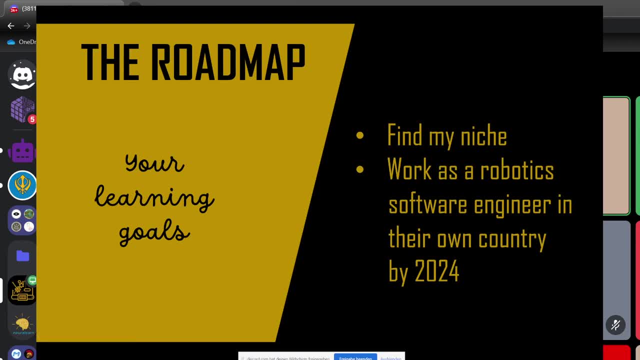 He thinks that he wants to learn mobile robots, but he's not absolutely sure. So he wants to be specifically sure about his niche and he wants to work as a robotics software engineer in his own country by 2024.. So this is his goal that he sets. 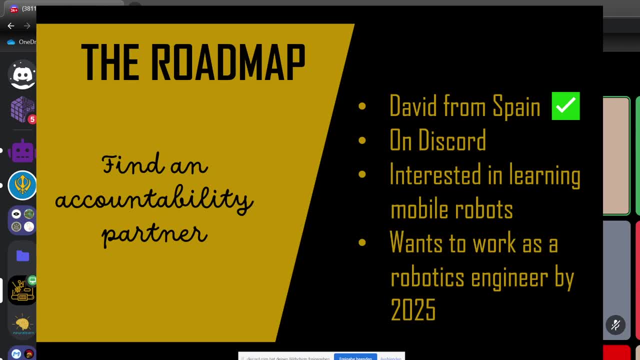 And then he finds an accountability partner on Discord- Again totally random David from Spain. And then he sees that David is also interested in learning mobile robots and wants to work as a robotics engineer by 2025. And so they could start learning on their own. 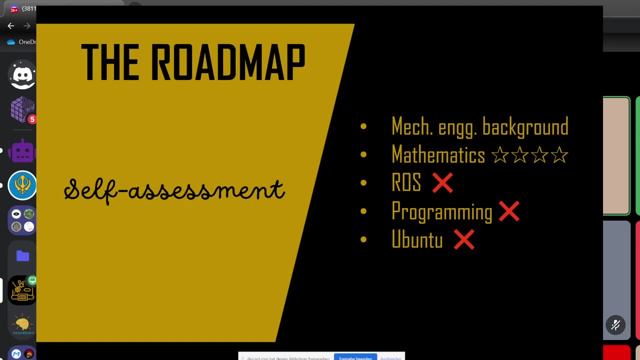 So George does some self-assessment. He realizes that because he's already enrolled in a university, his mathematics is pretty strong. He says that he is four out of five in mathematics and probably doesn't need much of a job to be able to do that. 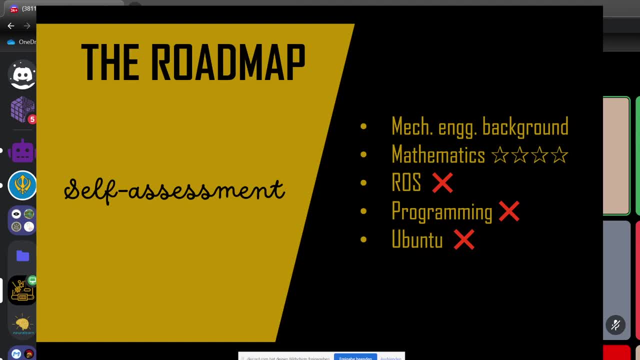 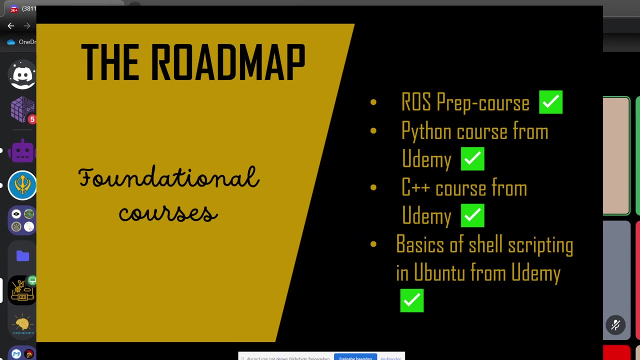 He doesn't have much mathematical foundation, but he doesn't know any ROS. He has never worked with Ubuntu and he has zero programming skills. He's currently studying mechanical engineering, so has a mechanical engineering background, So foundational courses could look like taking a Python course from Udemy. 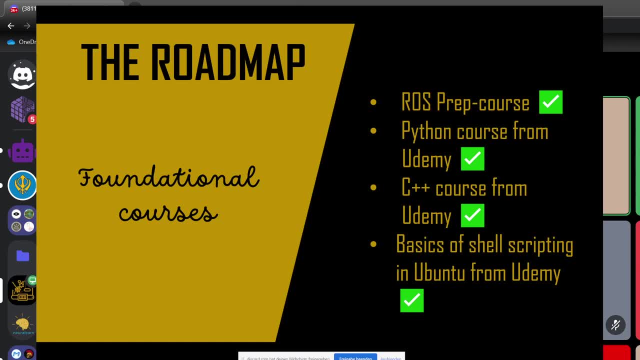 taking a ROS prep course and you all know there's so many resources and you could just take one good resource to just fill in the gaps in knowledge, So getting familiar with Ubuntu and other Udemy. so here I've taken Udemy as an example in all the cases. 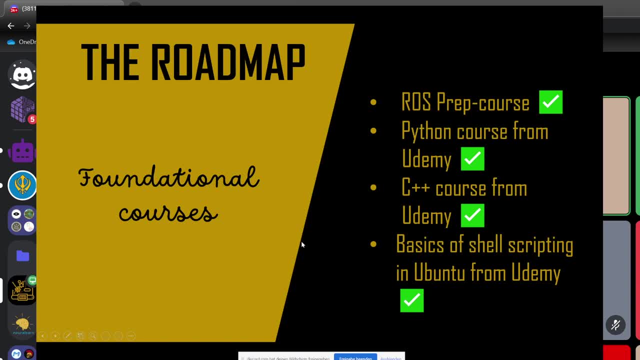 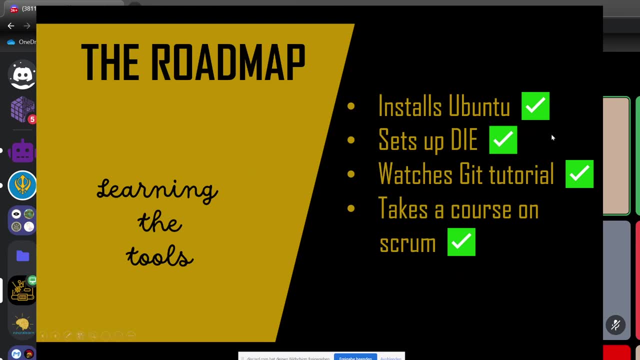 but it doesn't really matter, So this is for this particular hypothetical case study that I've taken. So then George goes about learning the tools. He installs Ubuntu, sets up IDE- not D-I-E, Sorry again- And he watches some Git tutorial. 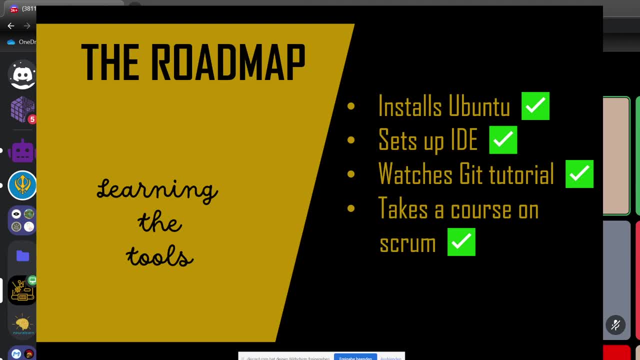 and in a couple of hours he's able to learn the basic tools that are required for Git. He takes a course on Scrum because he's working with David, his accountability partner, as well, So he would need some sort of system. Then he starts building the projects. 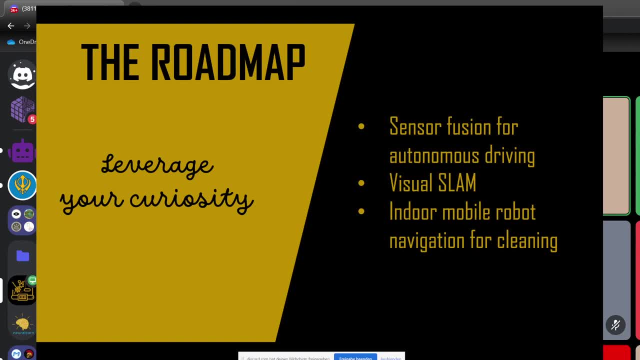 So he does the curiosity exercise and he is really curious about Visual SLAM sensor fusion for autonomous driving and indoor mobile robot navigation for cleaning. So these are just things that he came up with. So the activity looked like. he came up with 50 different projects. 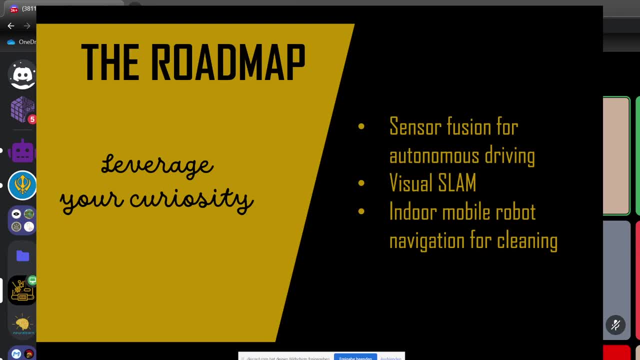 or 20 to 30 different projects, And then he started filtering based on his interests and the ones that are practical to do. So these are the projects that he chose based on the comprehensive activity that he did He identified. he looked for companies online. 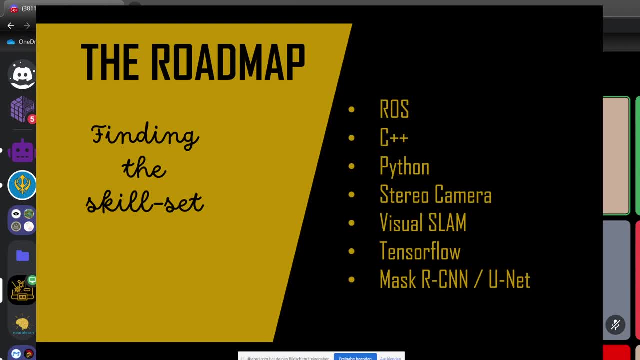 He identified the different jobs that are there, different job openings that are there, and he saw that ROS is required almost Everywhere. for similar kinds of projects that he came up with, C++ is required And also Python stereo camera. working with stereo camera was a requirement. 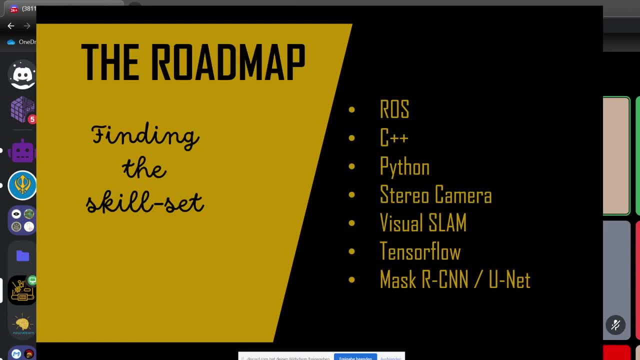 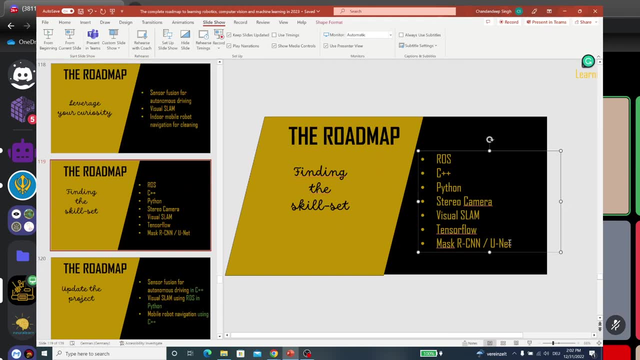 for navigation: Visual SLAM, TensorFlow, MaskR, CNN or Unite. Actually, I had more projects and I removed those, So I think let's keep it simple And for this particular case, since these are all sort of mobile robots, 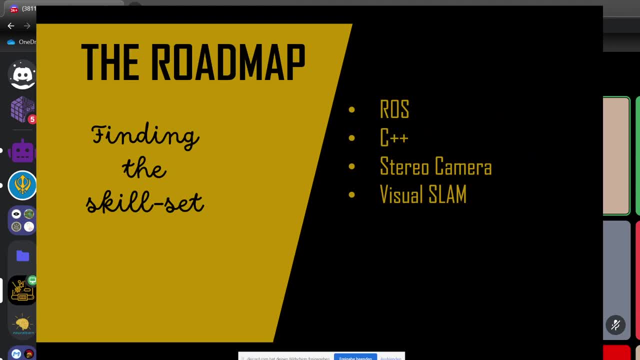 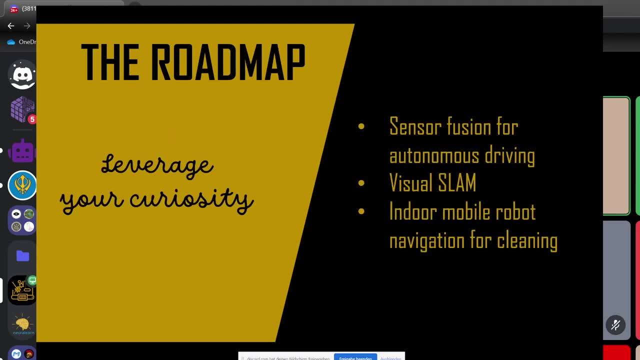 and navigation projects. so he identified that C++ is more important than Python. This is what the companies use, And then he updates it. So previously he had no idea which programming language to use, which tools to use, but he updates it now that he'd use. 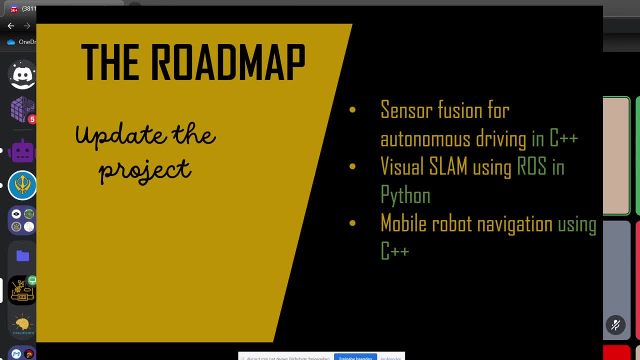 he'd do the same projects but he would use ROS and C++ and he would stick with that, because those those are the ones that are used in the industry. And he updated his project list and he does the project. He does the project by structuring it into several activities. 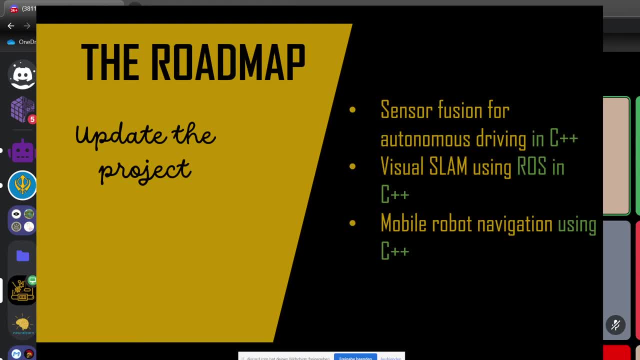 I've not covered it in this session today, but you could watch the previous meetup session or some of my recent videos where I talk about how to plan your robotics or CV or ML projects, And there I've talked about breaking down projects into simpler activities and learning the concepts. 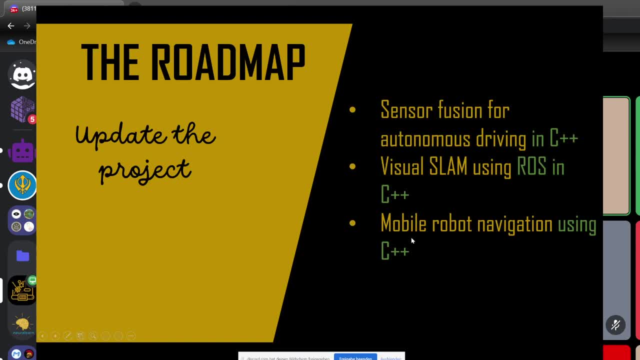 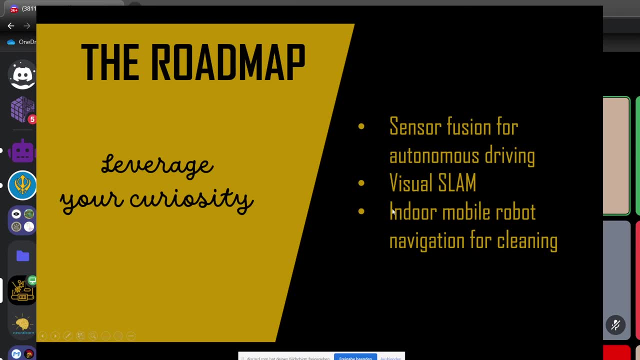 along the way. So this would take more time to cover, So I've not covered it here. Then he sees: okay, I'm interested in this, but this is very limited. This is based on a very limited knowledge of his. He doesn't know different other domains in robotics. 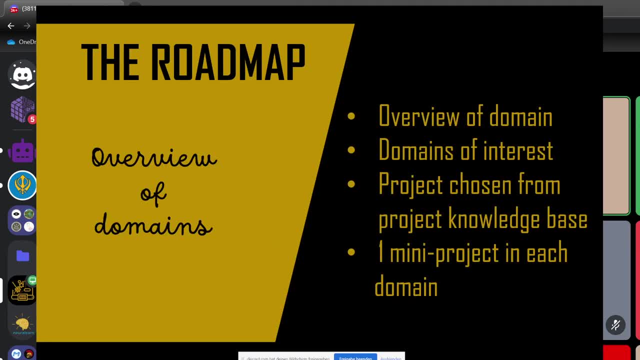 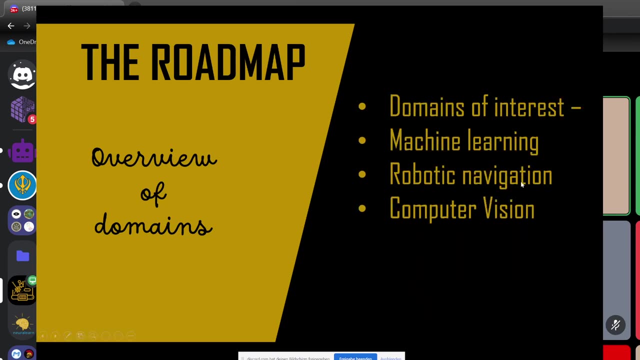 He doesn't know, he hasn't tried machine learning and so on. So he wants to try other specific domains and he would choose three specific domains and one mini project, one simple mini project in this. So he sees that there are three specific subdomains. 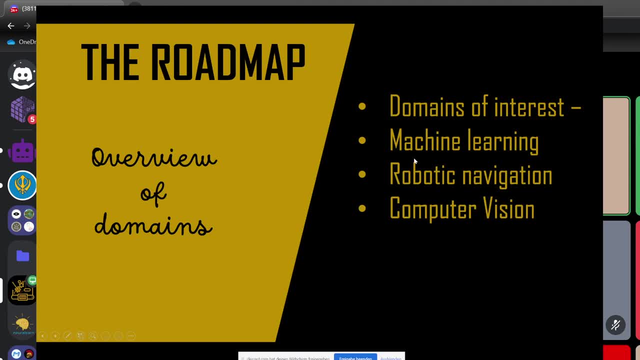 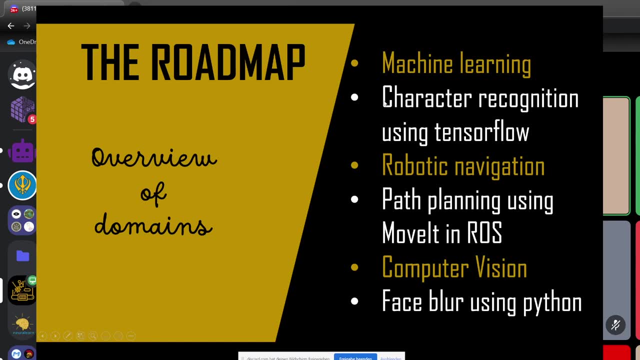 that he would be interested in machine learning, computer vision and robotic navigation, based on also his curiosity. So he takes up one simple project in each of these. So character recognition using tensorflow, path planning using move it and Ross- very simple projects- face blur using python. 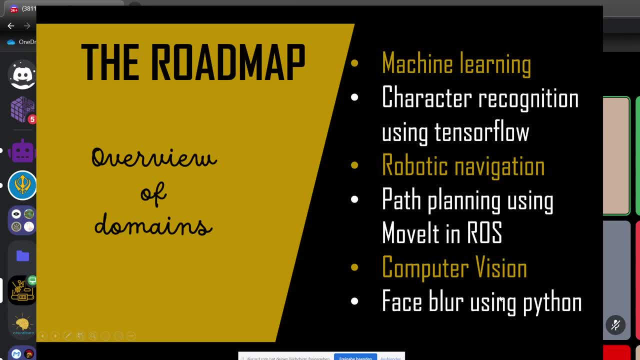 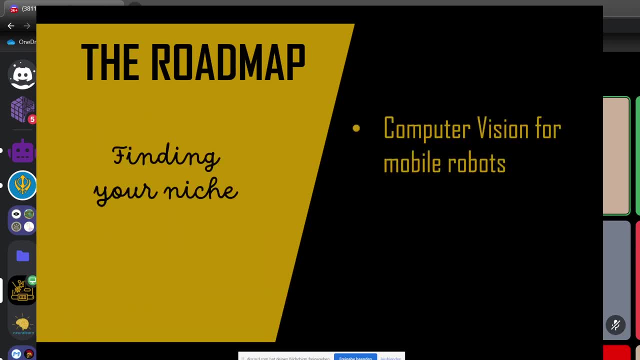 So all of these things he chose to do. So three more projects. So in total now he has six projects, and then he would spend time identifying his niche. He did the activity and I make separate, separate videos for the activities, or or an entire course, depending on if it is really something that is required. 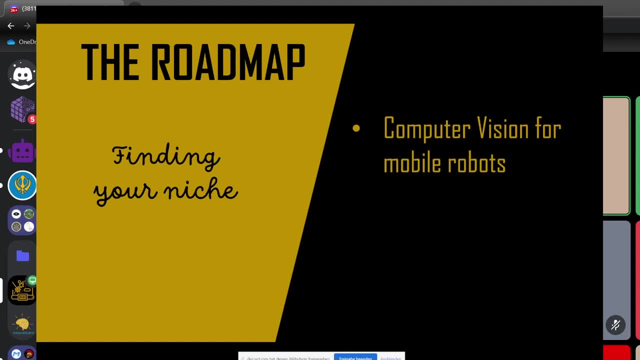 and I will talk about this later. So he identified his niche based on several projects that he did and the activities that he did, that he wants to work for computer vision, for mobile Robots, because mobile robots is something he's interested in, but based on the exploration. 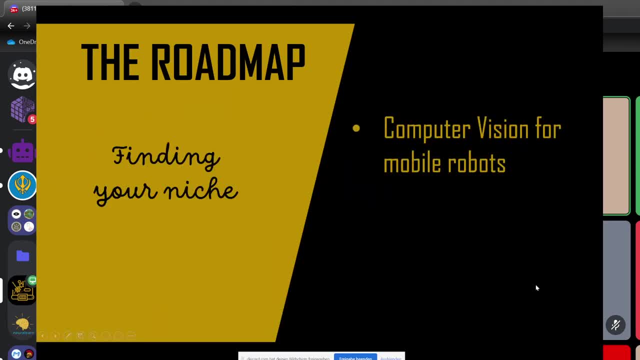 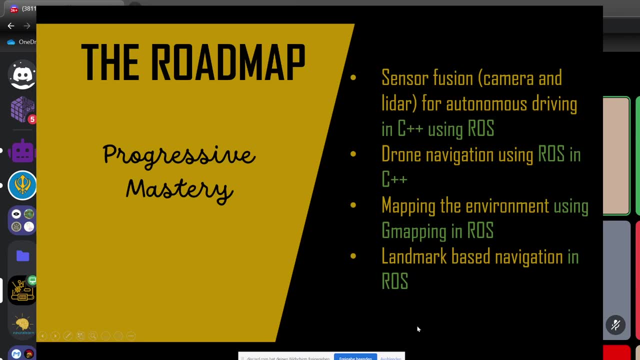 He also decided that computer vision is something he wants to learn as well. So then he would be. he'd be taking up progressively increasing more difficult projects, basically So sensor fusion for autonomous driving and C++ and Ross drone navigation, mapping the environment. So just just, I've just randomly put these projects before. 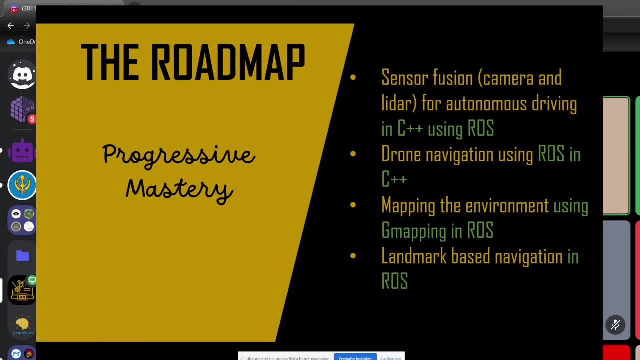 For today's session, but the idea is he, so I would also maybe prepare a list of projects of increasing difficulty or link up some resources, Like I have made one video on the top five YouTube channels that you could use to find computer vision projects. 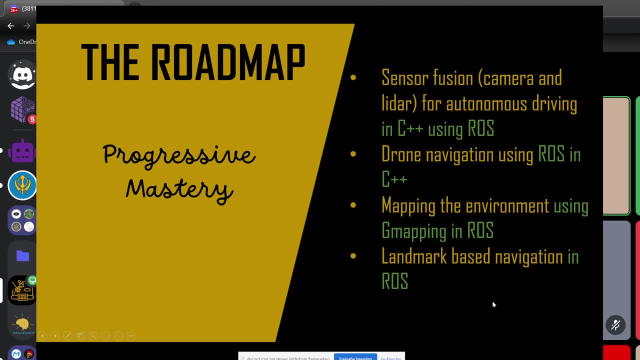 So something like that, and you could use this to find and decide for yourself What are the projects that you would do and, as you can see, all these projects are now in similar directions with C++ and Ross, computer Revision, stuff like that. Then he would build a portfolio of projects. 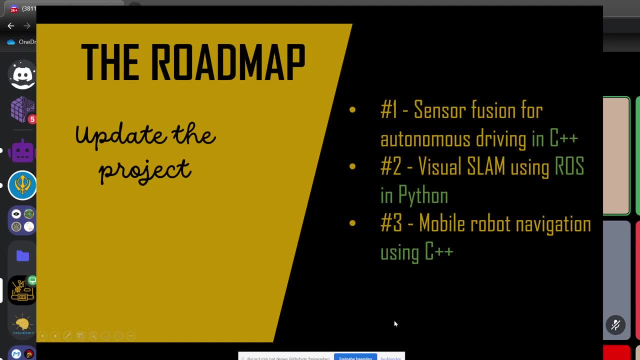 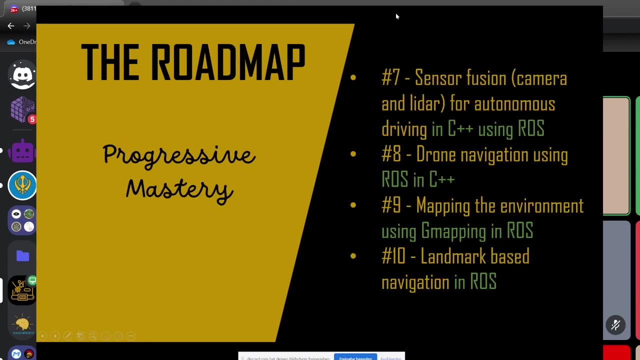 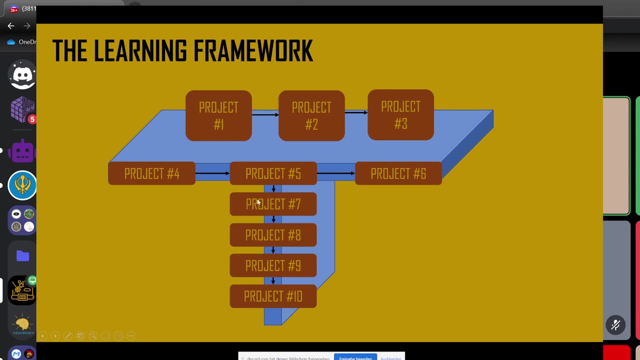 So he has these three projects that he came up with based on his curiosity. He has these three more projects based on domain exploration and four more projects based on progressive mastery. So at the end of this whole roadmap, the whole thing, he has a portfolio of 10 specific projects. 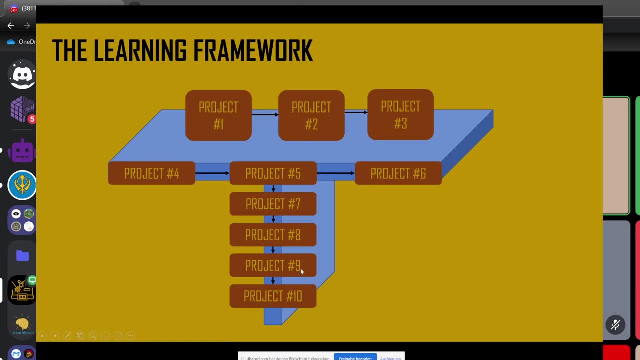 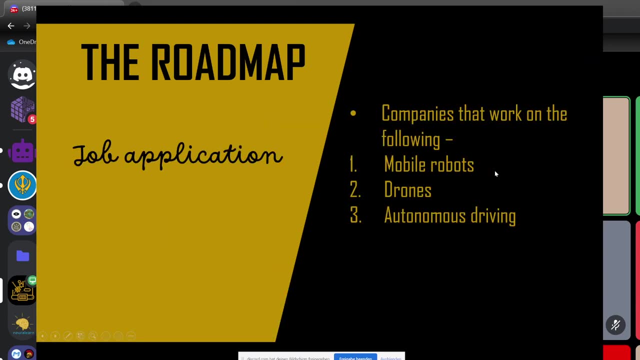 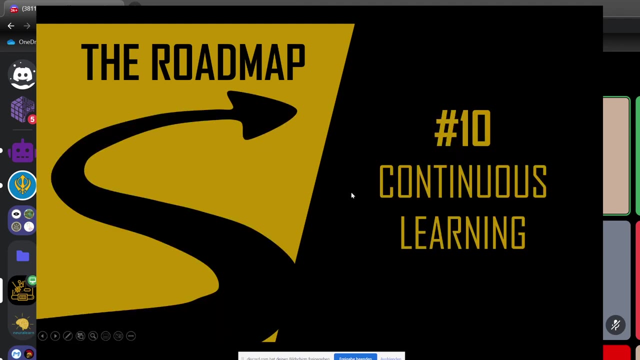 Of course, the six projects would be slightly smaller and these would be more advanced projects, but that is how it should be. Then. he applies for jobs: companies that works on mobile, that work with mobile robots, drones, autonomous driving. continues to learn, follows recent developments, reads research papers, builds projects and explores other domains. 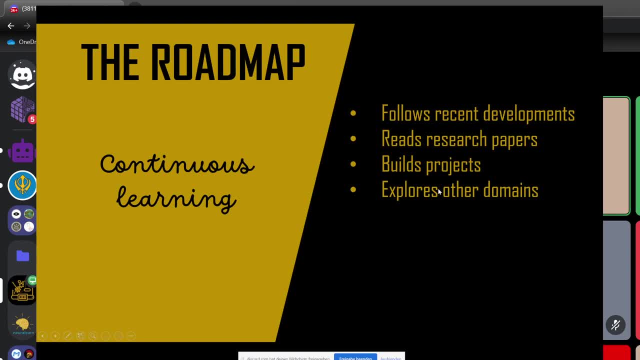 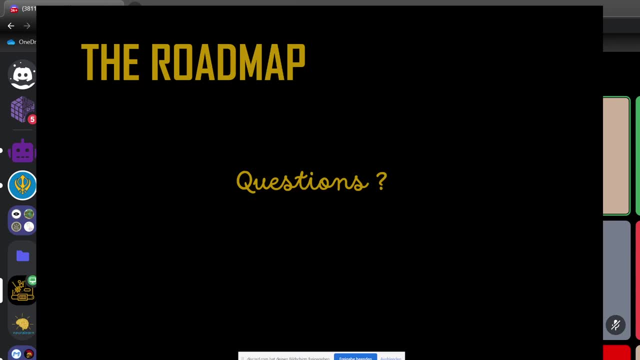 And that is how George would be able to learn and become a professional from an absolute beginner. So that is about the roadmap. Now I'm very curious to address any specific questions. or does it make sense, or not at all, because I have no idea if this was useful or not. 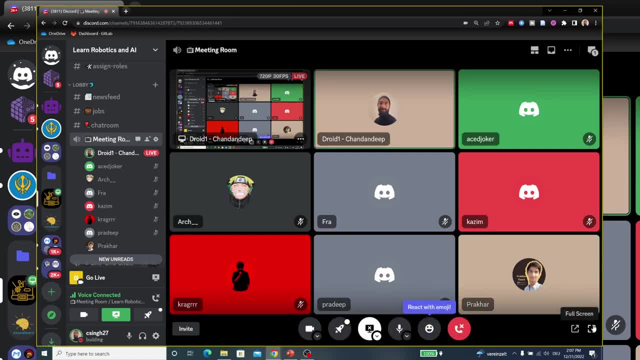 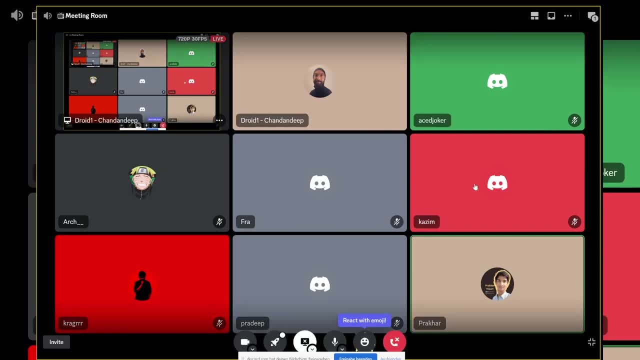 This is just totally coming from my own head, All right. So let's hear from you one by one. By the way, where will we get the presentation PDF, Can we? Yeah, I'll share the presentation. Yeah, So overall, 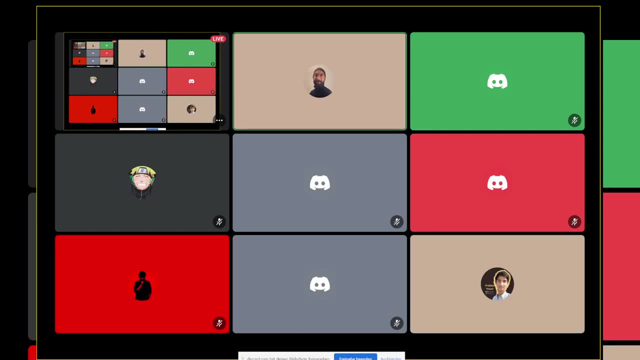 first of all, any questions regarding it. I think it was pretty straightforward the whole thing, But if you have any questions regarding this, I will be making projects using any like I have heard About Arduino and Raspberry Pi. What will be the process of building a project like that? 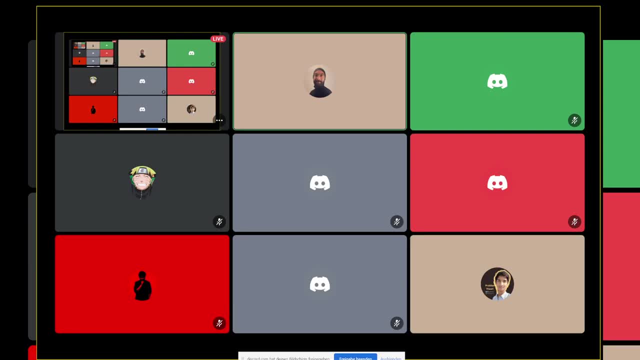 Yeah, So that's a good question. So so, two things. So, of course, one thing is that the projects that you define would be would be based on your own interests and things like that. And, of course, Raspberry Pi is a good option that you could consider and you would maybe not come out, come up with a Raspberry Pi project on your own. 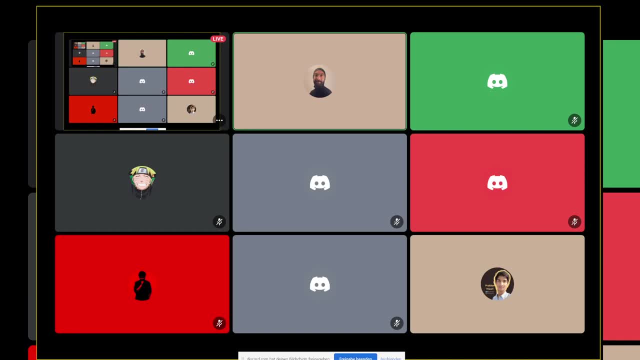 But you would come up with a project based on domain exploration, computer vision project and so on, And so this is one thing, And the other thing is that Arduino is. I would not recommend spending too much time learning Arduino, because Arduino is more for hobby projects. 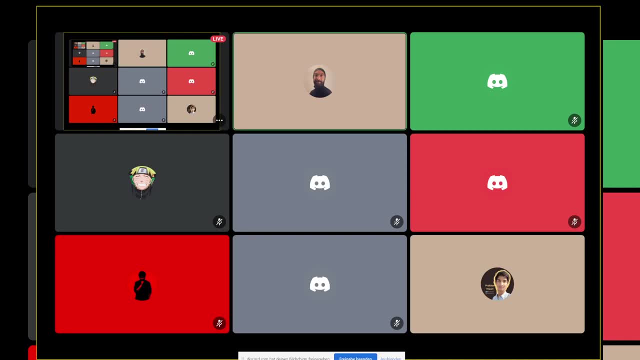 right, And of course I did a little bit of Arduino also when I was doing my bachelor's in India. but that is literally of no use. That is just for like hobby projects of home automation or small robotics projects that you would want to build and it would be a good project for school students, or if you want to just see if build some like simple projects in robotics. 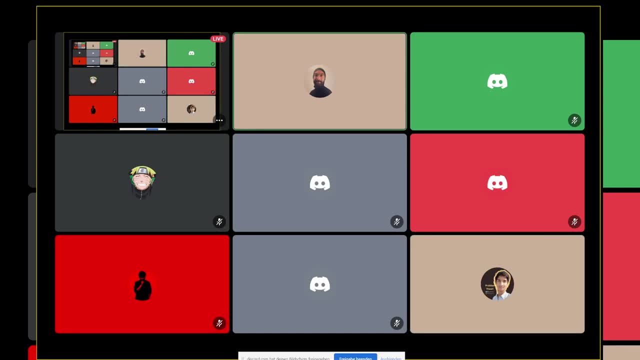 but Raspberry Pi, of course you could do that, and you don't even need to work on Raspberry Pi or or Arduino for this. You could just Focus on, you could just build, you could just use computer vision projects directly on your system, because most of the projects that you would be building based on this framework would be simpler and there's this possibility, of course, to take up Raspberry Pi based projects. 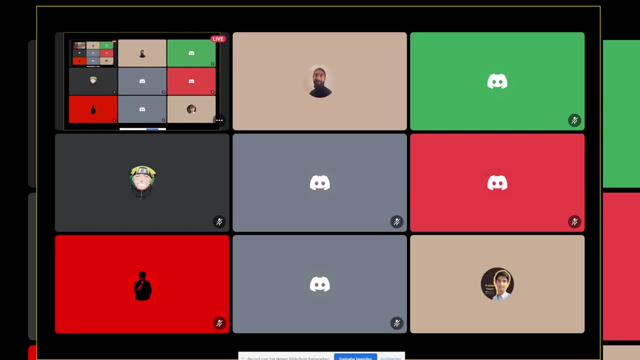 but that would be entirely up to you. Okay, thanks for sharing about it. Have you worked in any startup Related to robotics? Yeah, worked in a few startups related to robotics. I want to know what's the like, what's the environment there and how they work together because, like, I have no idea about how robotics engineer and what would be developing and how they're developing the product and what's like going on in the whole team. 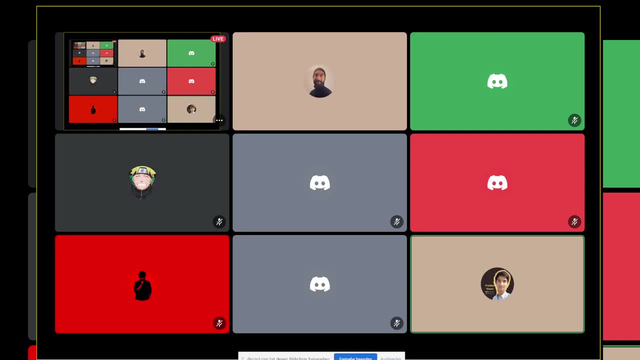 What the overview? can you give an idea of what's? because I'm interested in maybe in doing, or at least working in, a Startup in this field, basically? so I want to know, like, how the whole system works there. Yeah, so so be the startup. of course, robotics is interdisciplinary and there are different fields that are going on that are that would be there in a start up. 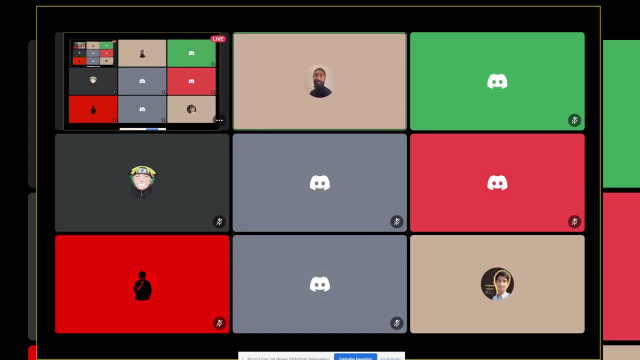 So there will be a mechanical mechanical team, mechanical engineering team, that would be specifically responsible for production related activities, so if it's a robotic manipulator arm deploying that in the industry, in the plant, in the factory and so on, and then there would be one mechanical design team. so, like several aspects of mechanical 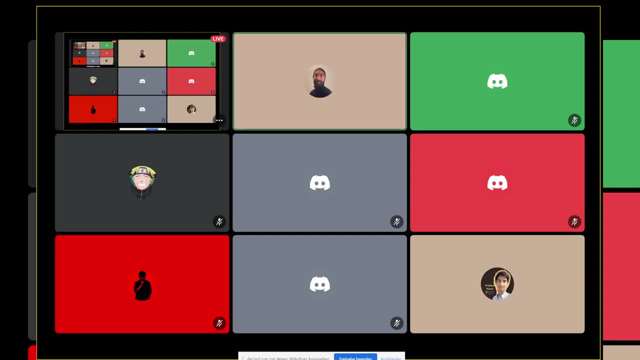 there can be smaller teams depending on the size of the company. so one would be the mechanical team, one would be the electronics team and one would be the computer science or, let's say, the general software team, and within that there could be an AI team. so let's just for simplicity, let's 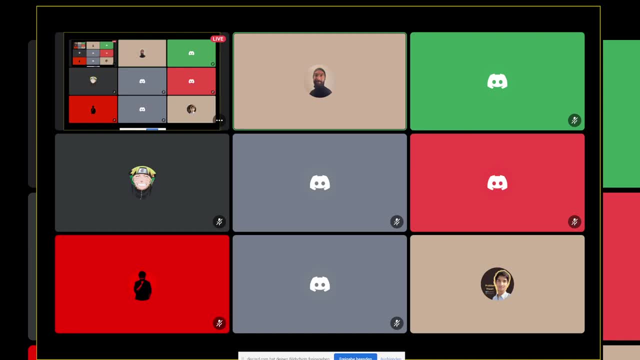 just focus on four specific teams. so let's keep it on general software development, mechanical electronics and then AI, specific software development, right? so it depends on the product. so the startups that I worked in, they were both robotic manipulation based, so they were using robot manipulator arms for solving problems in the industry. so one was pick and place and one. 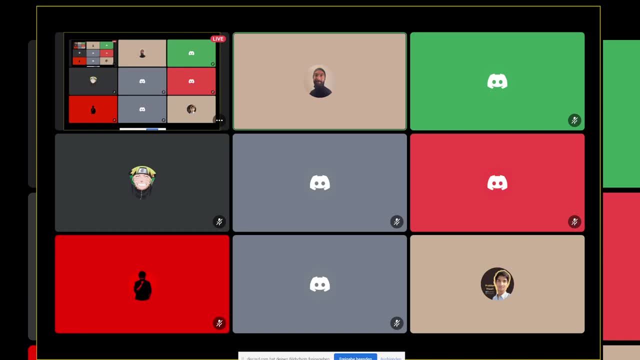 was manipulation of deformable objects right and so. so, for example, the mechanical team- and there could be application engineer also in mechanical team- that would be responsible for making sure that the robotic system is deployed properly and that the cameras and things like that- the hardware side of things- is functioning properly, and then the electronics is responsible for making 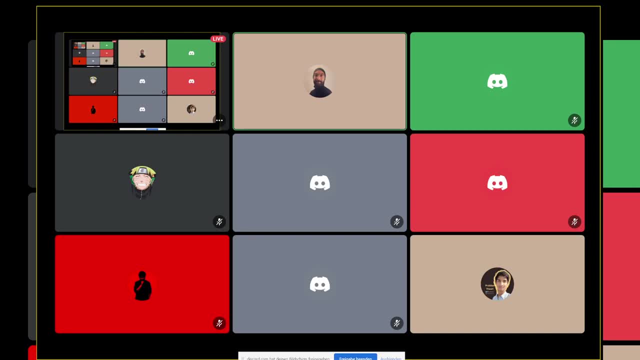 sure the controllers and processors and stuff like that works well and then the software team is responsible for making maybe the web interface and so on, things like that, and then the AI part is specifically so. one specific case is if it is robotic manipulation for bin picking, then the 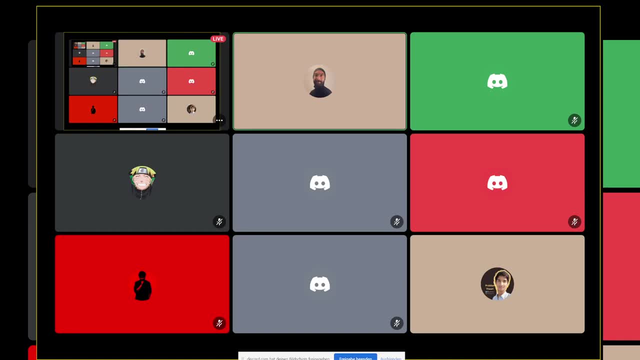 software would be the AI person, who would be responsible for making sure that the software is working in the right way, and then the AI person would be focusing on making a deep learning pipeline and integrating it with the robotic system. so that's why you would be working closely. 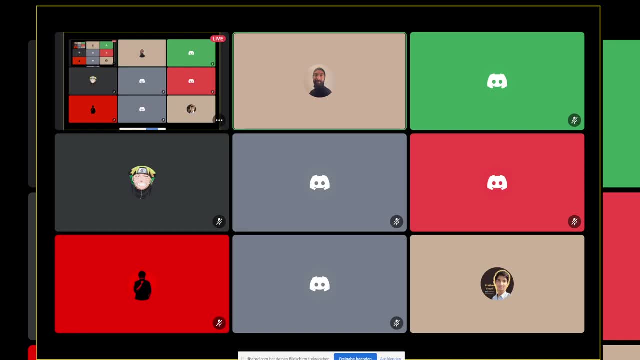 with all the different, all different types of teams. so, if you're working in AI, but if you're working in deep learning, and you have to, of course, also deal closely with the robotic, the mechanical side of robotic manipulation and making sure that the system that you develop is. 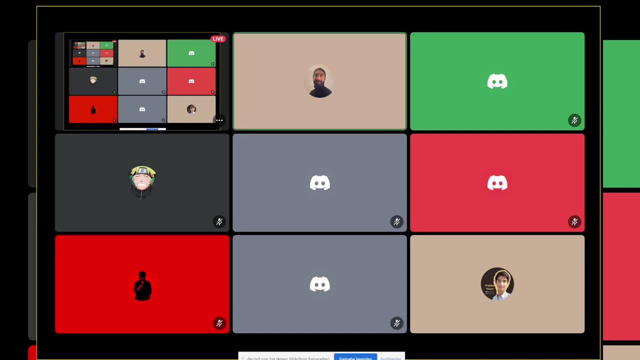 actually deployable. so you would have to make the system such that deployment is taken into consideration and also integration in the actual system, and you would be wanting your algorithm to be integrated in the existing software framework that is being used. so that is why it is important. 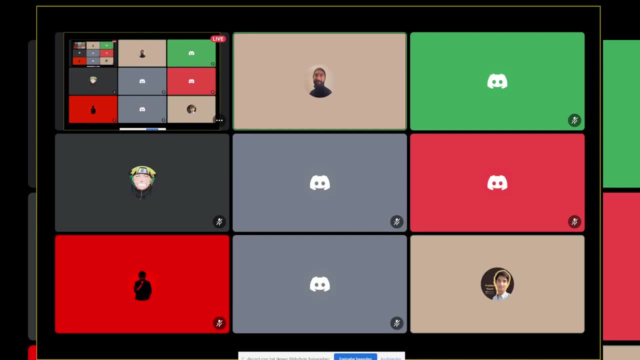 to make sure you have a basic, broad understanding of all the different areas and, of course, your primary focus would then be on deep learning, for example. yeah, basically the t-shaped, learning, the t-shaped exactly. and in startups, the good part is you can get to be more involved because 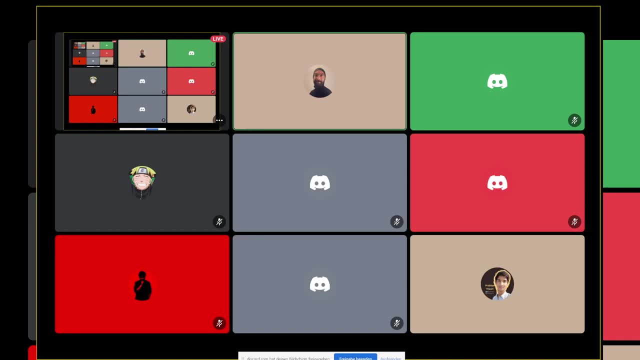 the teams are more small. so even if you're working in deep learning, you will get a lot of understanding of robotics and hardware in electronics and software development in general as well, because maybe sometimes you would want to do things in other domains as well, because there are 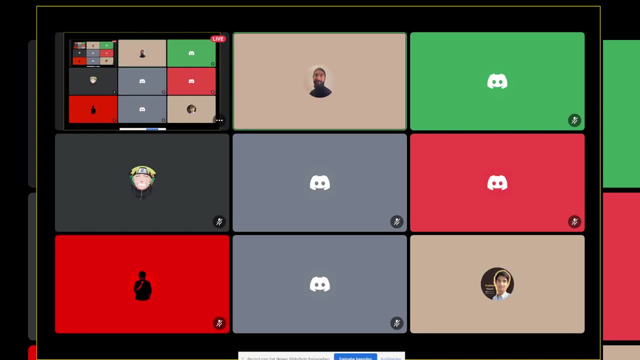 a lot of a lot of people. so it's it, this this way. it's very interdisciplinary to work in a robotic startup. so, yeah, startups generally, generally also prefer that if you have some interdisciplinary knowledge there, yeah, that makes sense and what's the like? I think there'll be more advanced technologies used in the 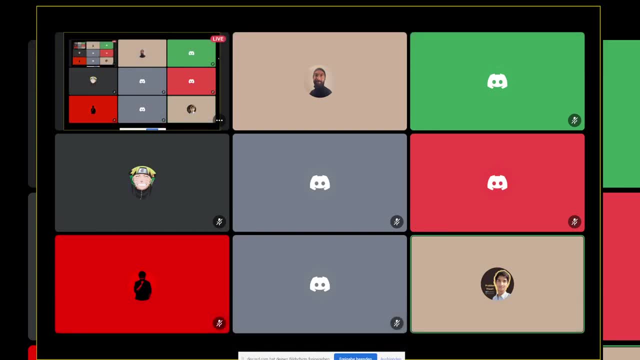 defense companies. we're making robotics, stuff in the defense field, like any aerospace, like flying things- I don't know how to term define it- like drones- yeah, drones and many other stuff. it's like the things are pretty much the same, or are there any advanced studies? so what's your question specifically? 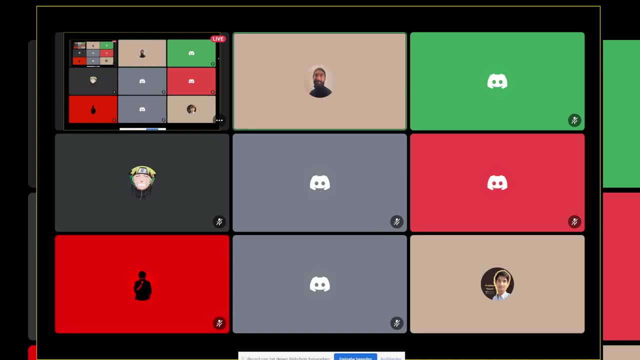 like: what are the things that are used in defense? yeah, I mean, I have not worked in defense so I can't specifically tell that- but of course drones are being used and then mobile robots are something that are used everywhere. so I would say mobile robots and drones and basically it depends, and it depends whether it's a research project or 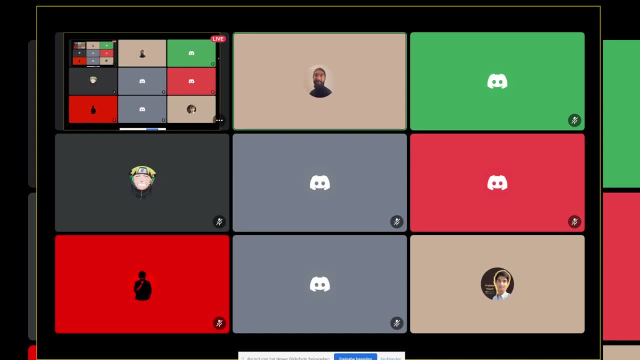 it's actually going to be deployable, so it depends on a lot of things. but drones is something that is being used a lot in defense and, of course, I think mobile robots are also major and it could also be, depending on the use case, mobile manipulation platform. so mobile robot with 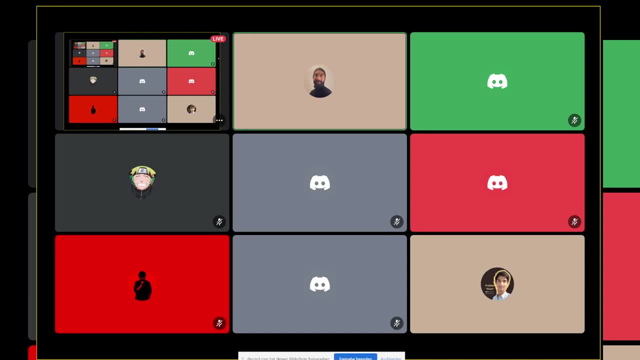 also manipulator arm attached on it, but I yeah, I think you would be able to find it on the official websites of the different defense organizations, so I would recommend you search that. okay, thanks for sharing. yeah, uh, yeah. so any questions regarding the framework or any like you could share, just also thoughts and criticisms about this overall structure does 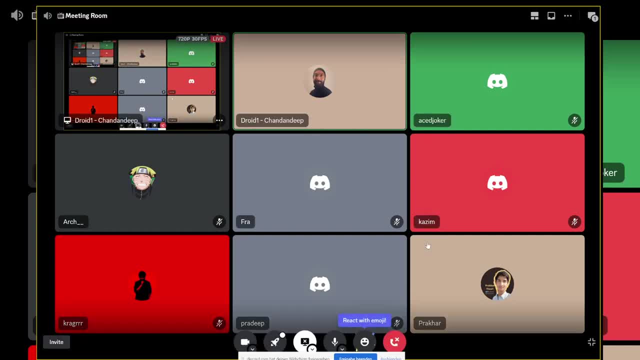 it make sense or not, and uh, yeah, I'm curious to know. so, Krish, hi, sorry, who was saying hi? um, I got um, I've got just two questions um, one pretty much on the framework, right, yeah, yeah, yeah, so, um, in the framework, I've um. you've definitely shared um a lot on exactly the 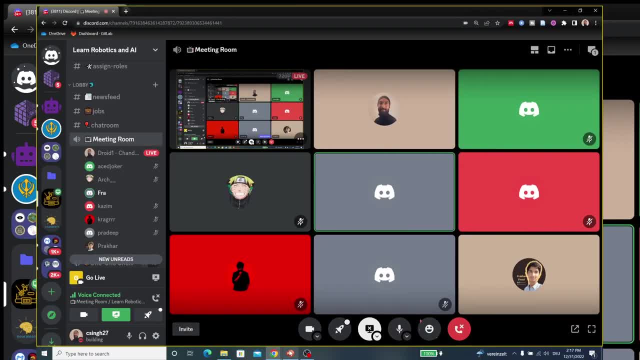 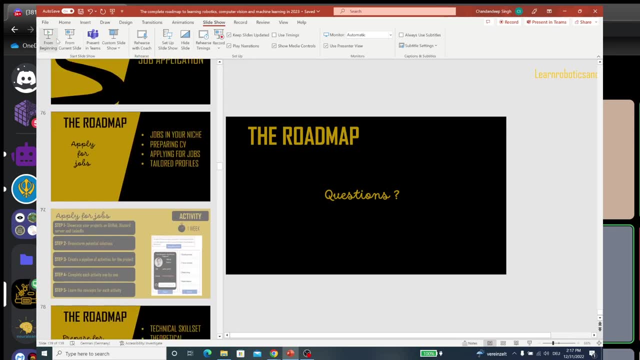 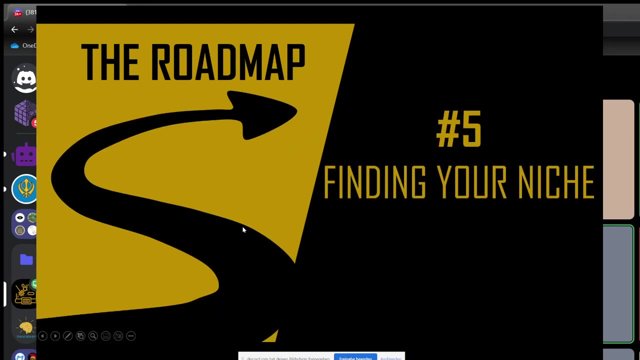 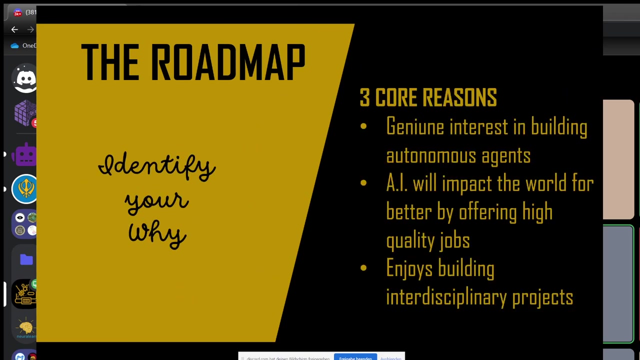 different kind of tools that um are expected of us to pretty much know of, and then, after choosing a particular sub-domain, we have to master it, particularly with Ross. I was just I just wanted um to know um pretty much, because I haven't um. I have a very big interest in mobile um robots. Ross is um properly um new to me and ours pretty. much and pretty much the internet. even though there's like a whole lot of resources, there's very different platforms and services. I think that can be useful. value of the future is how are they used and how do you preserve them out there. so thank you for taking my side. 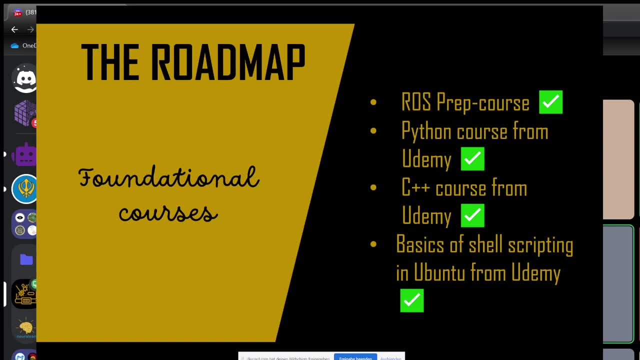 lot of resources, it's very difficult for me to actually like stick to find a particular thing that i can focus on solely. so this roadmap is good, but the tools, um. when you mention ross, i just want to know, um, is there a specific kind of ross that um we can be able to subscribe to, or is there like? 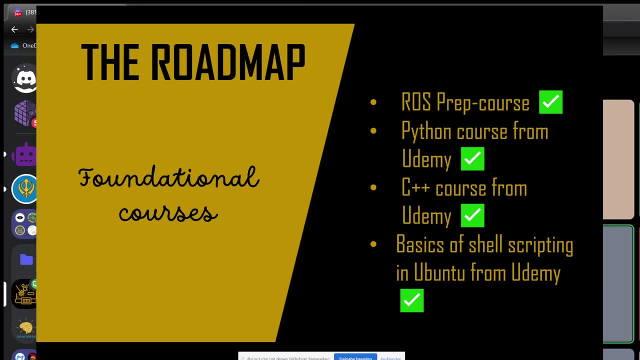 um different platforms that actually has um a, that actually has like um ross embedded into it, like web, like webots or um something along those lines. uh, yeah, so, uh, vbots is, i think, a different framework and ross is a different framework, so i would recommend that you focus on ross, uh, because, 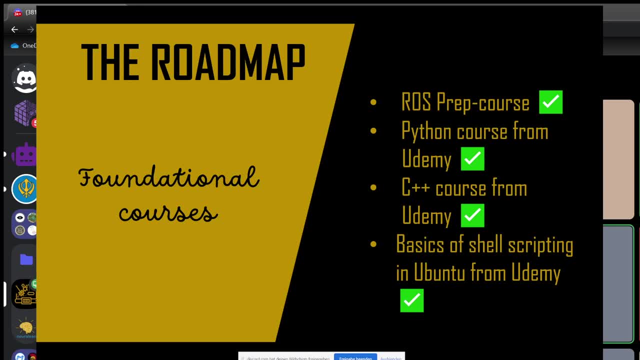 ross is more uh it's. it's more uh, sophisticated first of all, and then it's also more used, right, and ross is universal, almost universal now. uh, and for resources, i would say ross construct. i think maybe you've probably heard of it. so ross construct is a good uh resource and there are lots of free. 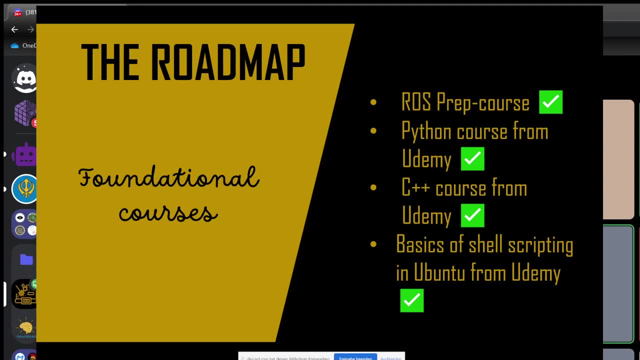 tutorials on youtube that you can find uh, and you could also refer to some uh books on ross pro. there's one uh called programming uh robots by ross, or something like that, or uh the um, or there's one uh that is more project-based learning. ross and ross, you should, of course, be learning in a. 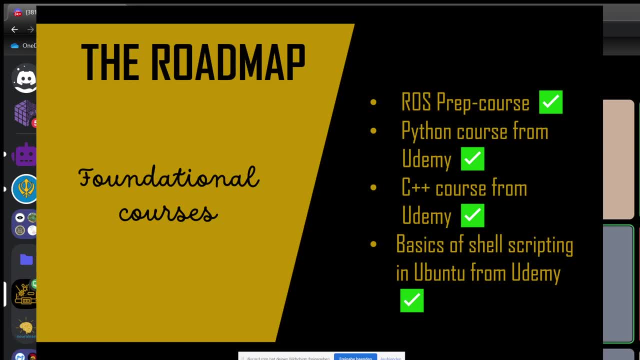 project-based way and that is by linton. linton, joseph, i think we also have uh in our discord server in one of the channels. i have to still see where it is, but in one of the channels it would be there. uh, but just search like linton. 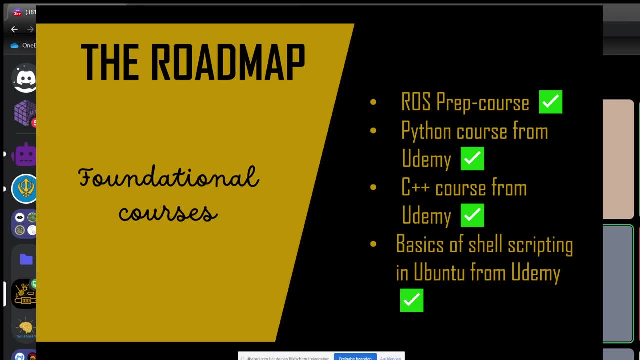 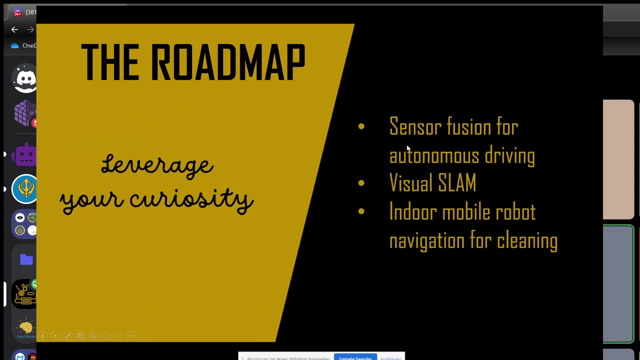 joseph ross project books. um, you'd be able to find, uh the pdf or purchase it, and uh, that would be a good way. and also, ross construct tutorials- actually, even ross construct tutorials would be good enough. uh, so the idea is that, uh, you want to do a little prep course just to get familiar with ross, but most of the ross that you 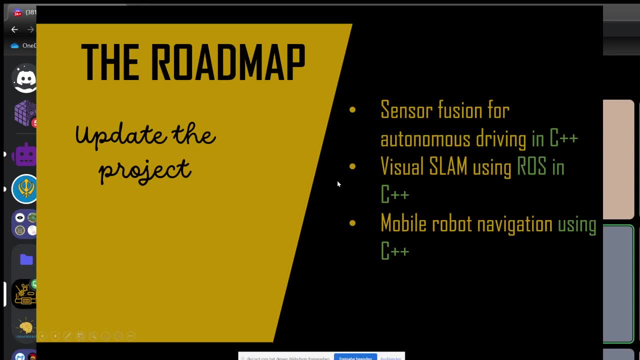 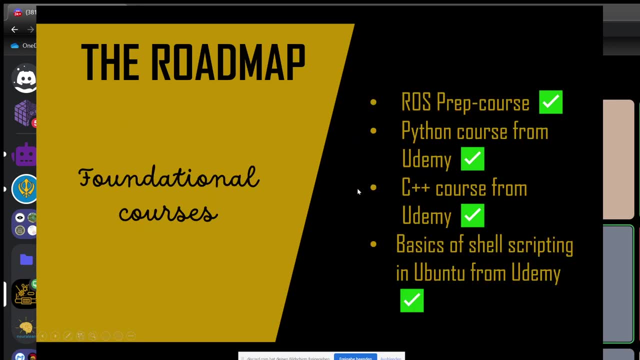 would be learning is, for example, if you take up this project, then you would be googling it and then you would be learning concepts along the way. so that is the idea. okay, perfect, thank you, um. and for my second question, um, back to the frameworks, particularly with subdomains. um, i want, i just 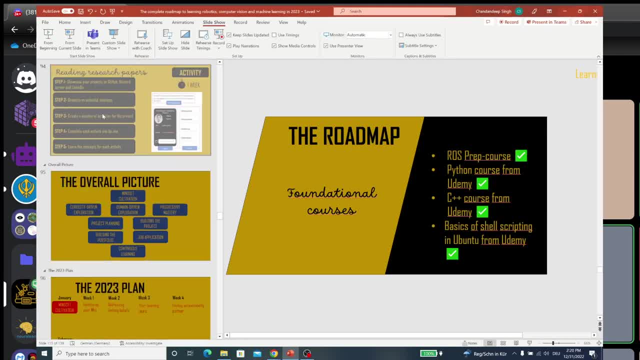 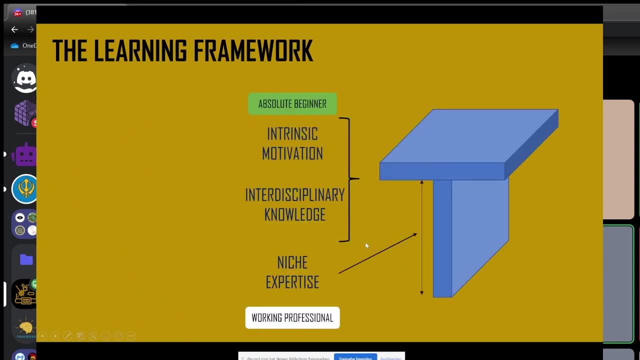 wanted to know um if there are other in within the subdomains um. i just wanted to know if there are other subdomains um, again um. let me take the example of my interest in mobile, um, robots, um, and i wanted to like um, go into like research, like finding, like pretty much trying to find exactly. 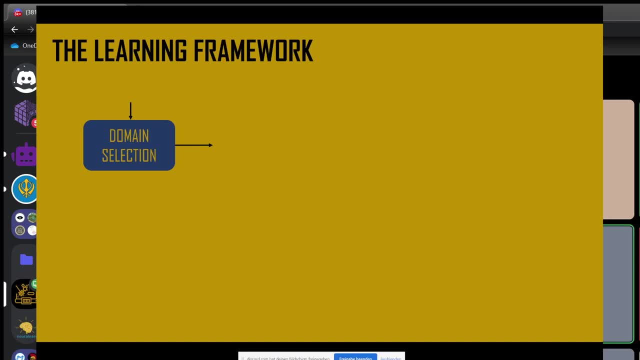 um. what can be the problem or the hypothesis of it? um in doing um that subdomain, um are they like any extra resources that i can be able to find um here on discord, like different blogs or um different websites that actually have real world or um real life use cases where i can? 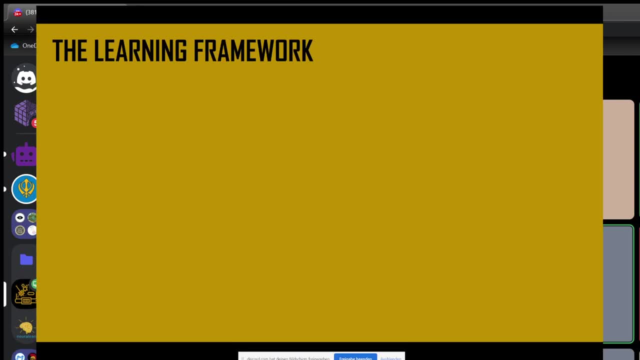 be able to study, learn and then actually find a problem within it that i can be able to research. so, you, you want to focus on research. so, uh, where are you based currently? and i want to know, uh, what is your background? are you studying, are you working right? um, i'm based in south africa. uh, i've 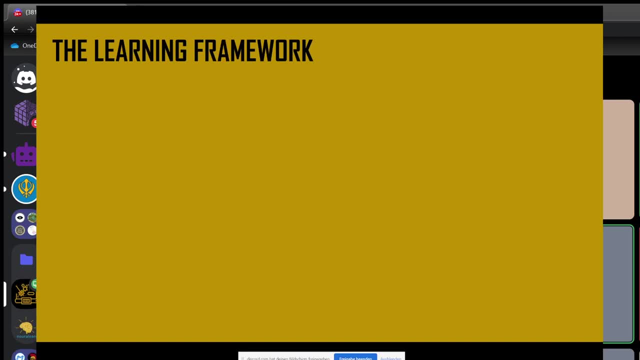 i pretty much. yeah, i can pretty much say that i pretty much. i'm finished with my honors degree in information and communications technology, um, particularly majoring in um data analytics and machine learning, as well as iot um architecture. okay, okay, okay. so you have a programming background and you want to. 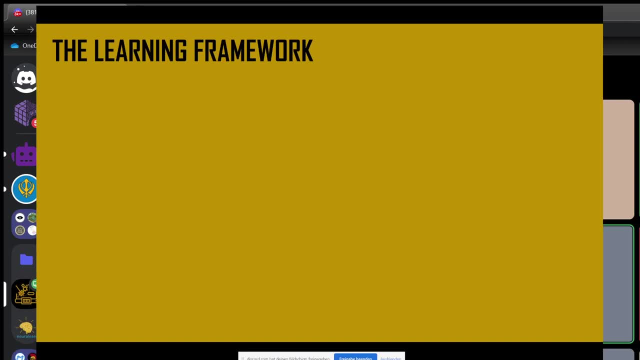 learn robotics and you want to specifically go in research? right, yeah, yeah, for mobile, for mobile robots, yeah, uh, okay, so for research, um, so do you want to go for a phd or do you want to do research on your own, just for your own interest? um, i definitely would like to take out. um, yeah, i'll definitely go for the. 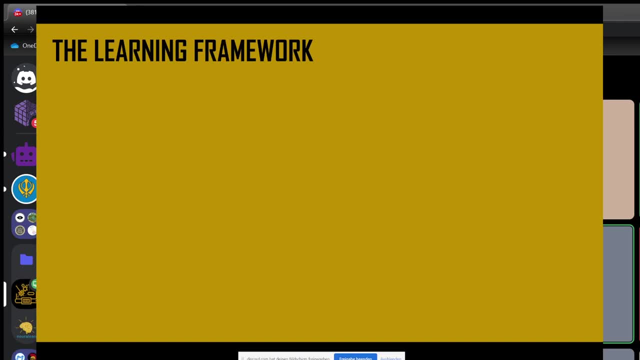 phd path. but what my? but my plan is um, because next year um my master's um classes are going to be offering up to me. i just wanted to take um the year just to really find a problem, to really solve that, and my interest is to do that. so i'm going to go for a phd and i'm going to do. 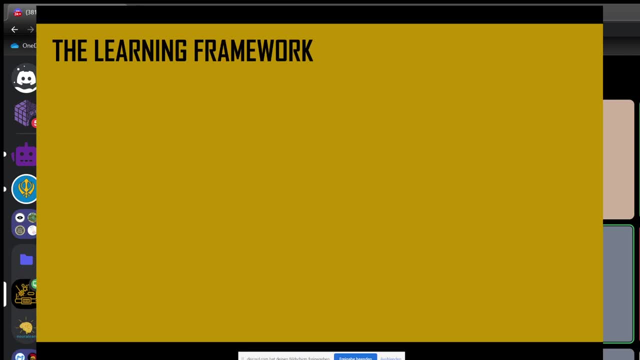 application for robotics and the. my interest in robotics is pretty much um a strong one. i don't want to focus too much on um iit for the most part and just focus on applying my programming skills in the robots. in robotics, though, um pretty much before i go for my master's and also reaching for 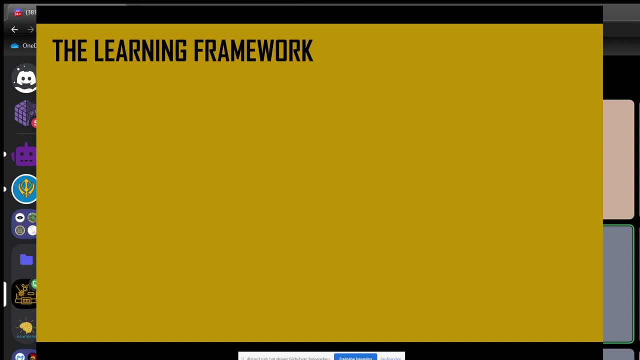 my phd um in iit and slash robotics. i just wanted to get immersed into it and also find a problem that i can be able to use as like a good research um for um, for my um, for my academic career. yeah, yeah, i guess that's the answer to that. i guess that's what i wanted to know about that, so i'm 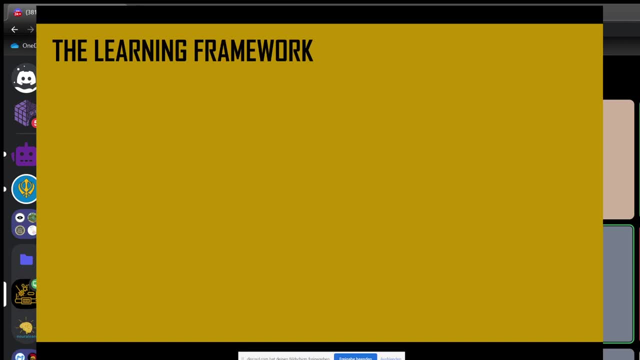 gonna ask you to provide us with some sort of that you're working on. so, um, what's your biggest problem? that's been the key to stay in the robotics realm. so, um, what's your biggest question for the? Yeah, so I think you can break it down into multiple stages as well. So the first stage, of course, would be to finding the right subtopic in mobile robots, right? I'm not involved much in research in the mobile robots domain. I'm more in the manipulation and reinforcement learning. with regards to research, 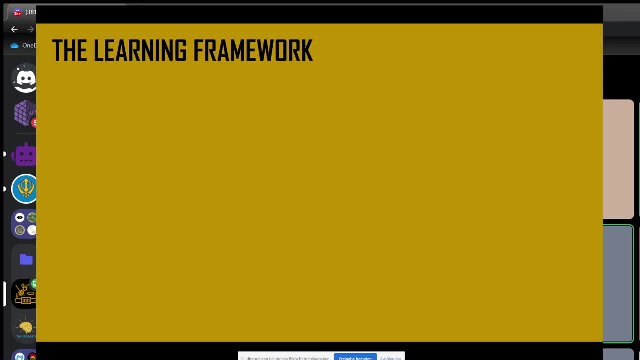 But for mobile robots? basically, the short answer is you have to skim through lots of research papers, collect ideas and see which ones you would be most interested in, and try to identify the gaps. And the way that you can do that is by seeing the last section of the research paper, where it talks about the limitations and possibilities of future work. right, 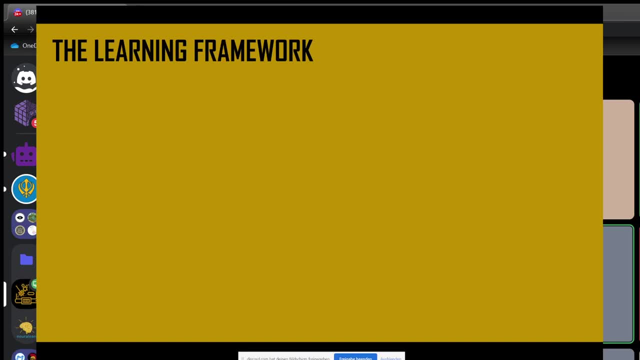 So once you do that, you'd be able to see: okay, these are open-ended problems with regards to making mobile robots autonomous, And these are the things that you can focus on. Also, you can attend conferences and so on, And you could get an overview of fields, like also watching lectures on YouTube. I think that would give you a good idea. 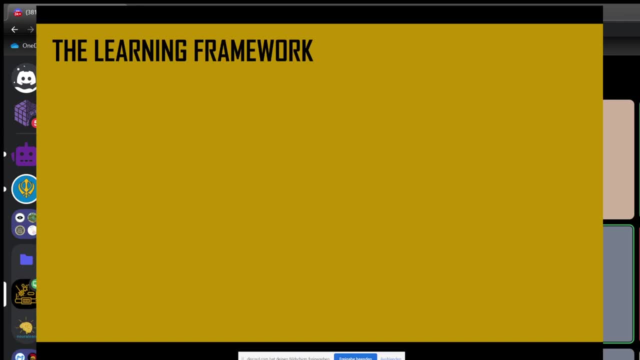 As to identify the gaps. So I think specifically, you can break it down into first. So the first step would not be to identify the gap. The first step would be to identify different areas in mobile robots, like different areas on which there is ongoing research. 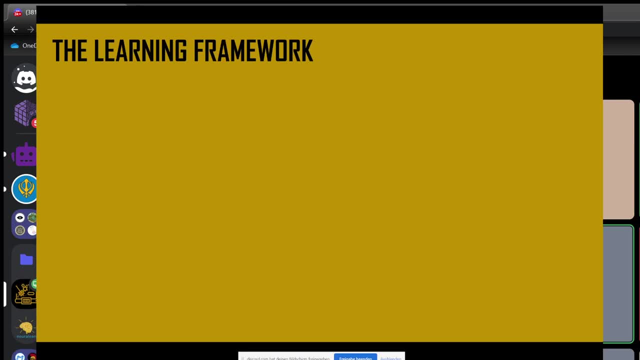 That would be the first step, And the way you do that is by reading the introduction, the abstract, and skimming through the paper just very briefly, maybe a day or two, And then collecting down the ideas, Make your own notes. And then, once you have your own notes from, let's say, 20, 30 research papers- as much as you can read- then you can identify that these are, let's say, five to 10 different areas on which there is active research. 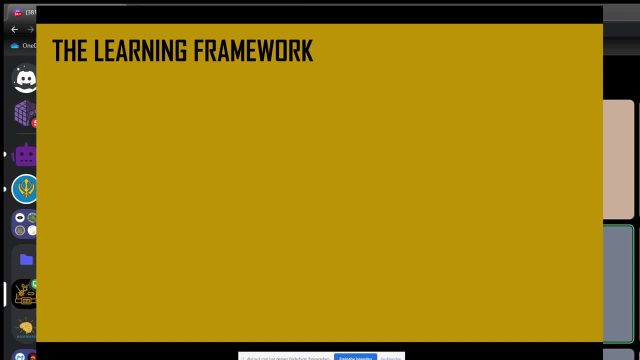 And then you would go on searching more And then you would see the limitations and gaps in this And then you would filter out and you can then decide: hey, this is a gap that I can, that I'm most Very much interested in, And then you would focus specifically on that. 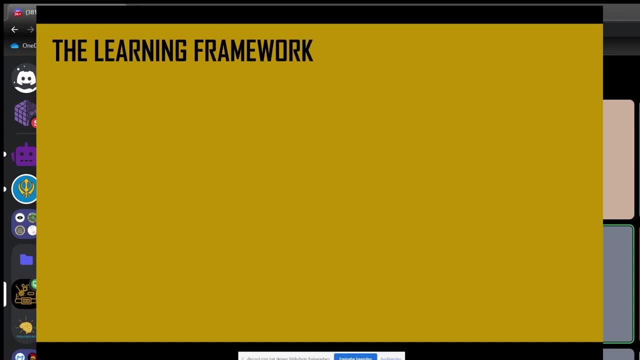 And that is also what one does in a PhD, But of course, this is easier said than done. This takes way more time. So, yeah, I think even identifying a research topic is a huge task in itself, So make sure you give enough time and don't pressurize yourself too much that I have to do it within a month or something. 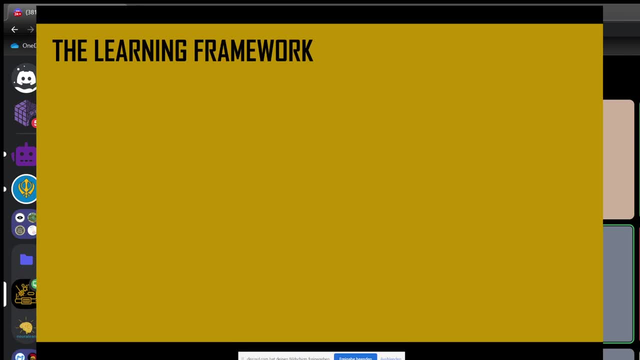 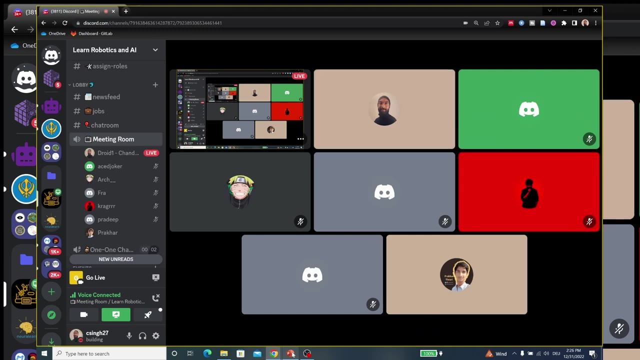 So it will be. It will be a longer process, but you'll definitely learn about it. Okay, Thank you very much. Yeah, No worries, And yeah, Any other specific questions related to the framework? I would like to know what exactly are the topics or? 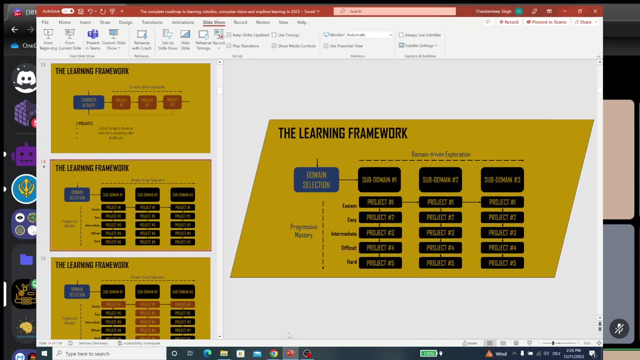 In, Like In Physics and mathematics, that one needs to know in order to have a better understanding of robotics as a field, Or maybe it may, Yeah, Yeah. So of course, in this presentation I've given just a very broad overall picture. 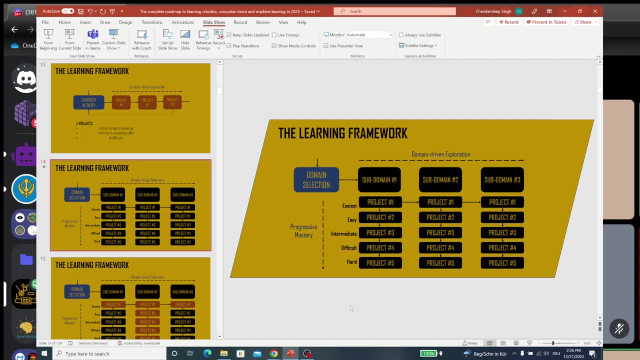 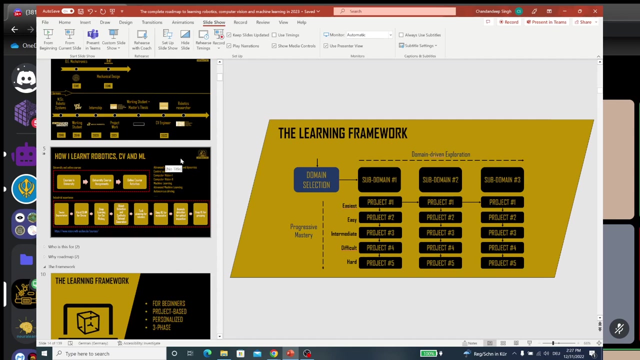 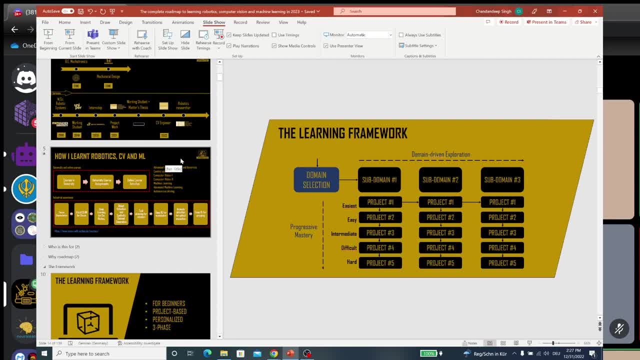 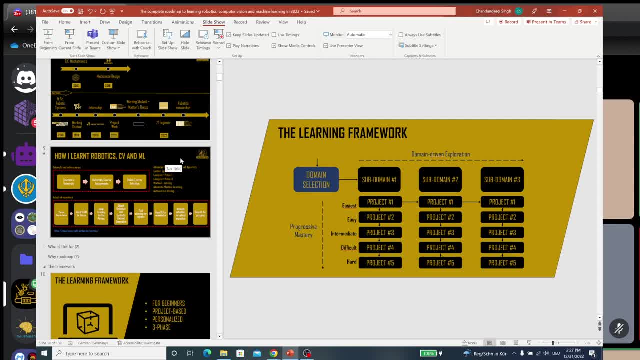 Yeah, Yeah, Yeah, Yeah, Yeah, Yeah, And so on. and then you take up a project in computer vision and then you see that this is how this is being used to solve this particular problem, and so on. So, yeah, just focus on the basics. if your basics are clear, don't spend too much time. 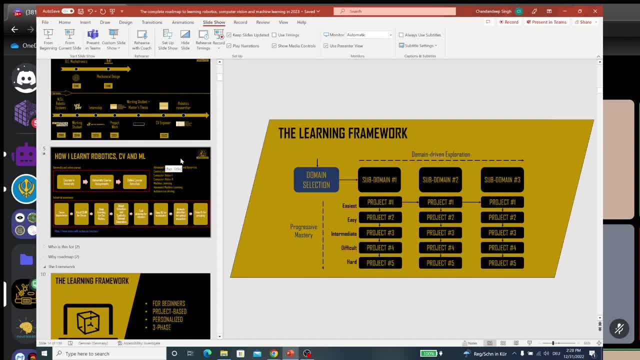 on mathematics or physics. of course, for robotic manipulation, mobile robots also, physics would be important, but just general laws of physics from your like 12th and so on. I think if you have that, the rest physics you can grasp along the way and of course, you would need the physics. 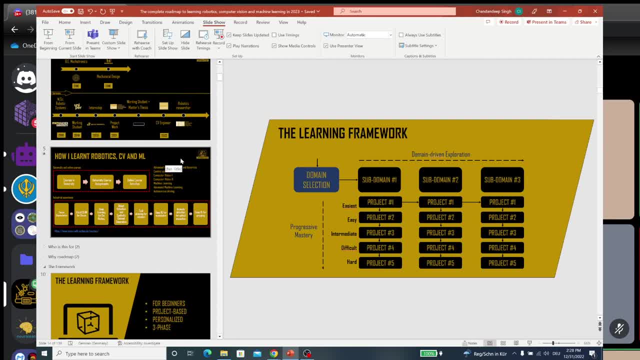 as well. but the idea again is that you would learn the physics of the theta angle that would be required for the movement of the mobile robots, or the trajectory planning and stuff like that that you would learn along the way. so don't stress too much on the fundamentals, just make sure. 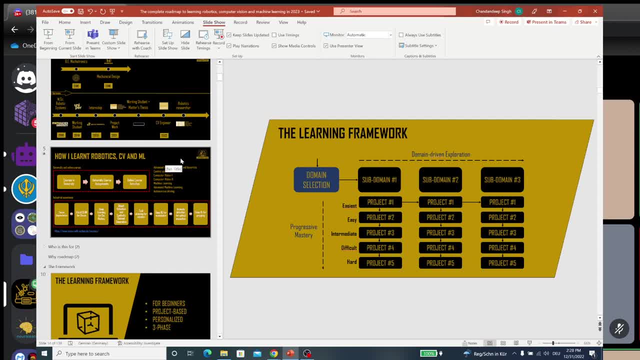 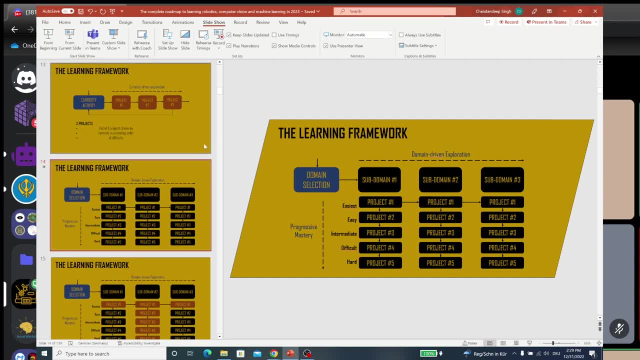 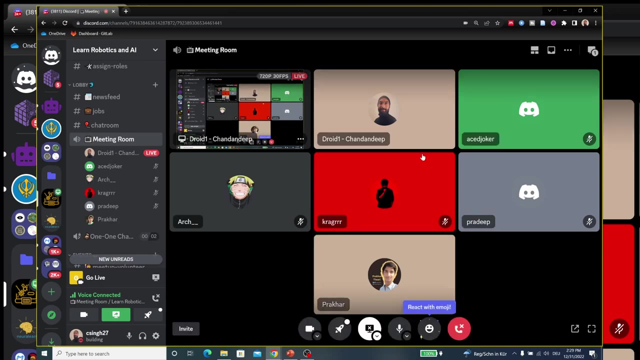 that it's. it's not to the level that you don't understand the basic terminology. yeah, got it, thank you. yeah, maybe I'll also make some this a video on the fundamental topics in more detail, some point. yeah, that would be helpful, okay, so so so far, I think East East Joker, I think you're new here. 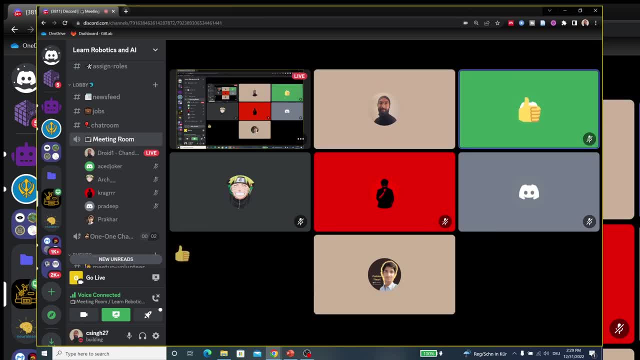 right, yeah, so could you share your feedback or maybe a little bit about yourself and what your background is and what your goals are? basically, yes, hello. so currently I'm a student. I'm studying in a bachelor degree in mechatronics in Malaysia, so my goal is actually: well, for now, it's just to be able to understand the how the robotics. 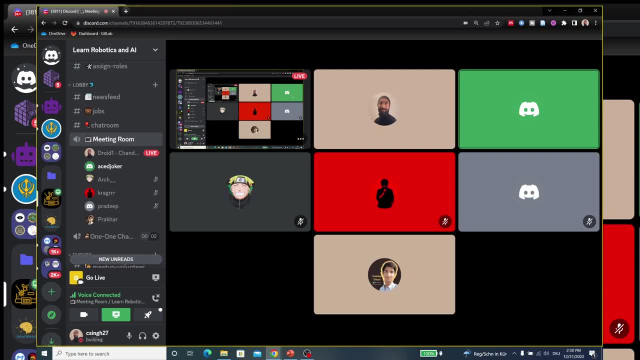 works. so I'm going to start with the robotics. so I'm going to start with the robotics, so I'm going to go ahead and try it and, having a strong foundation on the robot, this robotics and like taste, like raw section- I still don't really have much understanding about it yet. yeah, that's all I guess. okay, cool, cool, cool. yeah, sounds sounds good. and what do you think about the framework? do you think this would help? 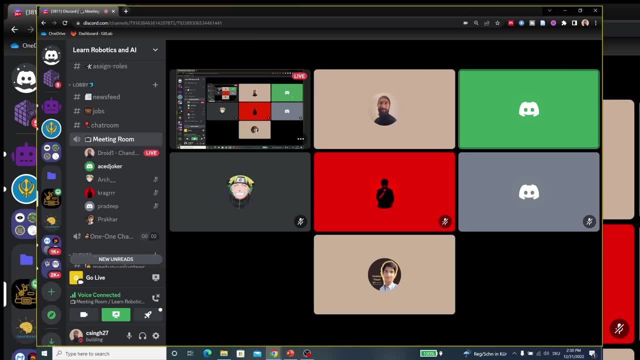 you systematize and plan towards your goals, or yeah, cool, cool, cool. yeah, sounds, sounds good. and what do you think about the framework? do you think this would help you systematize and plan towards your goals, or me sort of also? yeah, for me particularly, it is quite okay for now, since i really don't really have a roadmap. 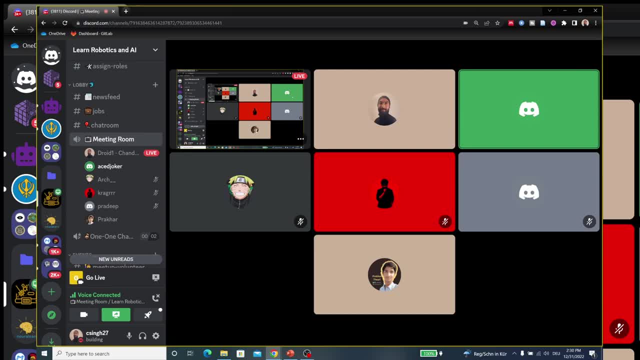 to study on before, like today, i would say so. yeah, i think i could use this as a reference. okay, okay, sounds good. yeah, thanks for sharing. and then, uh, krish, let's hear from you. yeah, so, honestly, i was a bit uh busy side by side writing my paper, as the deadline is today. 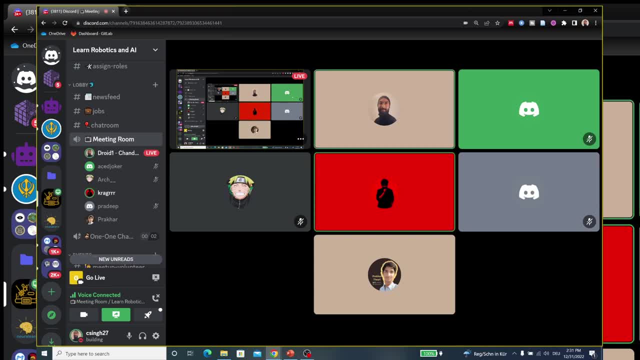 okay, okay, okay, no problem, no problem. new year, okay, you keep working till the end, very last moment. it's not like that, but like i was seeing some slides and i was hearing also, like i think the timeline- oh, sorry, not the timeline- i think the proposed framework. 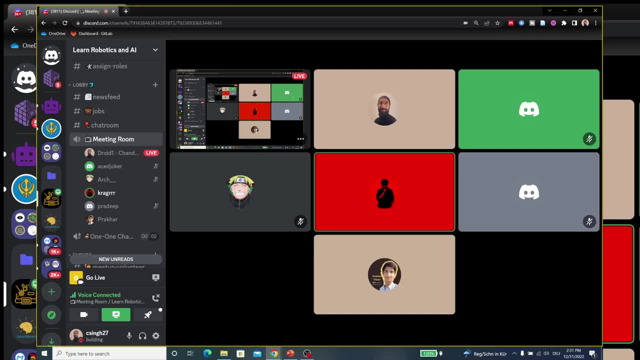 is like really well put up and i think, if, if we can get some guys like us, like minded, like who are, who are, who are present year, and maybe board uh, to work on this, I think, yeah, it will be good for the community also to uh, you know, brush up their skills and 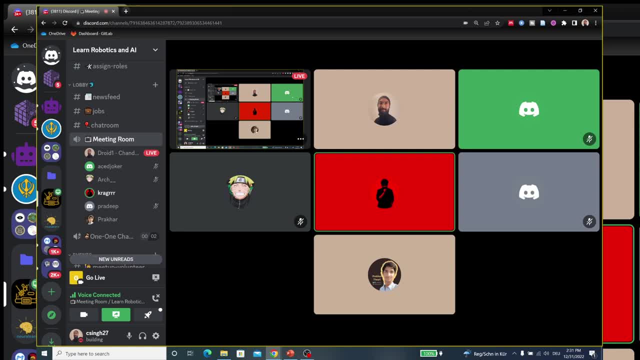 then learn also and then apply their skills and then, uh, write in their portfolios or their LinkedIn profiles: Yeah, Yeah, Okay, Yeah, Thanks for sharing, Krish. Um, so the last one would be arch. I'm just going to underscore: um, we cannot hear you. 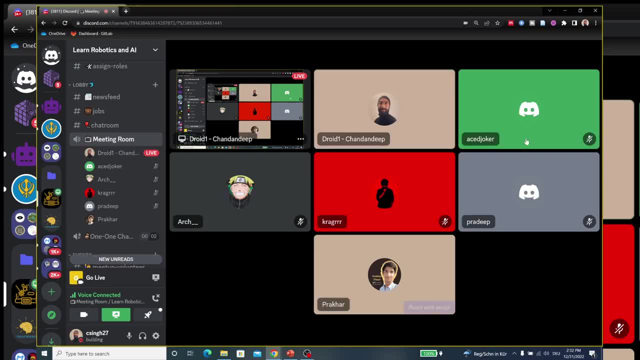 No, I think he has some issue with his microphone. Okay, Um, yeah, I think we can um wrap up with today's session. Uh, I hope it was not too long and boring. I think it was too long actually, to be honest. 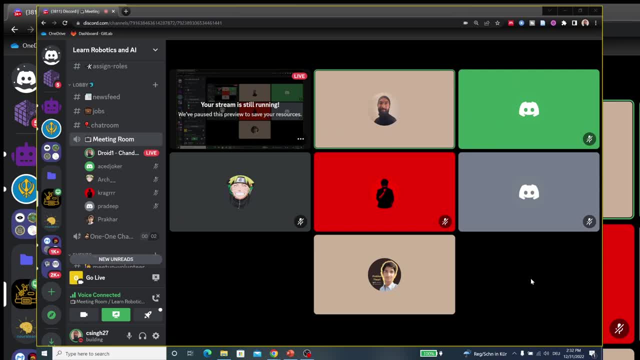 Uh, but uh, I hope it, you, you were able to get at least something from this And, uh, if you have any questions at any point, or if you have some ideas or suggestions, also just reach out to me. on discord itself: uh, and that would be cool. 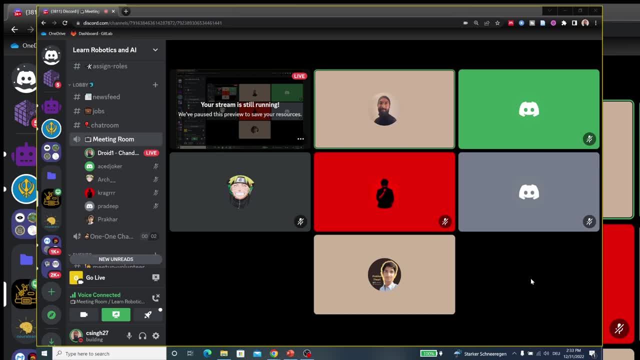 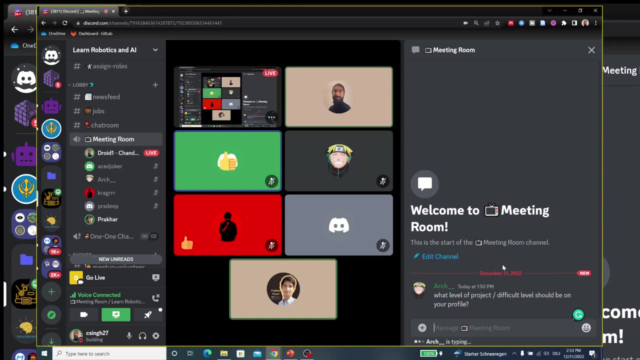 And uh, Uh, if everything is clear, then I wish you all a very happy new year and a good time ahead. Arch is writing something. Thank you, Uh. what level of project or difficulty level should be on your profile? Okay, 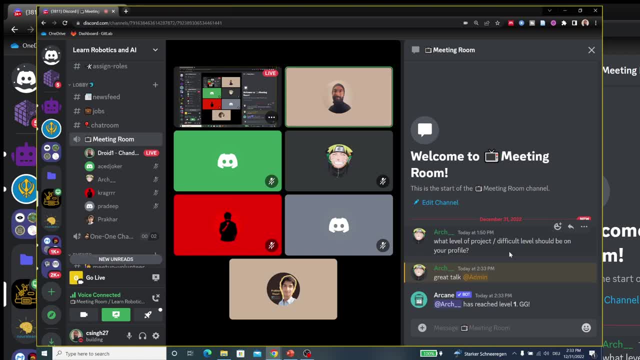 Um, what do you mean? This is a. Could you expand on it a bit? By the way, I wanted to know if we can make a GitHub repo or something, or a little website where we can lay out a whole roadmap of robotics for the people who are just. 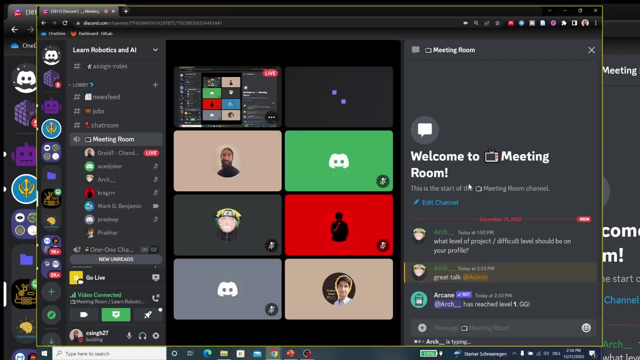 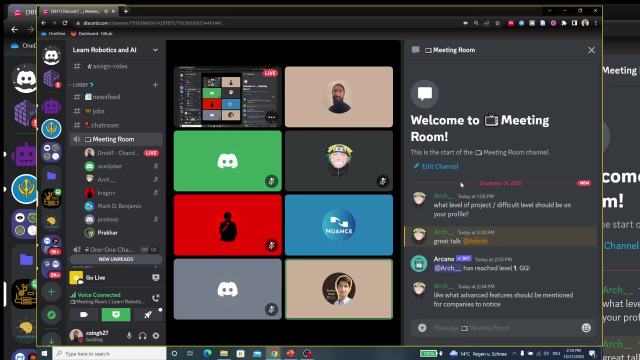 curious to know, or Mm-hmm, Yeah, Uh like. if you know, there's a website called uh like. the URL is roadmapsh, which contains literally the roadmaps of uh like front-end development, back-end development and stuff. 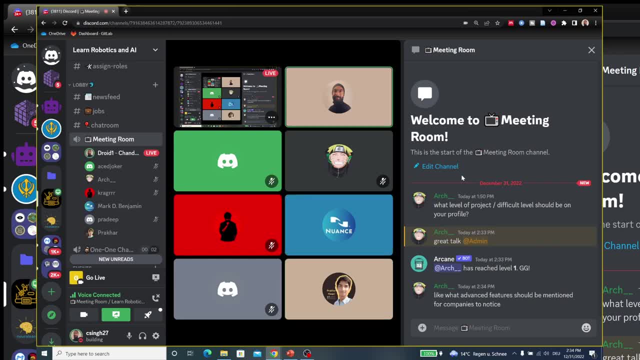 like that There's also for- yeah, yeah, There's also uh for computer vision. I've found those uh roadmaps on GitHub and I think some of them are pretty good Uh, but the idea is, uh, they are mostly like you watch this lecture and then do this little. 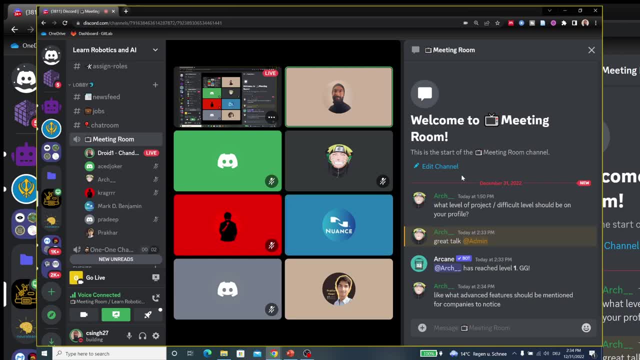 activity and so on, Uh, so. So that is a bit different from this approach, but of course, there are some good uh, actually the one by uh Syraj Raul. I think he made some good um, GitHub, uh, repository, uh. 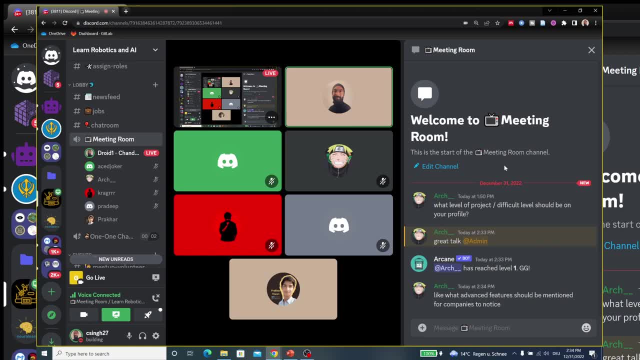 the roadmap thing. uh, that was also like take up the lecture and then do this assignment and so on, But I think that is also something that you could uh refer, and at least for project ideas. So, Yeah, Uh, maybe you can check out, uh, Syraj Raul's resources. 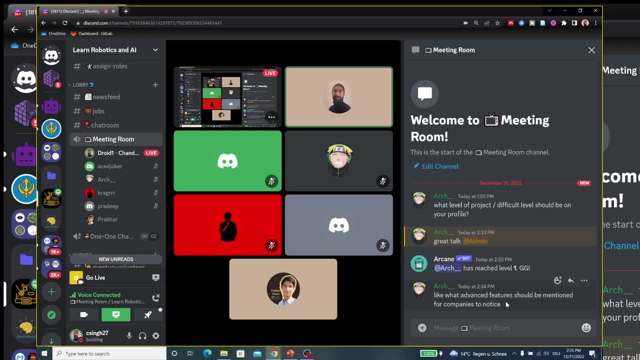 Yeah, Yeah, Yeah. If I find some other resources, I'll share it on discord. So, yeah, Thanks for I need to go for now. Thank you for audio. Yeah, Thank you, Thank you. Please share that PDF format. 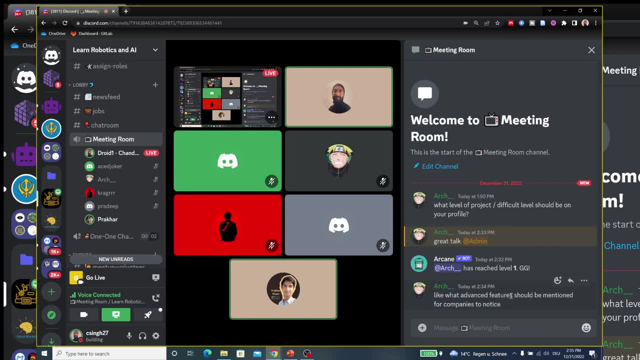 Yeah, sure, Sure, I'll share the PDF and uh, uh, I'll uh add it in the announcements. Okay, Thank you. Take care, everyone, Take care. Happy new year. Bye, So let's see. 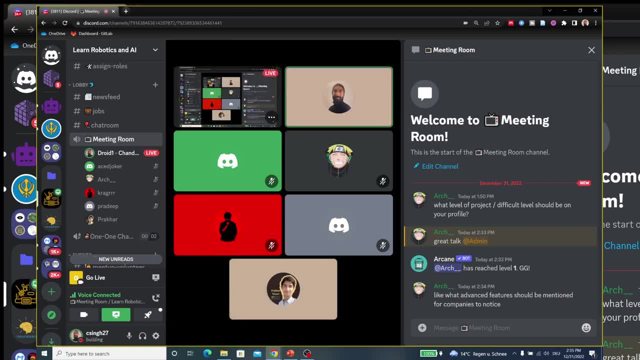 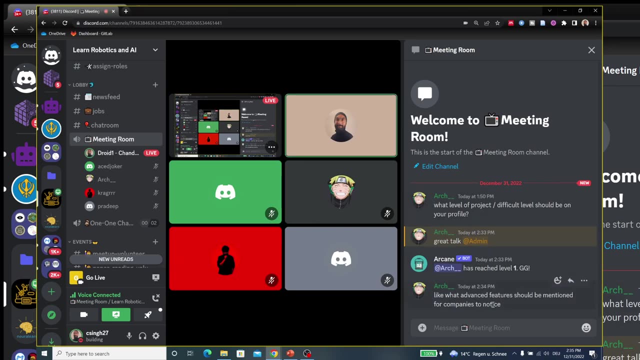 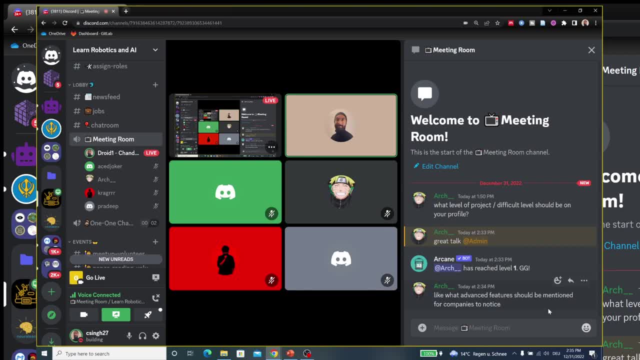 Finally, you are uh, uh, Wow, Wow, What a day. Thank you, Thank you. So I'm gonna uh around the generator. That was like a Yeah, yeah, Yeah, yeah, That was pretty cool, Evan was till uh. 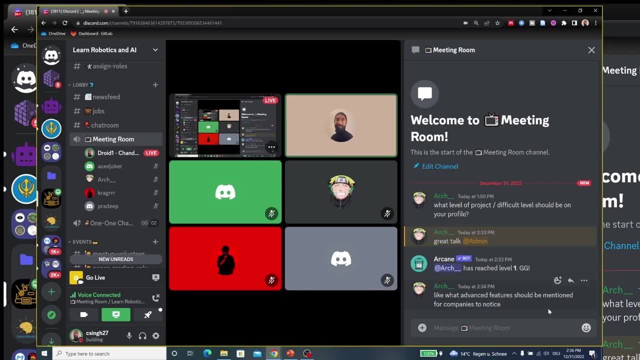 some company. maybe they require python skills and mainly python, and the idea is that your, if your project is the projects on your portfolio are very similar to the projects that are going on in the companies of your interest, then that increases the likelihood of getting a job there very much and even if there are no job openings, you could do a voluntary application. 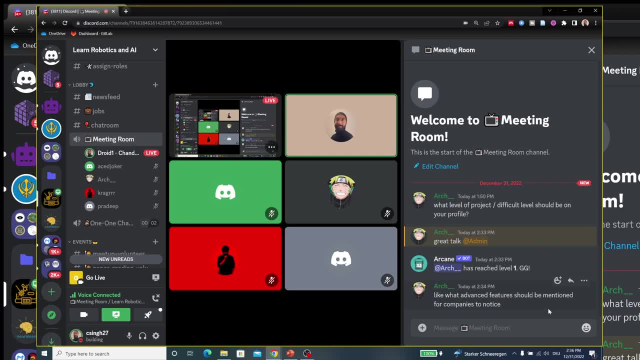 and because your profile is so much in alignment, they would a lot of companies consider that as well. so, in short, it depends on uh. it depends on uh. the company and the project need not be very advanced. so, addressing the first part of it, what level of project or difficulty level? it need not. 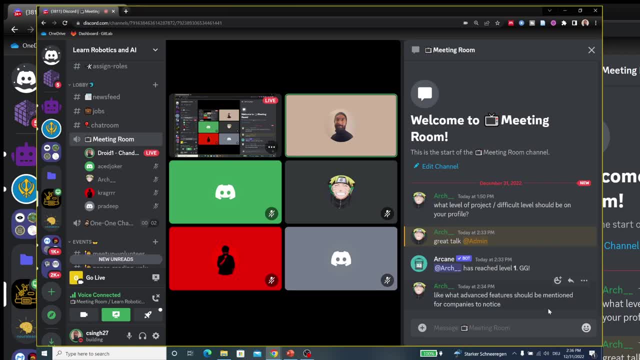 be that difficult, but it, if it is aligned and you're using the same tools, i think that's already a good demonstration, because you are showing you're learning on your own right, uh, and if you can get an internship in a similar kind of project to gain some experience, that is also a possibility. so yeah, i think that would be my take on this. 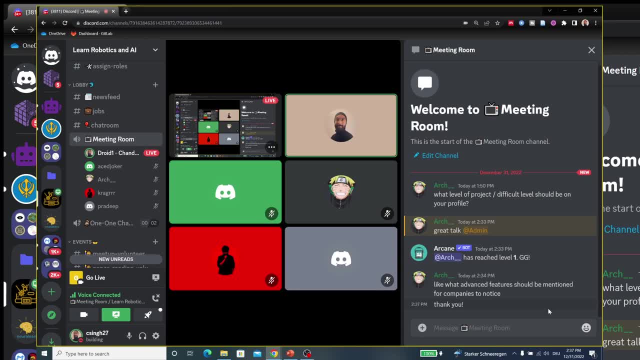 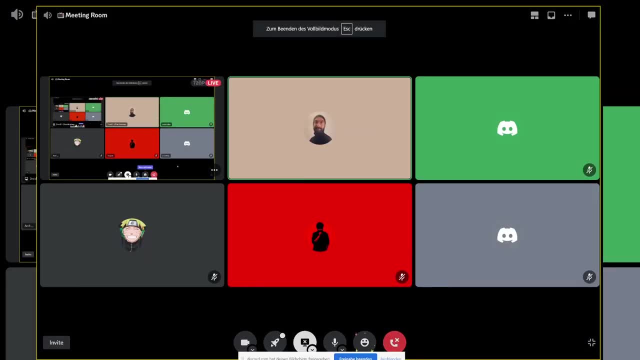 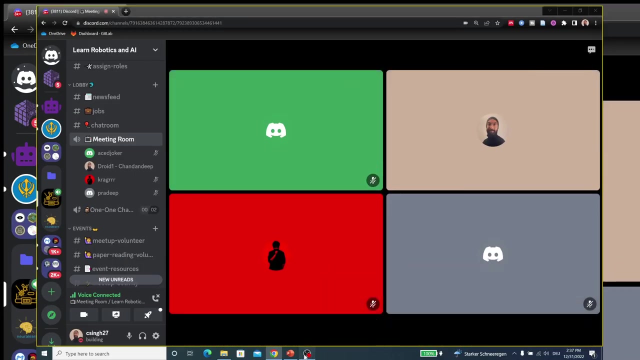 all right, yeah, thank you. thank you everyone for joining. uh was a nice discussion with you. thank you for the questions and wish you all a very happy new year and have a nice time ahead, and make sure you reach out to me if you follow the roadmap and you if you are stuck in any phase of this. all right, bye.